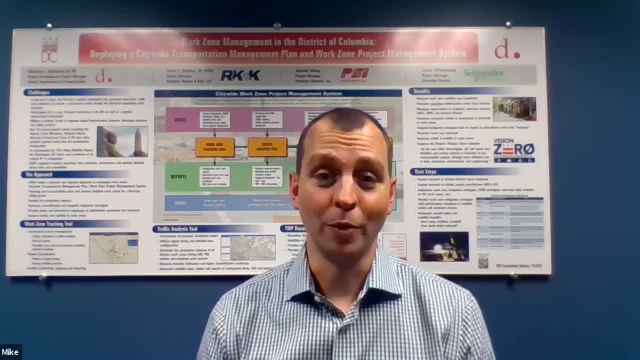 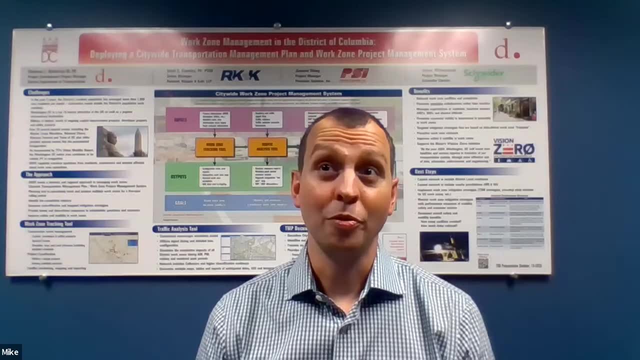 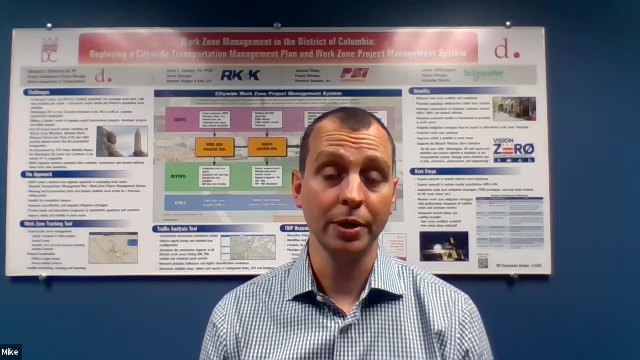 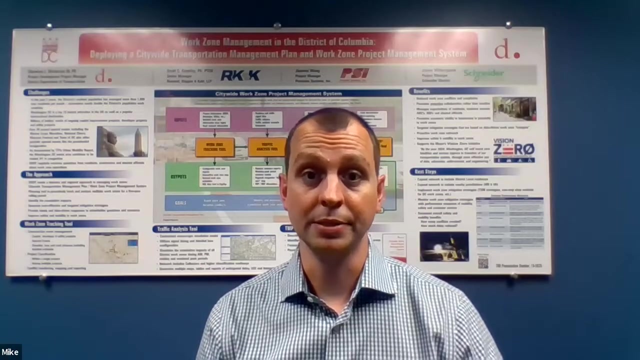 anything within the right-of-way the government property from along the roadways. Besides that, there are other types of transportation engineers, such as traffic engineering is another one of the big ones There. they look at everything from planning future roadways policies. they'll do modeling on what? 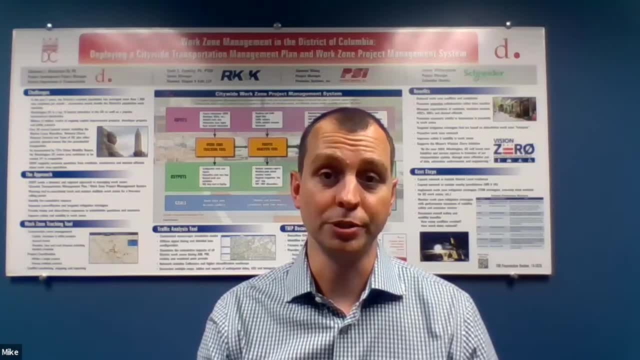 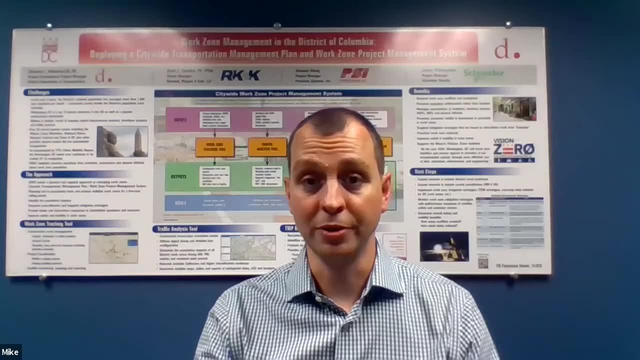 current conditions look like, what potential future conditions look like. they'll take different concepts and really see how that'll affect traffic and pedestrian and bicycle use in the present and in the future if they're implemented. and then you also have transportation engineering, which is another one of the big ones. 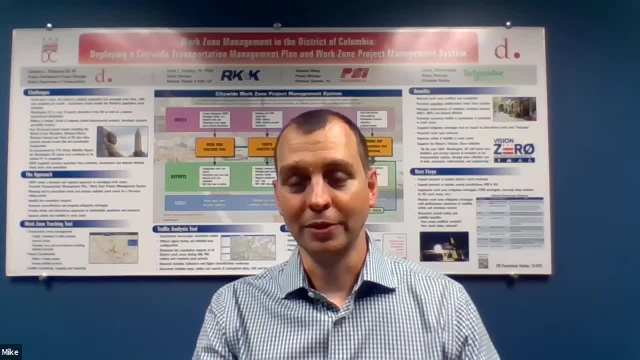 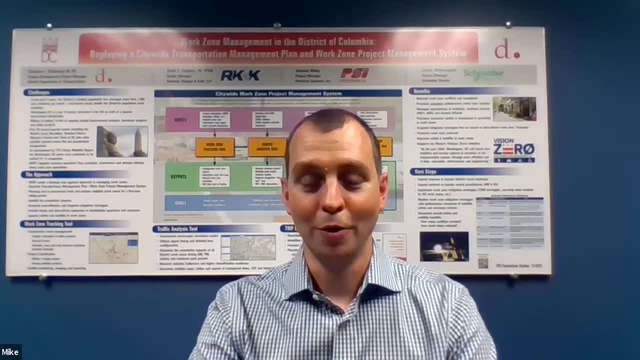 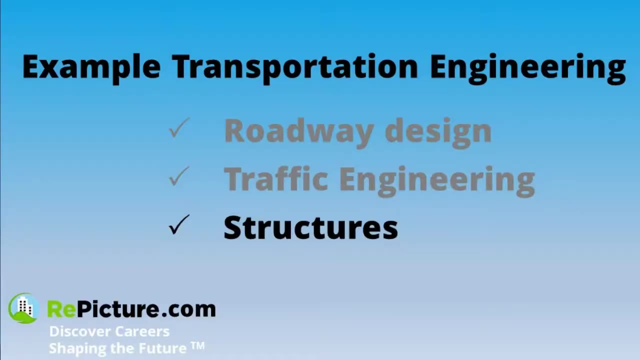 The traffic engineering design side, which includes doing things such as signal designs, lighting, really kind of more of the operations in the day-to-day of how the infrastructure is really put in. And then of course you also have structural engineering, so you will have bridges. 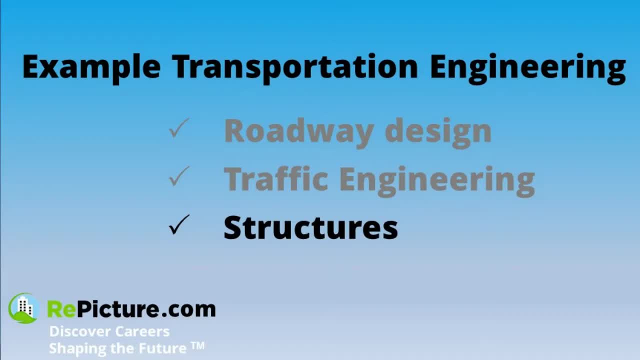 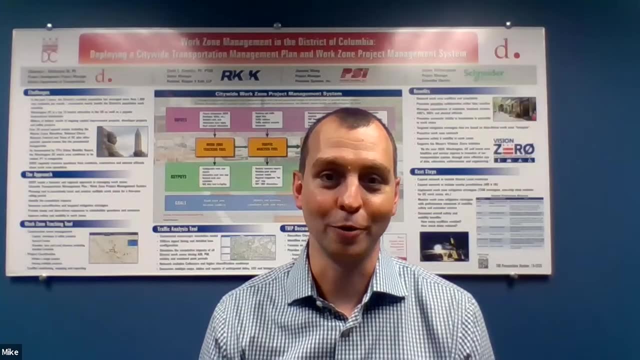 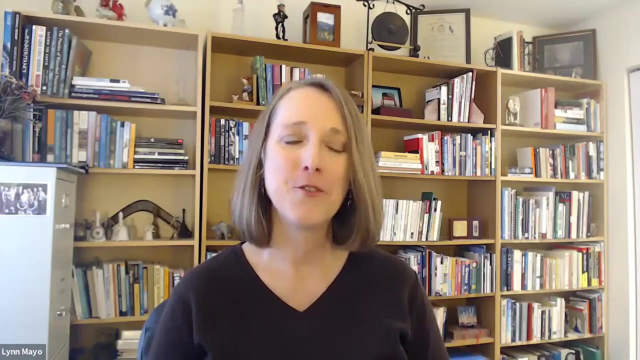 and culverts to get streams across streets, so it really touches on within those. just a few of those are some very broad categories of the transportation engineering. That's great and, like you said, it's just amazing how many different things are covered in there. 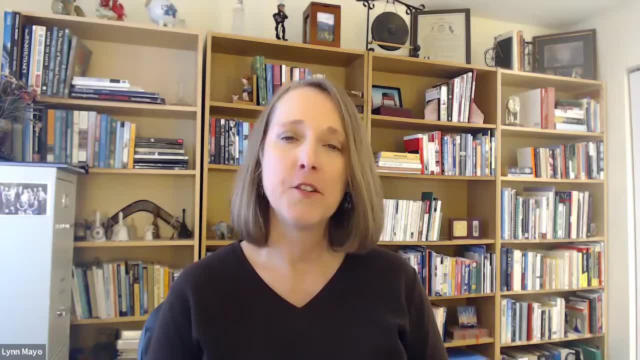 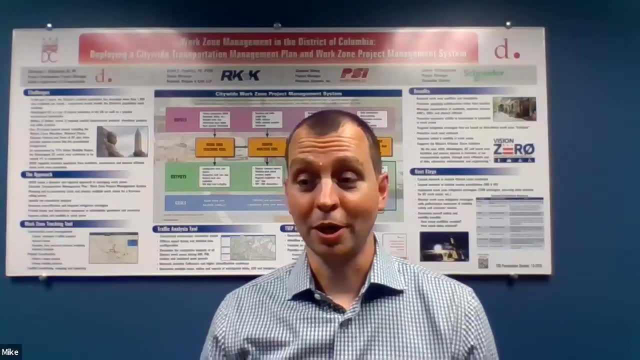 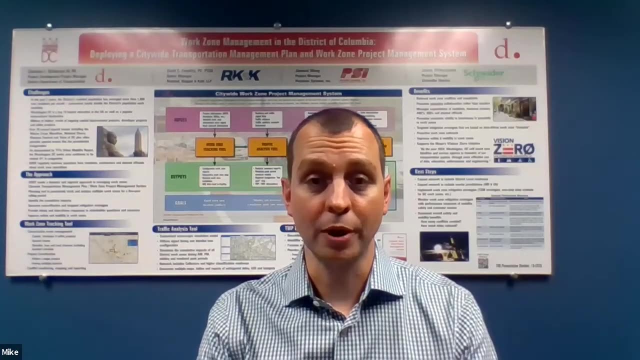 So like what kind of projects? and we talked about roadway design, but like what kind of projects do transportation engineers work on? So most of my projects, they're actually a pretty large range. Right now I'm working on two projects within DC that are actually looking at redesigning corridors. 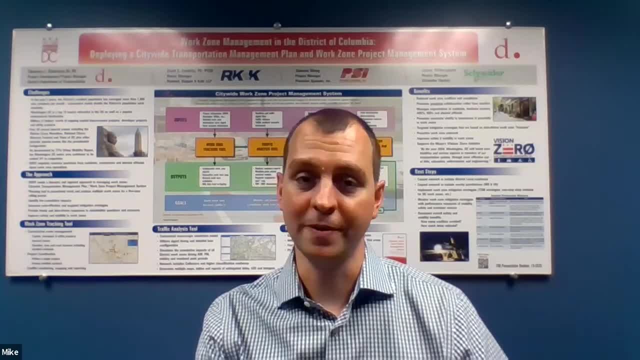 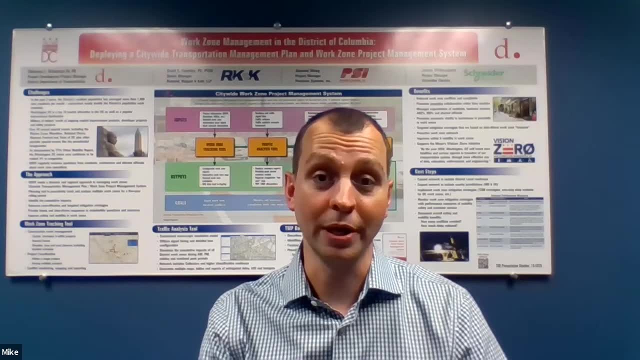 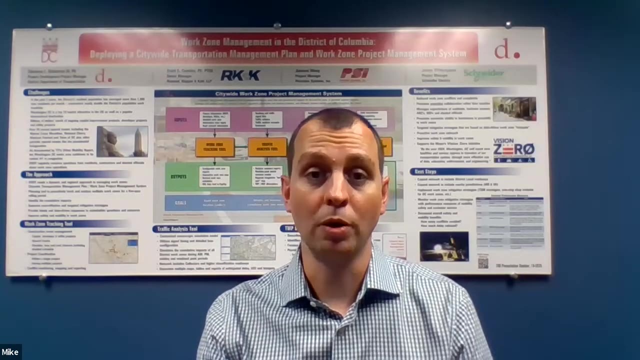 One is on Connecticut Avenue, just north of DuPont Circle, so it's a very heavily traveled road, one of the busiest in the DC area, and we're looking at changing the roadway configuration to provide better pedestrian and bike access, while continuing to provide the travel lanes for 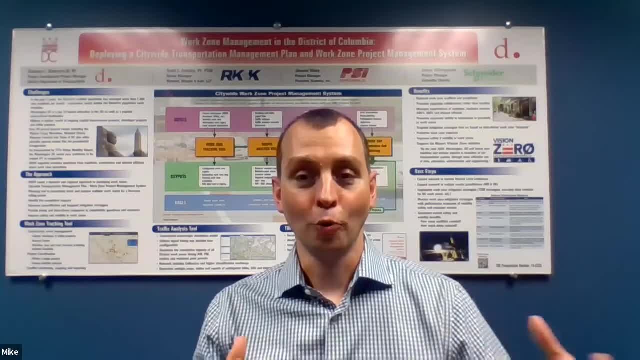 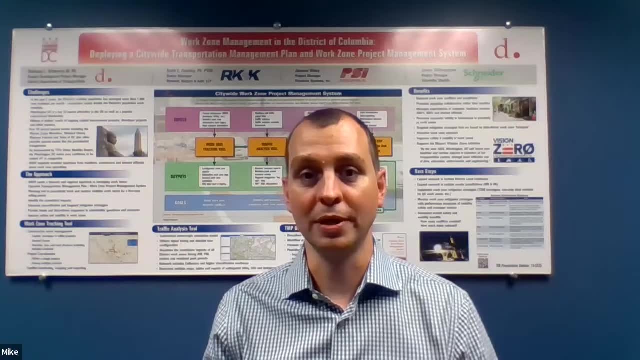 vehicles. So it's really just looking at going through redeveloping the area, including, like I mentioned, new streetscape and all of that, to kind of beautify the area, And then another project that area a little bit, but also then keeping our operations for all users. So there's. 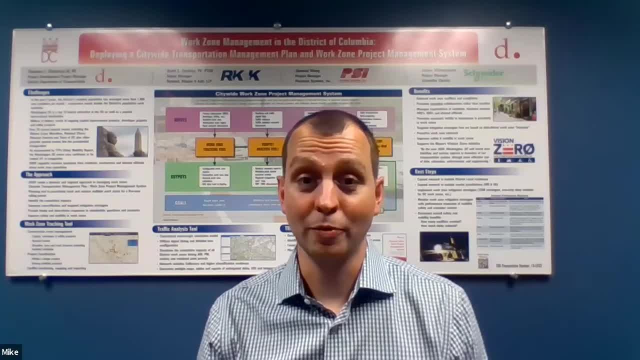 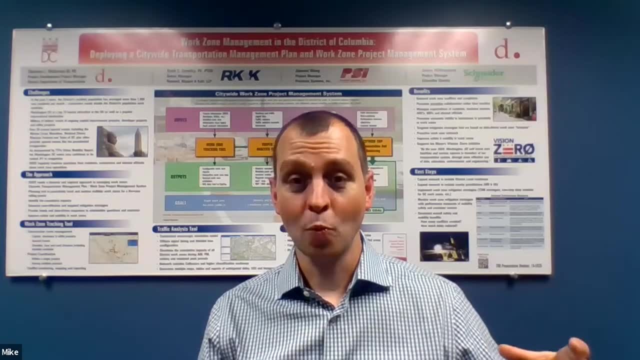 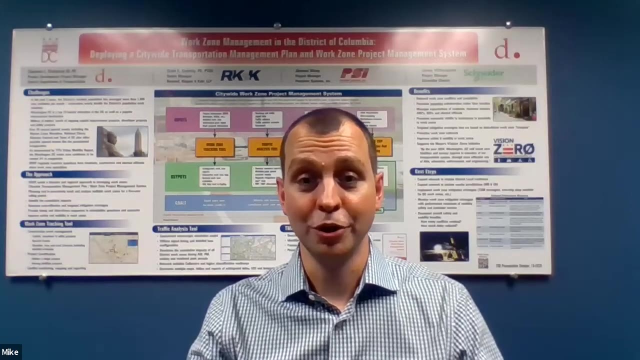 you can have projects like that. Another project that I'm working on right now is the is out in Route 66, so west of DC, where we're looking at the I-66 and Nutley interchange. So here it is a massive interstate interchange where we're doing. a completely new reconfiguration of the interchange as part of an even larger project that's redoing. I think it's well. I think it's like 20 miles of I-66 to add in toll lanes. So you have some of the Connecticut avenues which are a 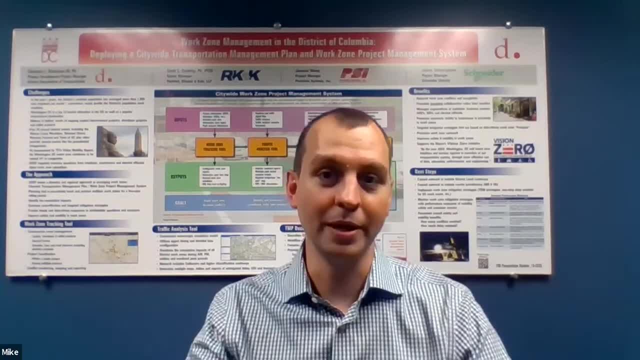 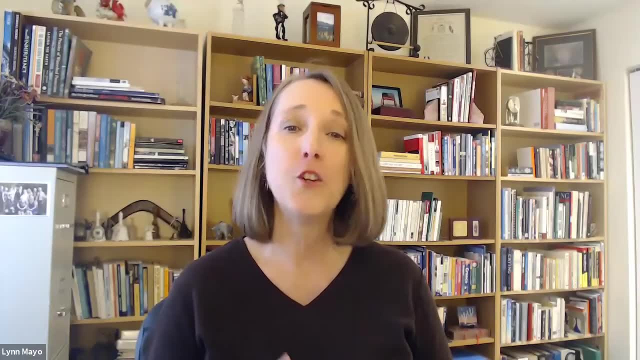 little more local projects and then you have some of these more big interstate projects where you're really dealing with large highways. That's interesting and I love the fact that there's local ones, that you're looking at the bicyclist and the pedestrians and things like that, so it's not just cars, you know, involved in. 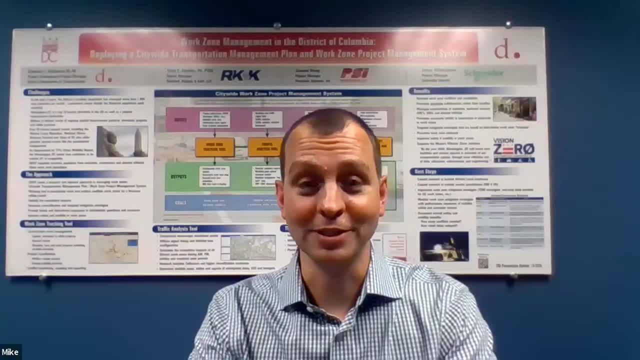 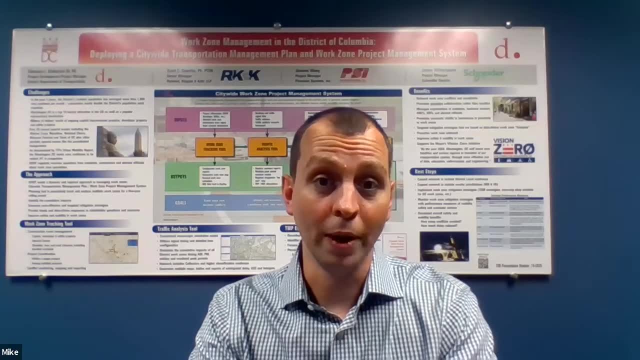 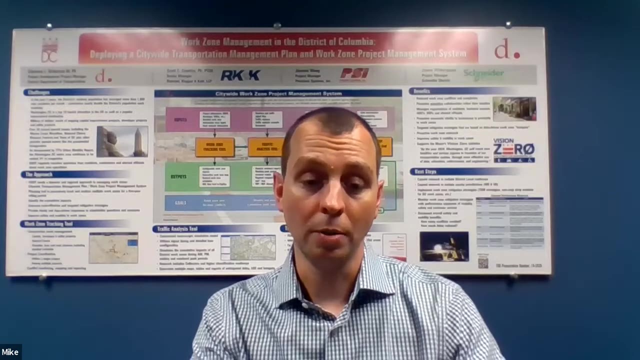 transportation engineering. Yeah, And actually a couple of the other projects that I've been involved in in the area have actually just had a sole focus on bicycle and pedestrian improvements, where the municipality I was working with had funding just for those, so we would be looking at creating. one of them was out in Silver Spring it. 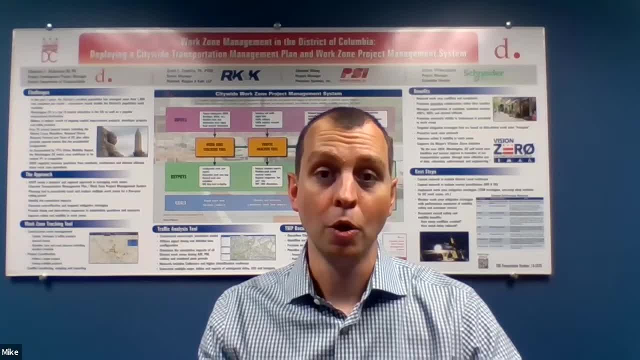 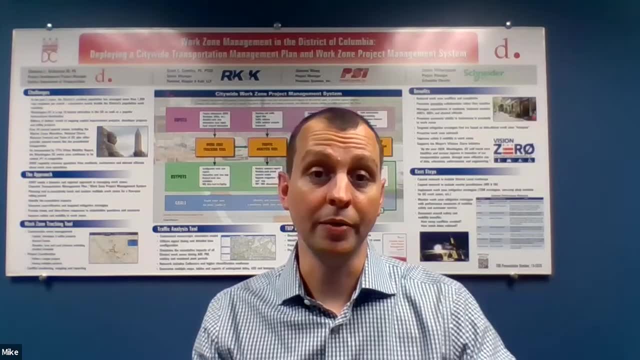 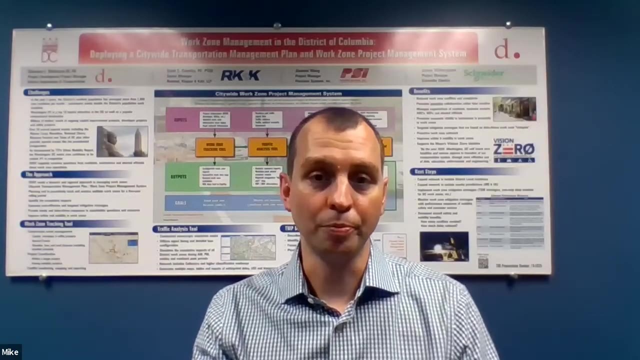 was creating a whole bike and pedestrian priority area where we'd be looking to make sure that there were bike connections throughout to get people on bikes to wherever they needed, and then also to include a lot of intersection safety improvements for pedestrians to increase safety for pedestrians crossing the roads and make sure that they had those connections as 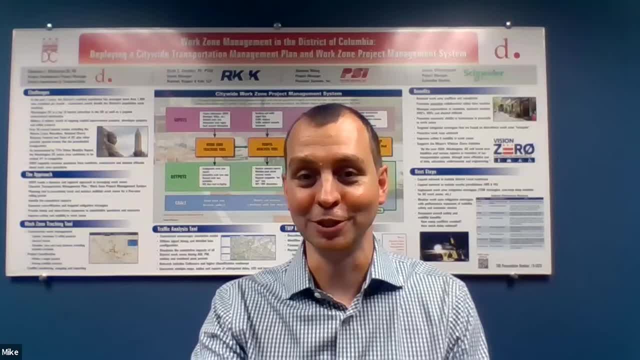 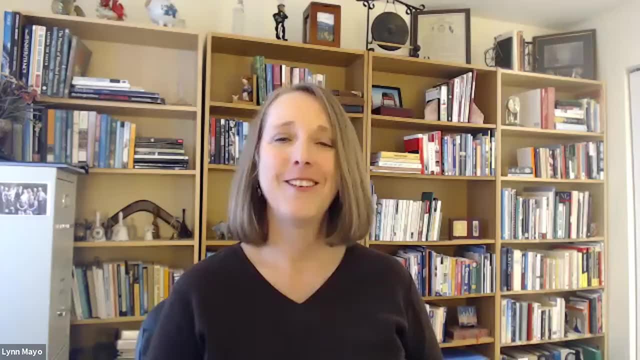 well, so that you were walking along a sidewalk, it didn't all of a sudden just end. You had somewhere where you were. you could connect to wherever you were getting or going. That's great. And so with the transportation projects such as that, there probably a lot of different people involved. What? 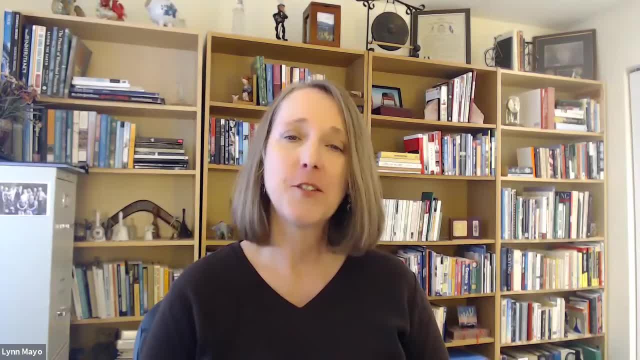 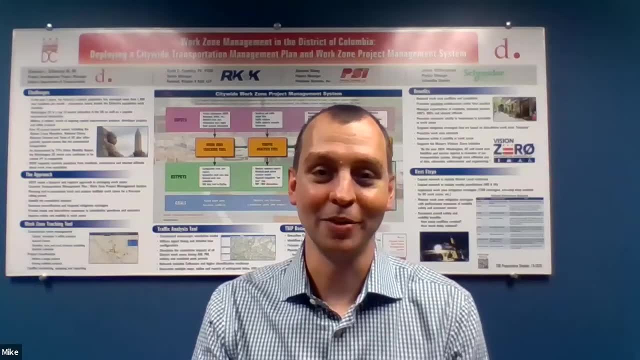 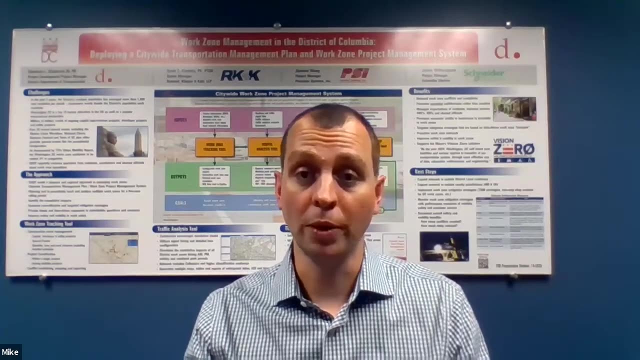 what did transportation engineers do on those projects? Yeah, Great question. Um, so it really just depends on the project and where it is in the lifecycle Towards the beginning of the project. I know on the roadway design side what we do a lot of is looking at the corridor and laying out. 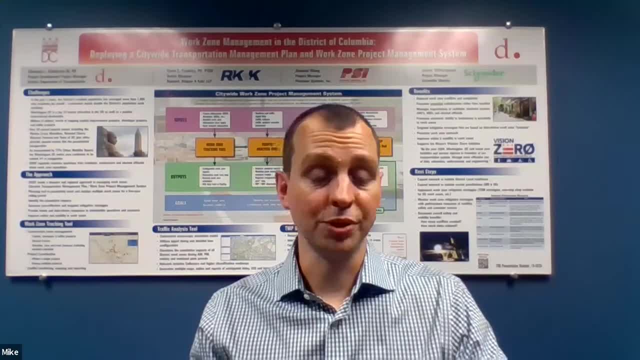 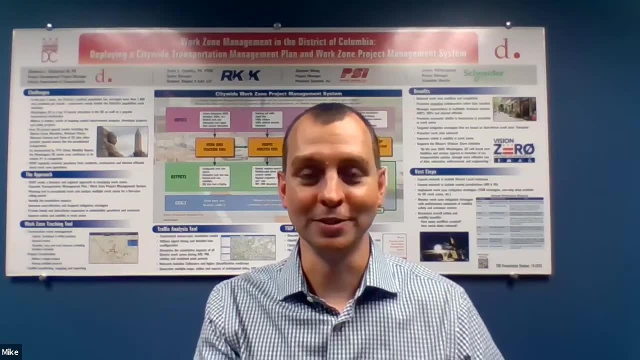 where the best situation for the road is. So we're looking at, and it depends a little bit on if it's a brand new road, if you have like, if we're putting a new road through a field, that's a little different than if we're redoing an. 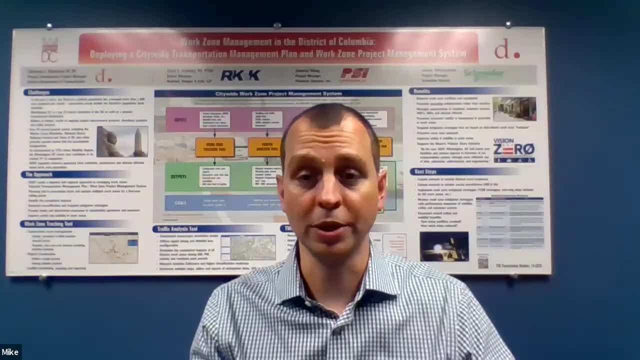 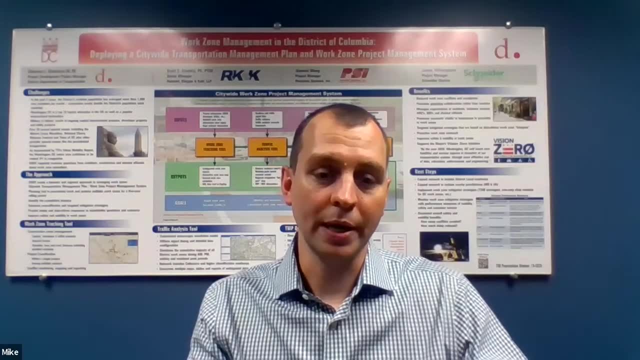 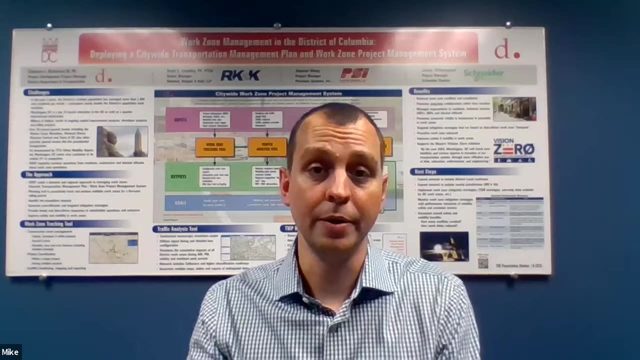 existing road. Most of the work that we really are doing is reconstruction of an existing road. So we have kind of where the road is already laid out, but then we have to look at what the different uses are going to be, working with our traffic engineers to figure out how many lanes are needed, how many. working with the. 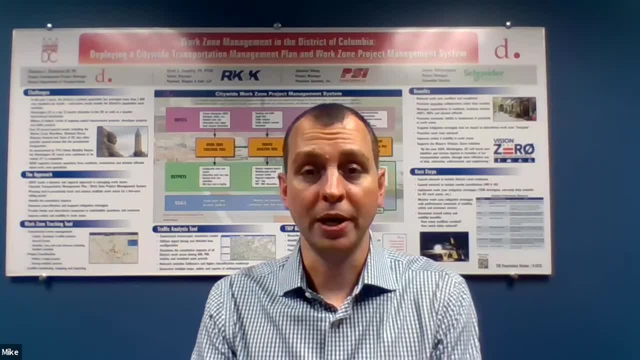 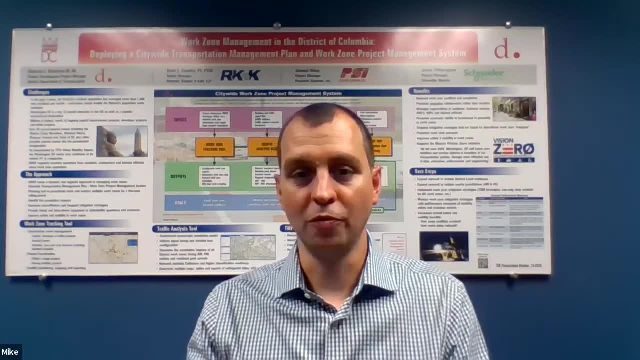 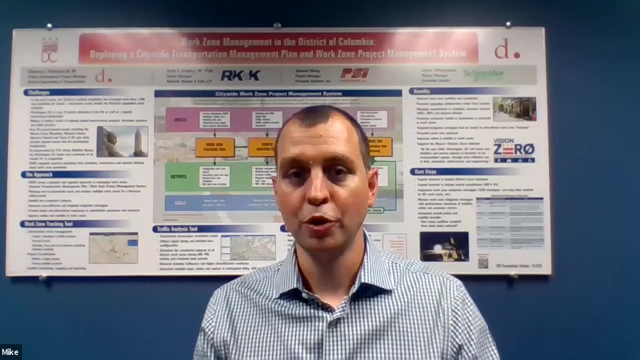 municipality that we're working with to determine what type of pedestrian and bike facilities should be along those roadways. And then, once we get kind of each of the different elements of what the road roadway should all entail, we then go through and kind of lay it out, create a concept, make sure that it is. 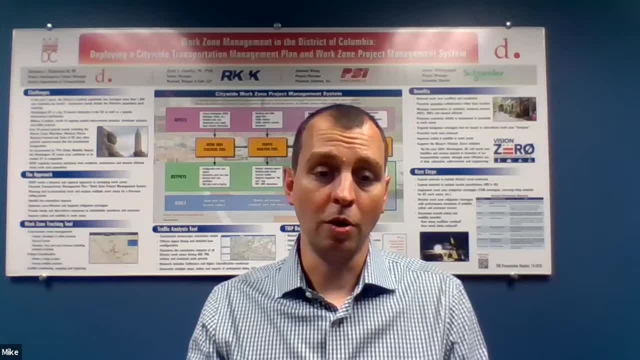 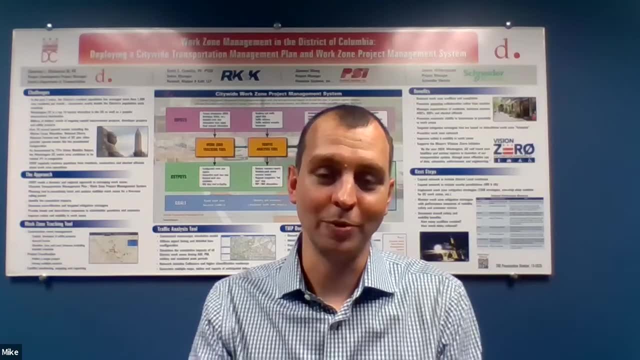 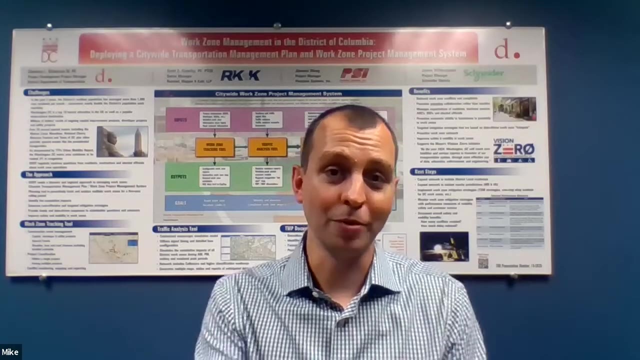 meets all the requirements of both the national standards and the local standards, and to most of which are. I mean we start off with the roadway requirements, which are largely making sure that drivers experience a smooth drive through the roadway, Making sure that they can do it at the appropriate speeds and hopefully not too. 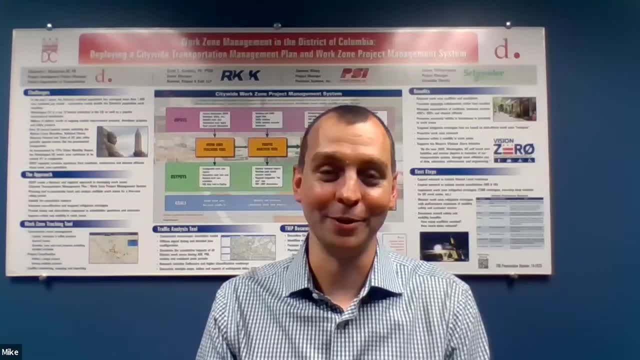 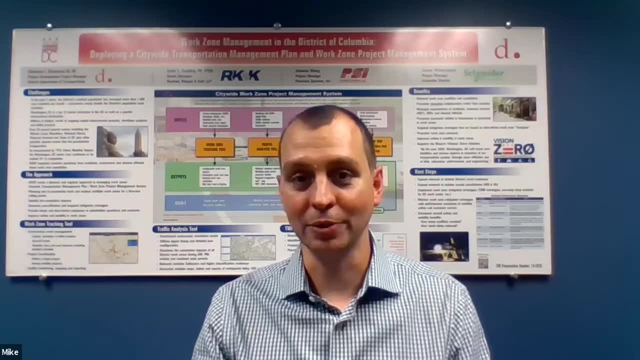 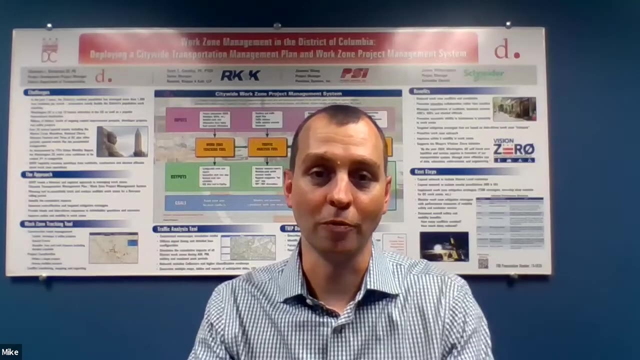 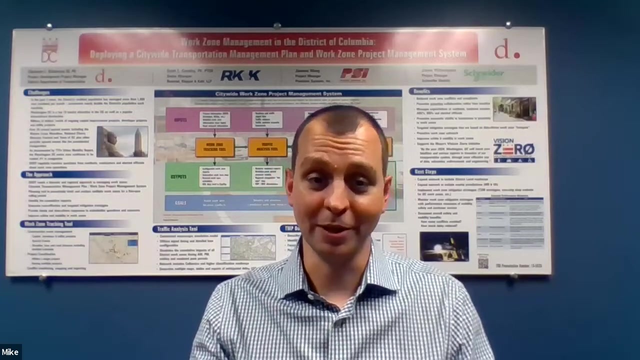 fast either, And then also then going from there checking to make sure that we are doing things- the sidewalks- and all meet ADA compliance, that we are having those bike connections through, that we are actually creating a system that's going to work for everyone. So we kind of lay that out to create a concept, or multiple concepts, depending on. 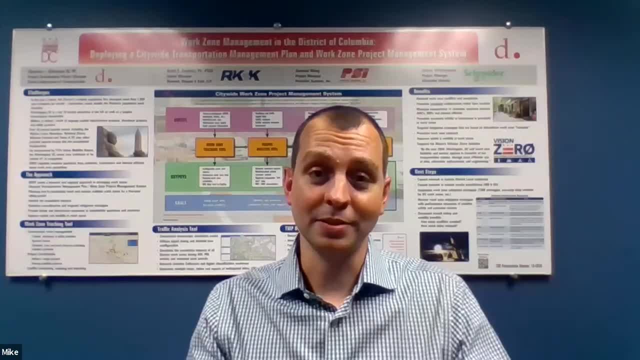 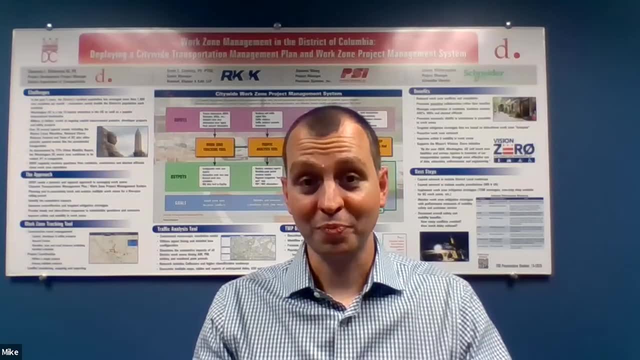 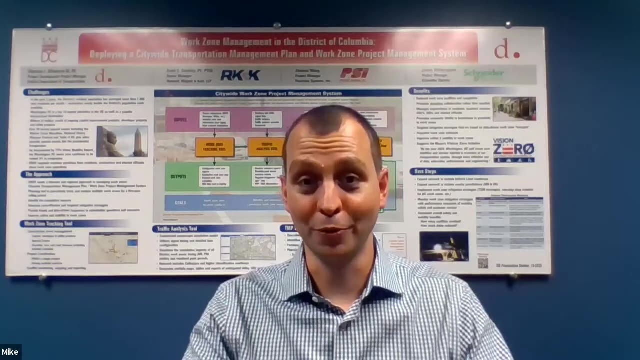 what's happening in the corridor and then, once a concept is selected, then we actually go through and go more through the details of it. So with with roadway engineers, we look at once again I say the alignment, so really the horizontal alignment where the road goes through the corridor, and then we also look at 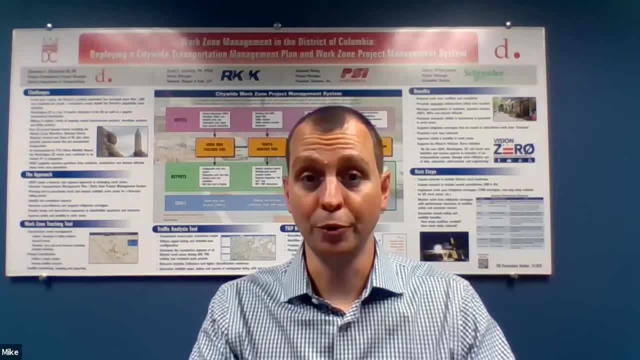 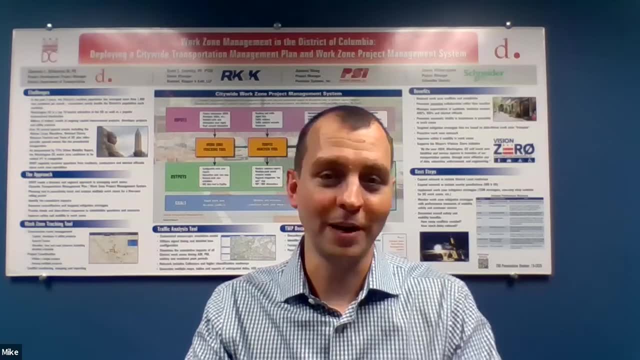 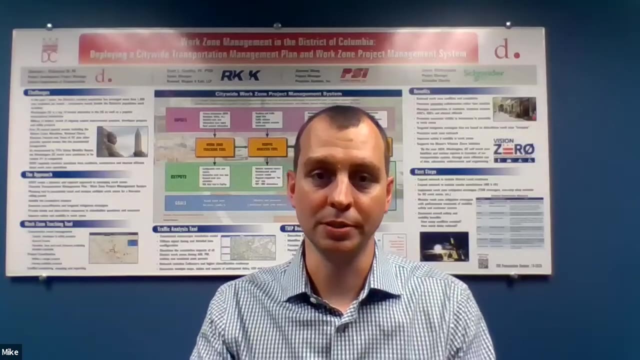 vertical to make sure that the profile, the road is smooth, meets the requirements for all of the vertical curves as well. And then we do kind of more fine graining, grading around each of the intersections, ensuring smooth connections, like I mentioned before, ADA compliance for sidewalks, all of those to 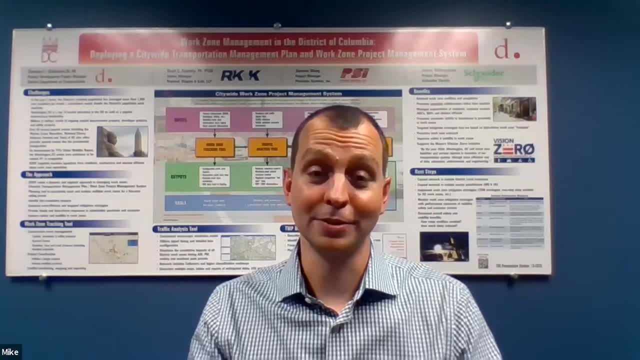 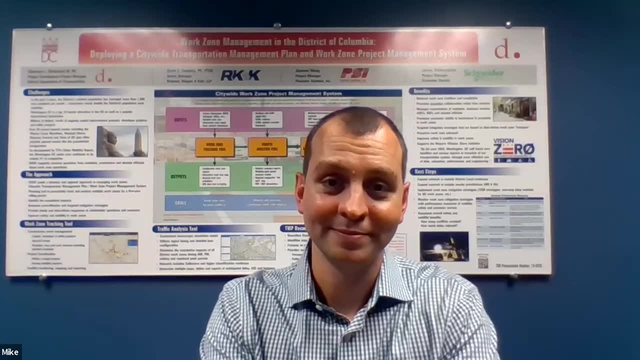 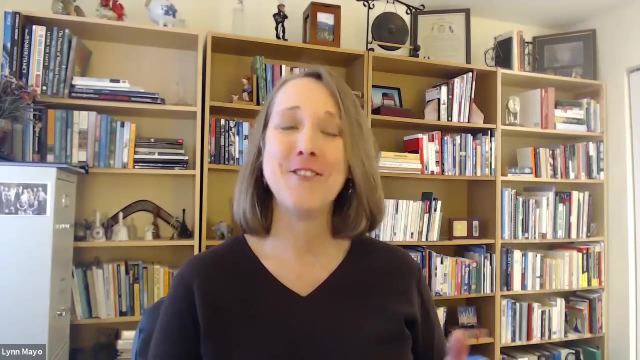 really get into the details of how everything connects, that it's constructible and that we end up then with a fully designed, usable facility. That's a great explanation, and I love your term. I forget what you said exactly, be it an acceptable design speed or appropriate speed. so hopefully get not people not going too slow, but also not. 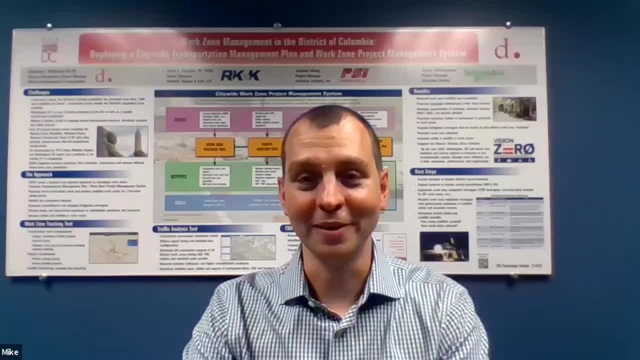 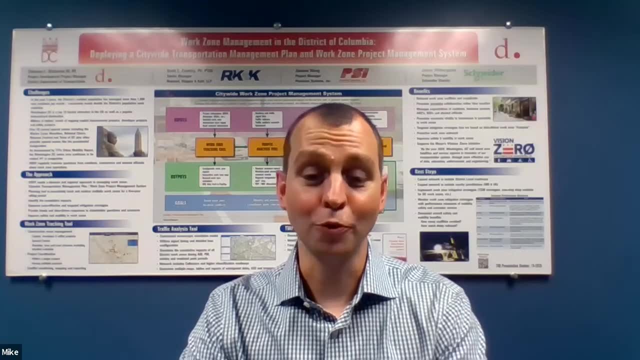 going too fast. Yeah, I know that is one of the big things that's kind of a push in the industry right now is looking at target speeds so that we instead of normally we design to a design speed. so it's everything has to meet that minimum. 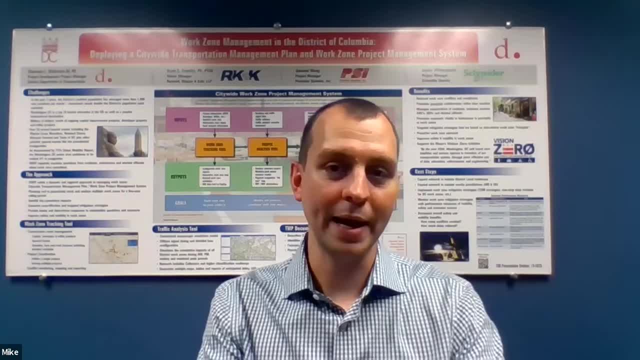 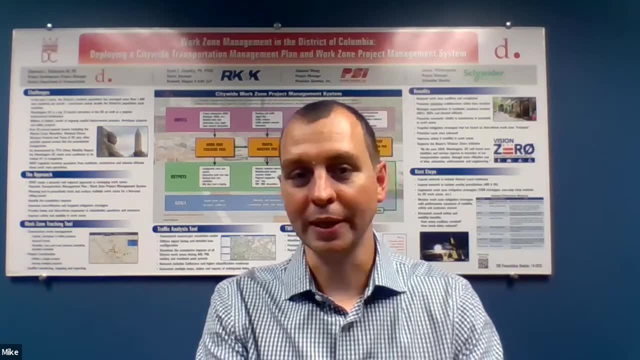 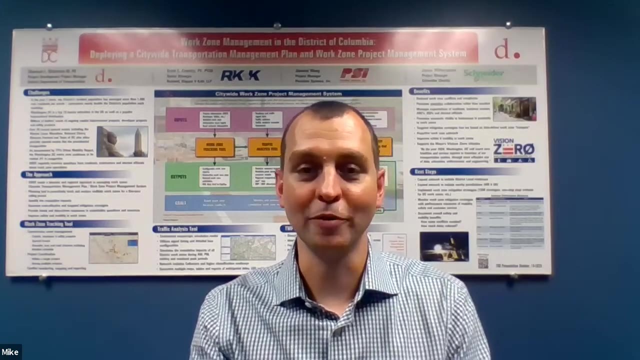 design speed but we don't look too much at what the maximum speed somebody could drive through a corridor is. Now it's starting to change. that we're looking at to improve safety, bringing down some of those top speeds, doing traffic calming through corridors to really get everyone so that it's a more consistent 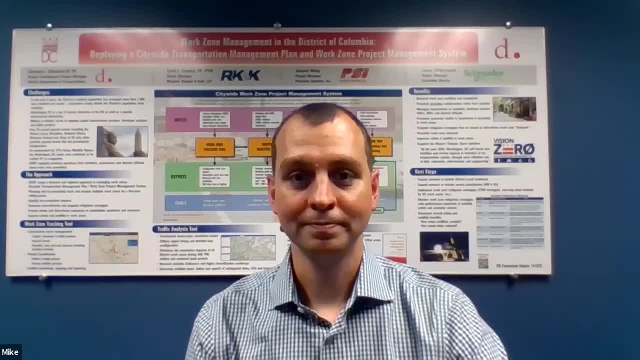 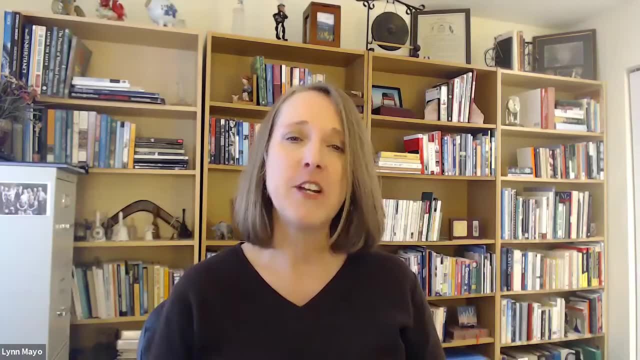 speed through to create a safer environment. Yeah, yeah, that's really important, especially in those urban areas, it's really important. So it's a kind of good overview of what transportation engineers do as far as like a typical day at work, and I recognize that's a. 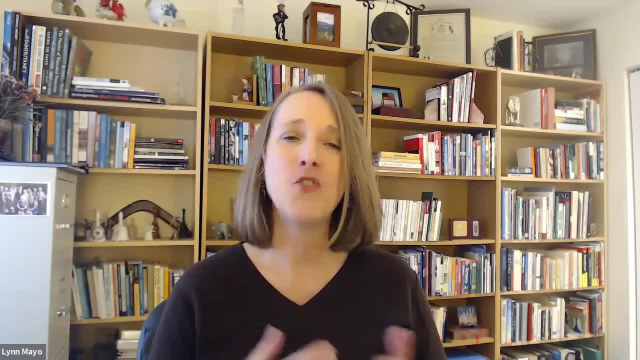 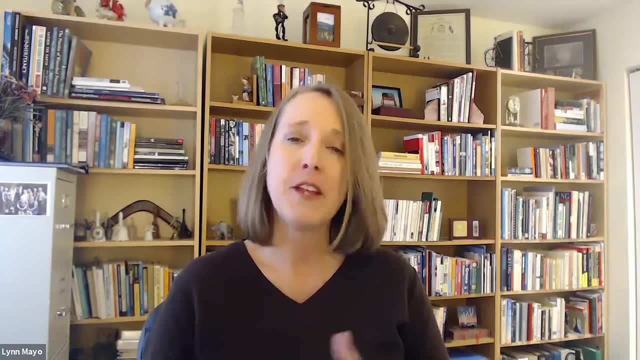 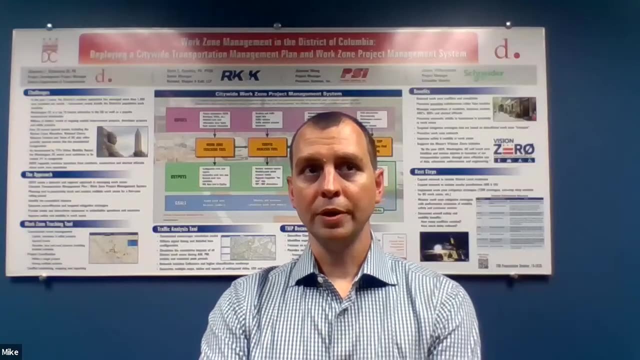 challenging question. but what would you know typical transportation engineer, maybe early in their career, do? What would they do on a typical day versus later in their career? like yourself, you know what type of things you do on a typical day. Okay, yeah, um, early on in your career you kind of are dealing a lot with the the 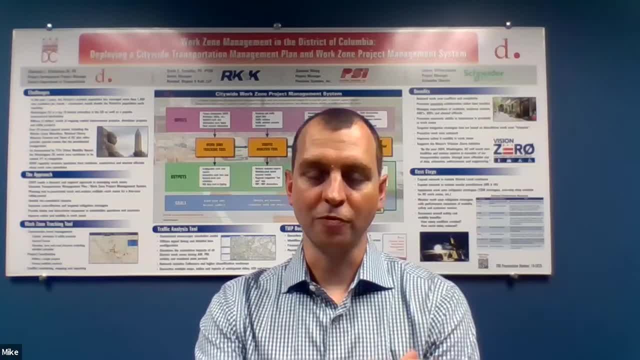 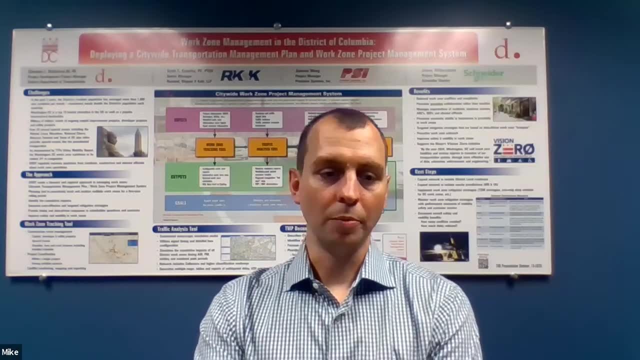 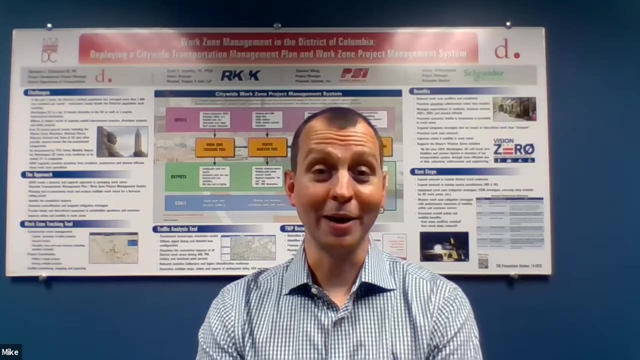 day-to-day. it's singular design. you'll be looking at kind of one project going through and digging into the design of one aspect of it. It could be creating a graphic for one of the concepts Um, or I know a lot of. in my early years it was a lot of doing drainage design, So I 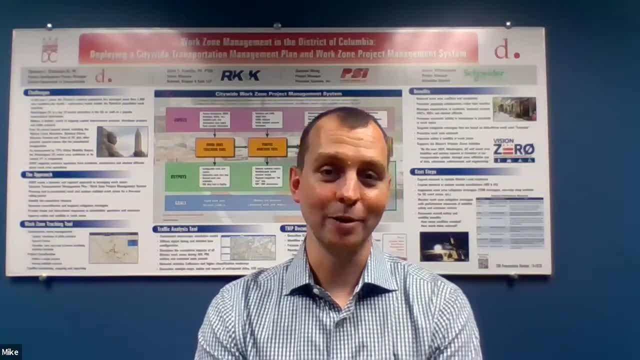 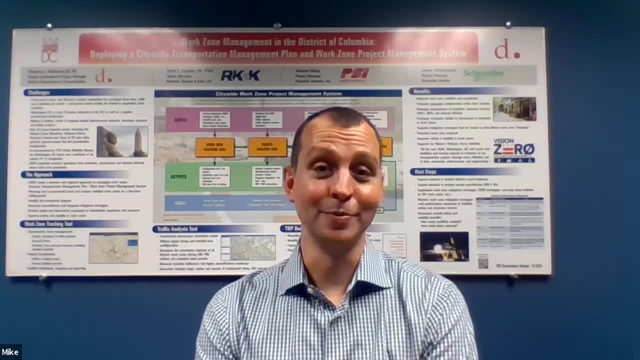 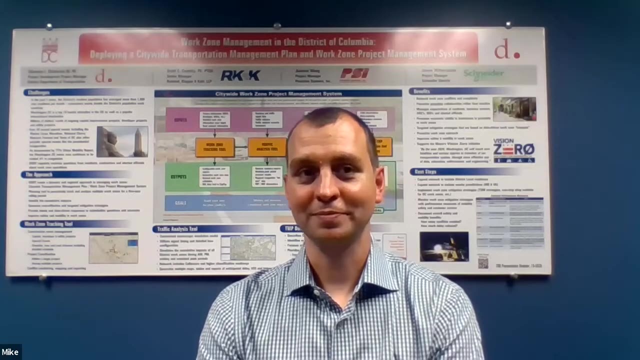 would end up having to do the drainage calculations, laying out drainage areas, inlet calculations for the water to get in the storm drain system and then pipe calculations for how it gets through. Um, so it'd be a lot of that, a lot of I mean. it's not the 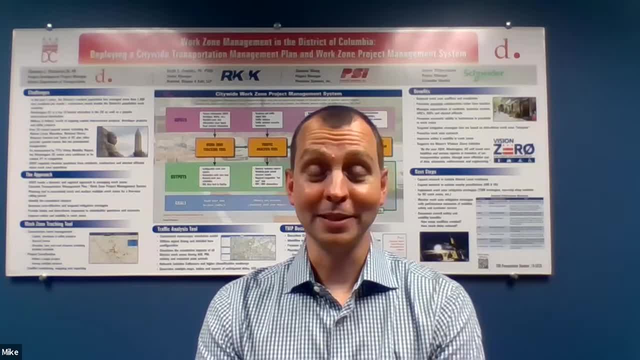 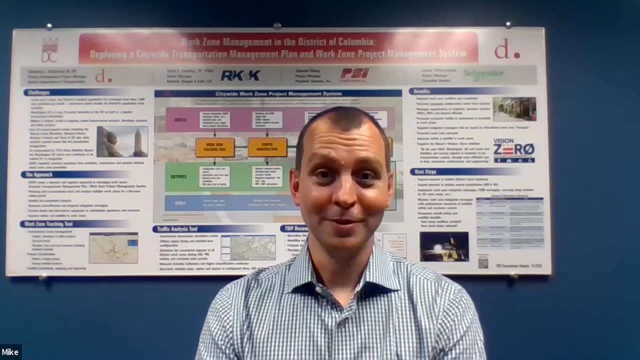 most fun thing but checking grades and and uh slopes to make sure that we are meeting ADA compliance. on sidewalks, designing a lot of curb ramps, because you may see curb ramps on the sidewalk but what you don't realize is that the design that goes into those is every 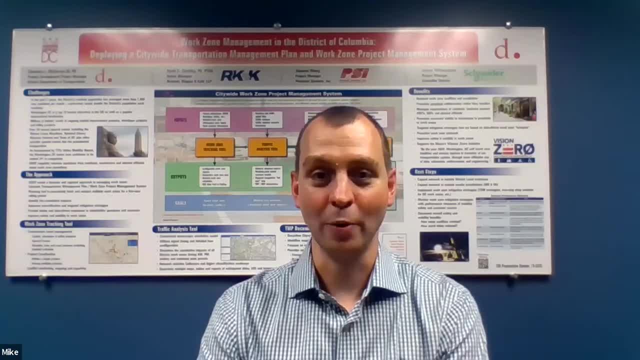 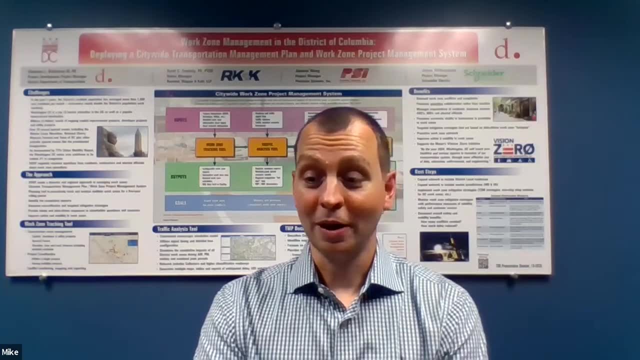 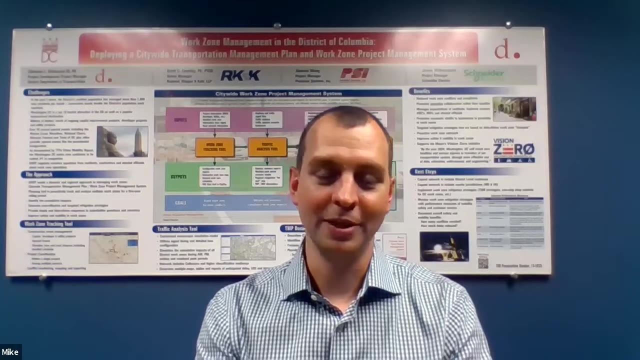 single point on them has a very specific elevation, so that way we make sure that it is an accessible ramp so it meets the requirements and is usable. So it's a lot of working on the fine details of that, Um, normally early on. I mean, it depends on what projects you're on a little bit, but if 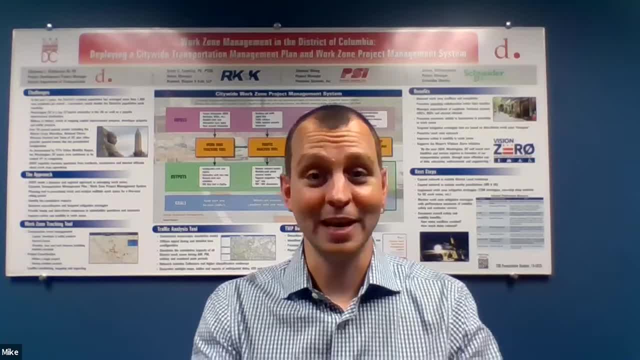 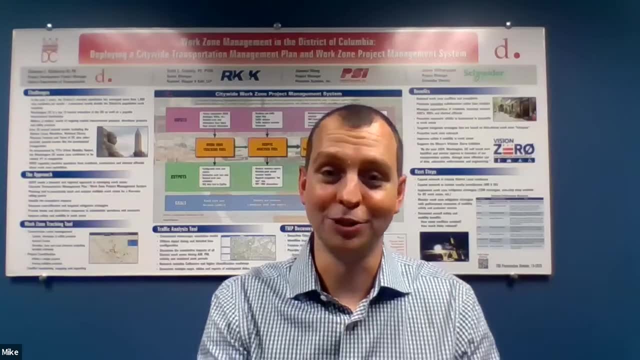 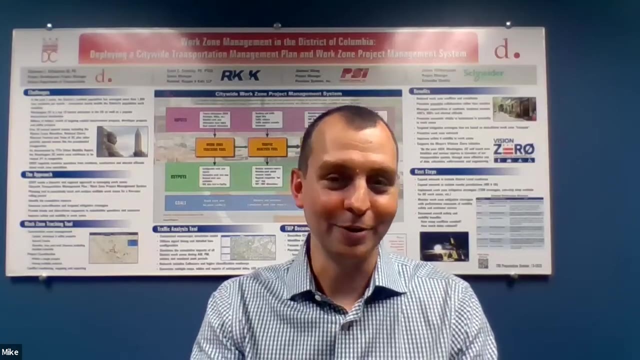 you are on a large project, you will kind of have just that project that you're working on. so you get to know, and one project very, very well, you also may at times have a bunch of little projects which you're doing pieces here and there of. so it can kind of vary a lot depending on what projects you're. 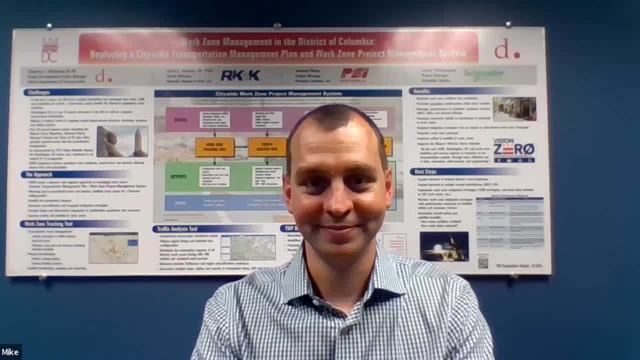 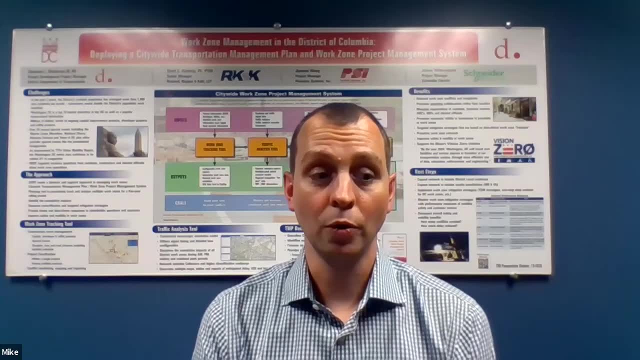 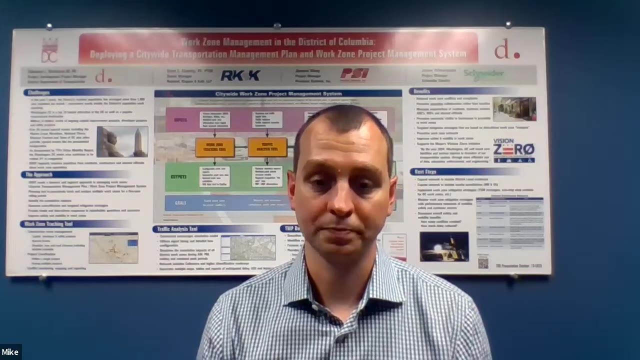 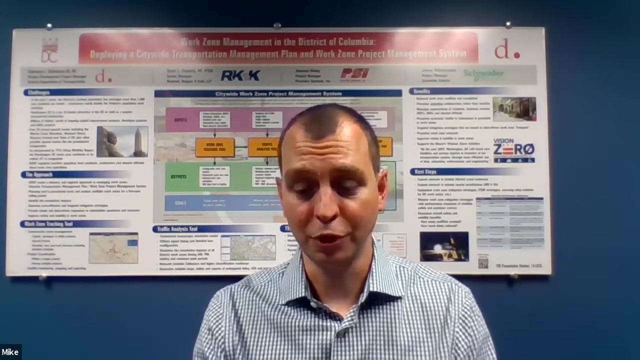 working on and what opportunities you have. okay, great, they mentioned a DA. what is a DA? oh sorry, yes, it's the American Disabilities Act and so that's to make sure that all people are able to use the facilities, that, even if they have a disability, that they are able to use, use the facilities. so, like I mentioned, with 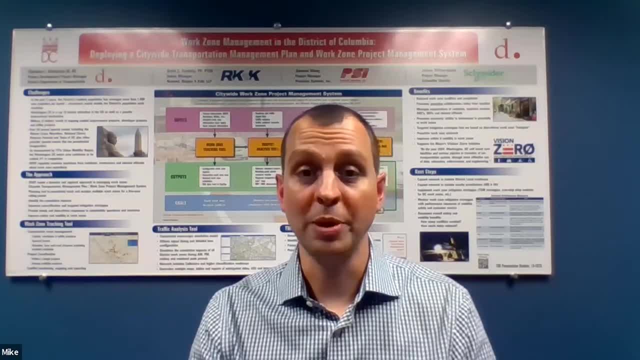 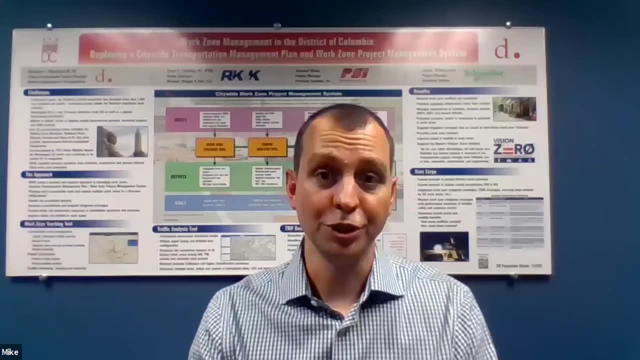 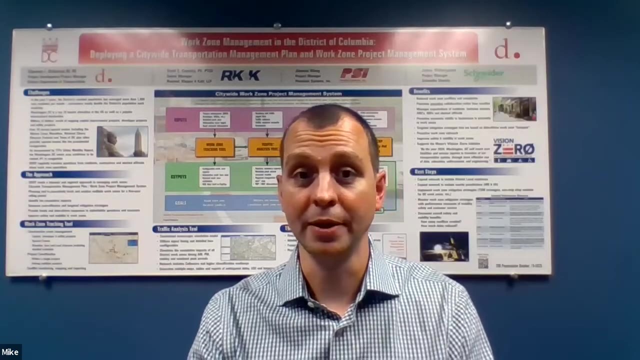 the curb ramps. they are designed so that way people and wheelchairs can use them. that people who might have a impaired vision, There's detectable warning surfaces that they can pick up with their canes. When we do traffic signal design, there will be audible pedestrian signals that alert them to. 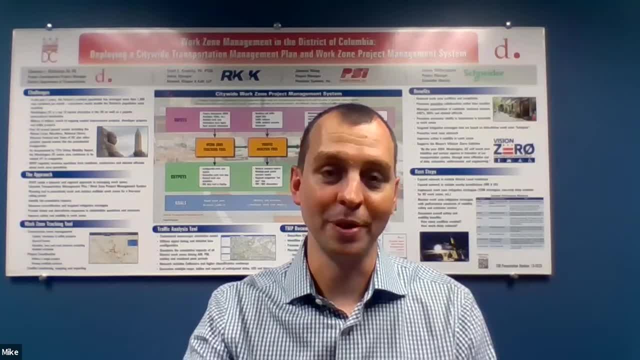 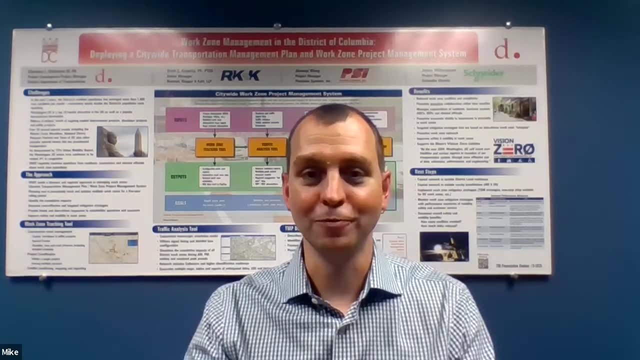 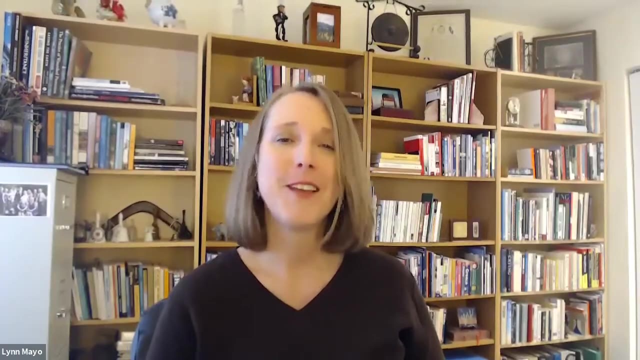 not only when the light or when it's safe for them to cross, but also alert them which directions to cross. So it's really just looking at all the infrastructure pieces to make sure that it is usable for all users. Yeah, so that's important work to keep everyone safe. Yes, So you talked. 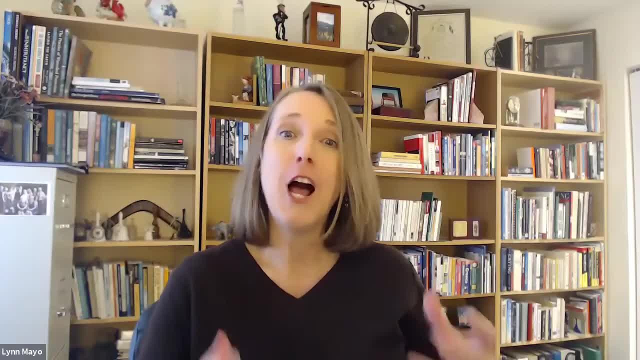 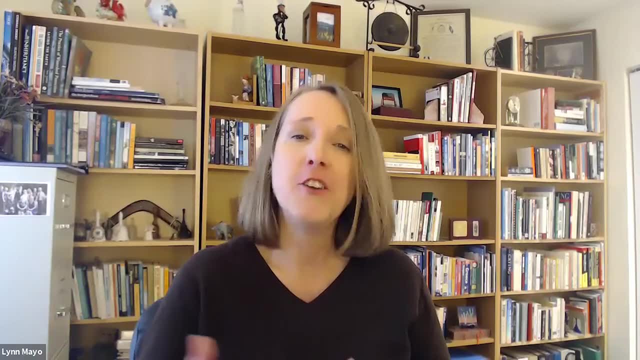 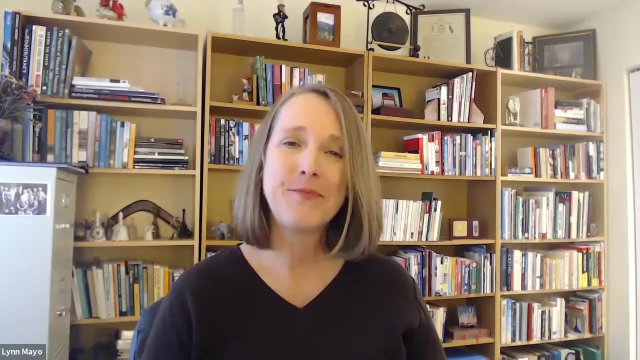 about, kind of, in your early years you maybe do a lot on one big project or, you know, do parts on small projects. After you have 10, 12 years or more experience, what's your typical day like for you? What's your typical day like now? So my day now I'm managing a couple of different. 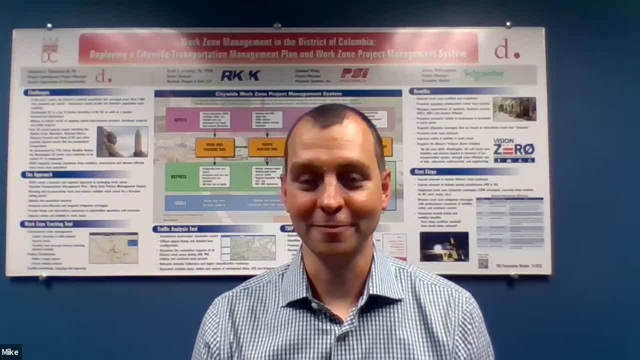 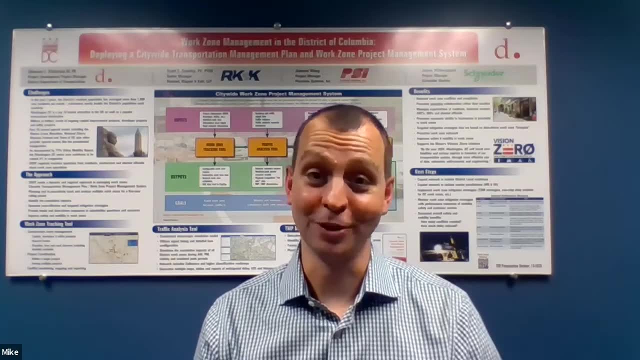 projects. So it kind of depends on what I'm doing. I'm managing a couple of different projects So it kind of is a lot of checking in on everyone and what's happening with each of the projects. So, as we mentioned before, with transportation engineering, we have all of those different. 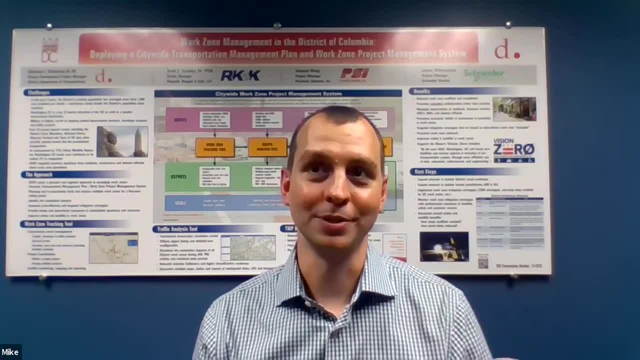 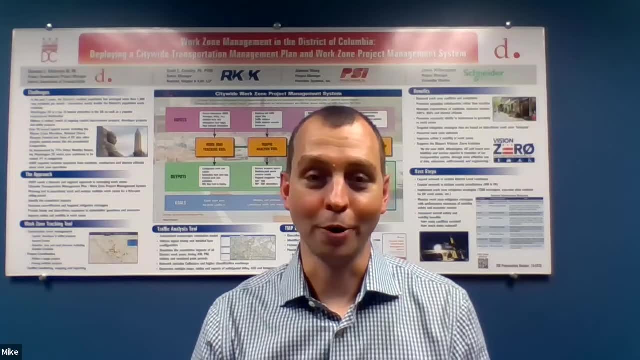 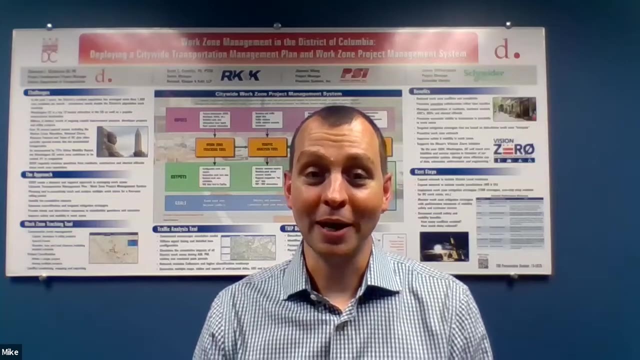 specialties from traffic and structures. But then we also have people working on our projects for environmental resources, water resources, landscape architecture, utility coordination. We have surveyors on it. So I actually end up with most of my projects checking in to see what the status of each of the different things. 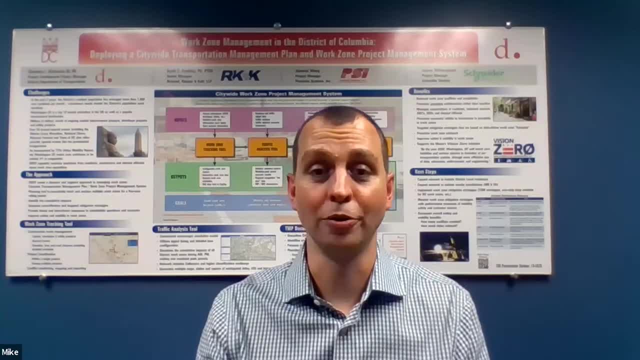 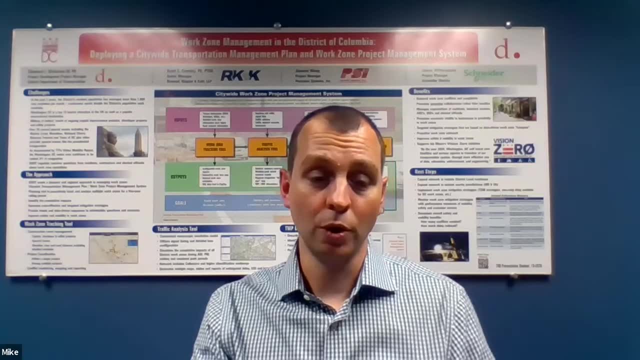 is each of the different disciplines where they are at with their design. I still am very heavily involved in the roadway design side of things, So overseeing the roadway engineers that are working on the project, but also jumping in and doing some of that work as well. 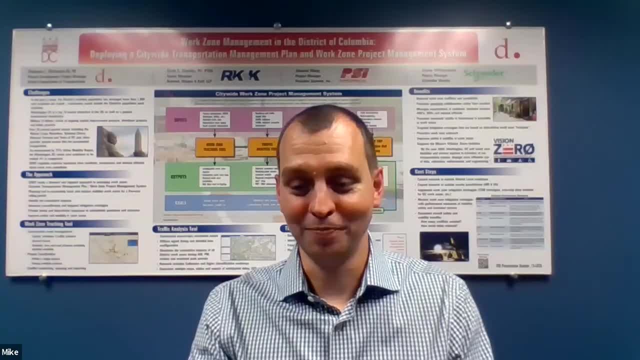 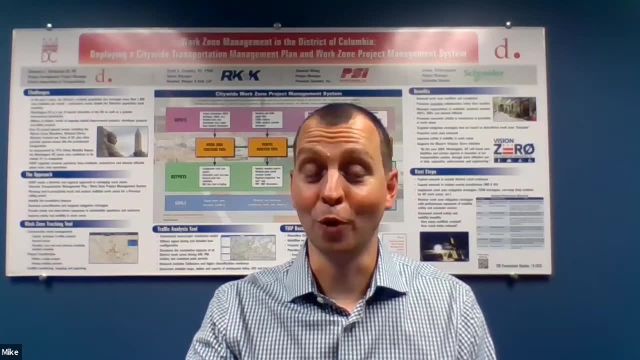 And yeah, and then also, as you move up further and further, you spend more time on the roadway design side of things. So I'm very heavily involved in the roadway design side of things. I'm also working on business development and trying to bring in new works, new projects. 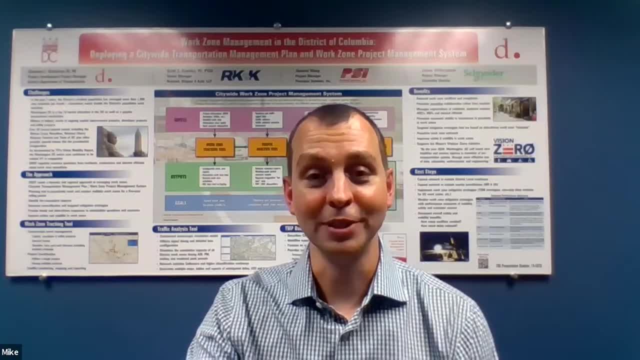 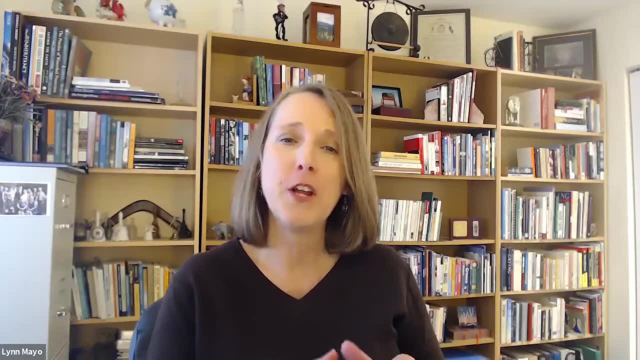 and being aware of what's out there and where the industry is continuing to go. That's interesting. So basically, at the beginning of the career it's maybe very focused in a different area, But by the time you get to your level you're really involved in all different 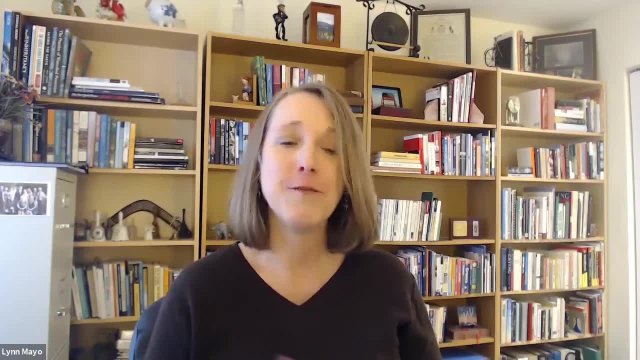 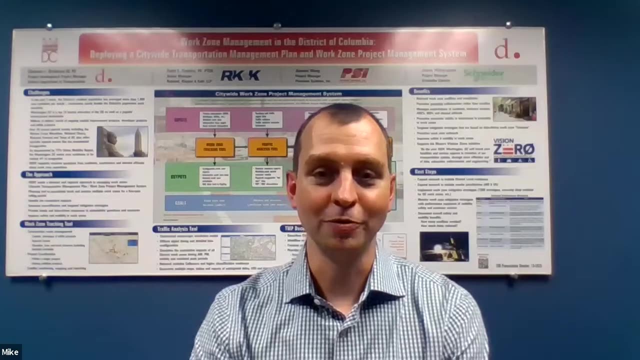 types of engineering and projects and transportation. But what type of? for the younger people, what would they, how much time would they typically spend out in the field versus the office if they were a transportation engineer? So I think it kind of depends a little bit on which type of transportation engineer you are. 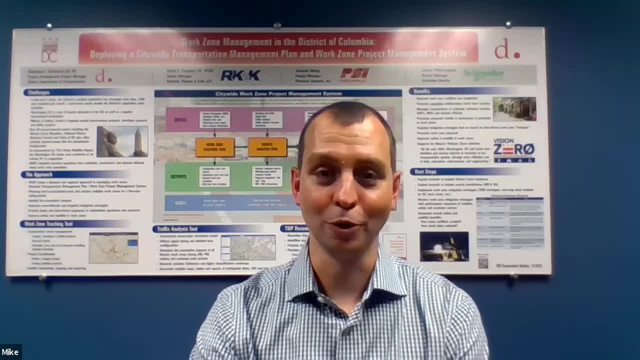 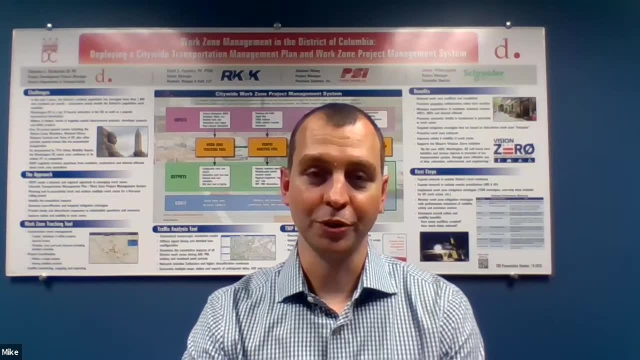 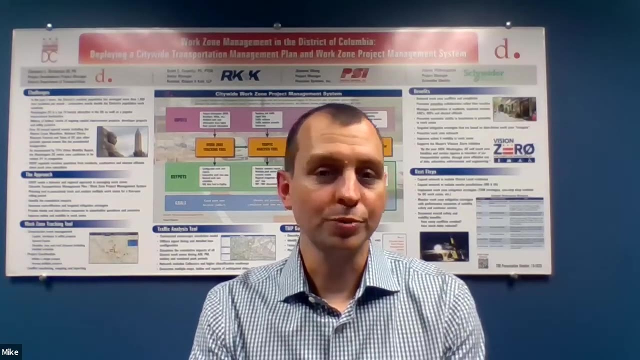 Because I know some of our structural people spend a little more time out in the field because they'll be doing inspection of existing structures that are out there. So I know once again for me I'll just kind of talk a little more from the roadway side of it. On roadway we don't spend. 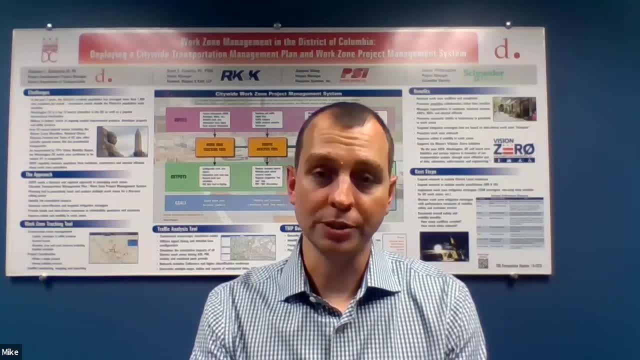 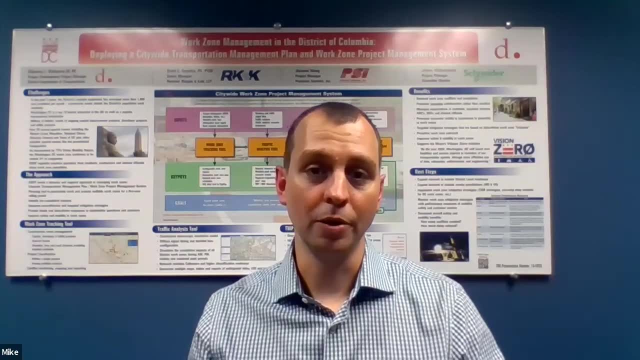 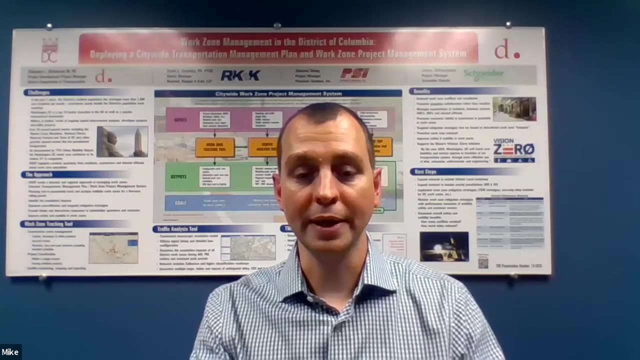 too much time out in the field. We'll do initial assessments out in the field because kind of with the design process we end up getting a survey and you kind of take a look at that and lay out. or on GIS information, you lay 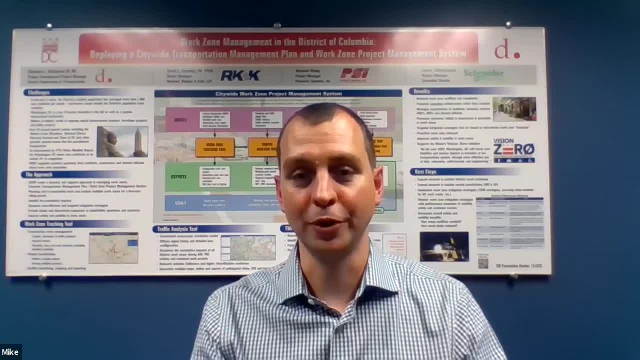 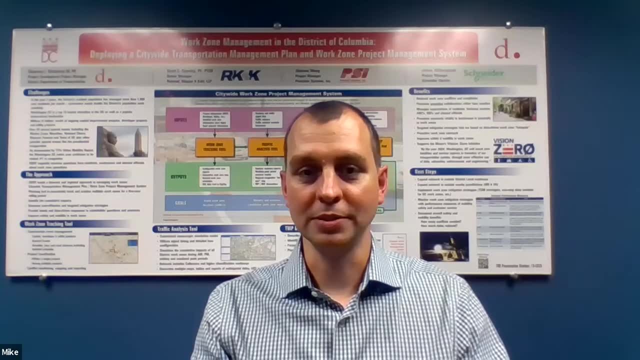 out where the roadway is going to be, what the features are going to be, all of that. But a lot of times you can't really get the feel of what the project looks like until you're out in the field and really get it. 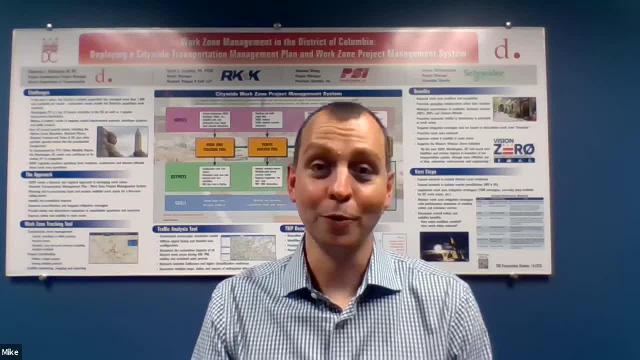 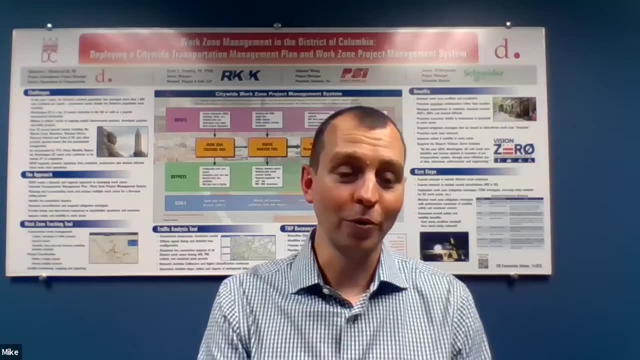 Get a feel of what the existing conditions are. So almost every single one of my projects I've gone out to the field at some point to walk it. make sure that I agree with what was surveyed, agree with the recommendations that we're making through the corridor. 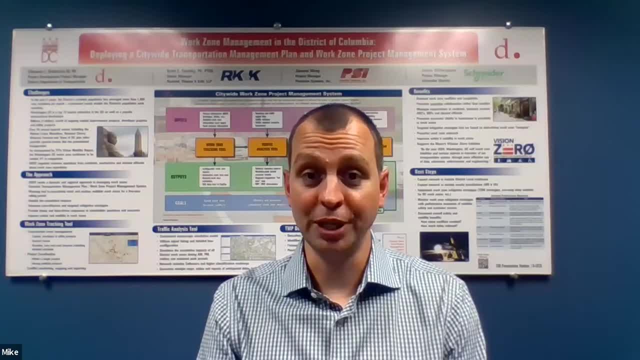 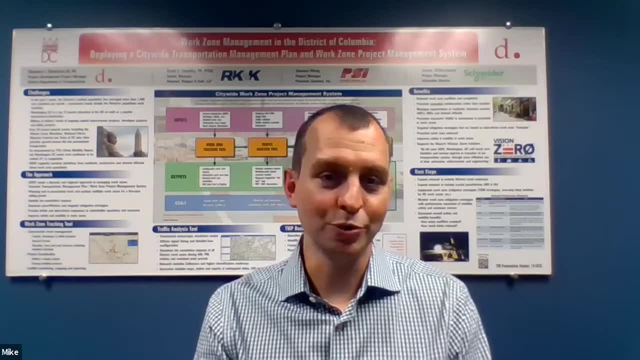 see if there's anything out there that we may have missed that would change our design. So it's kind of spot site visits here and there a few times through the design process, But most of the work that we do it's really in the office, kind of more of the desk. 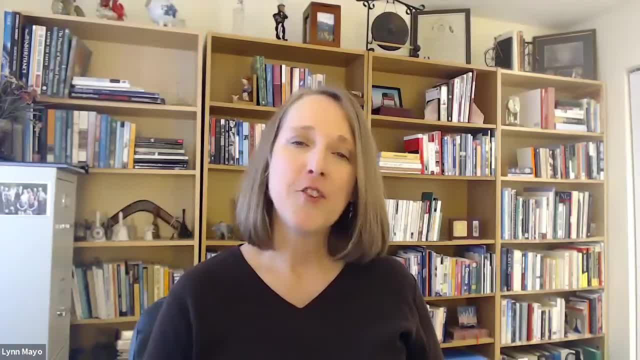 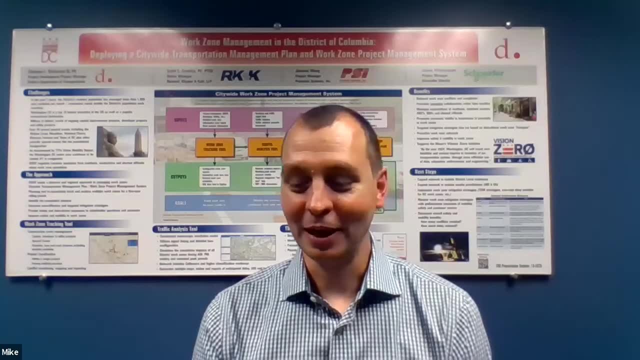 Great. So, Mike, what's been your favorite project? So I knew you were gonna ask me this and I was having a really hard time coming up with an answer for it. Kind of throughout my career, I feel like I've had a number of different ones. There are a couple. 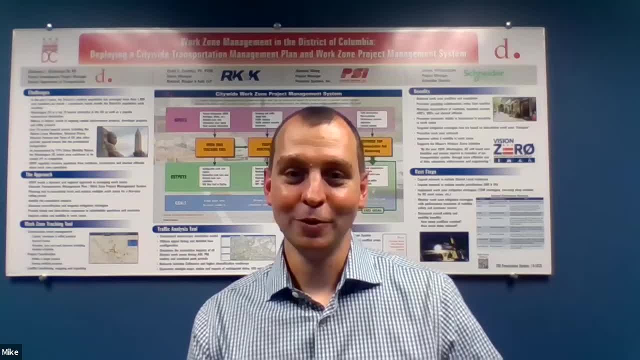 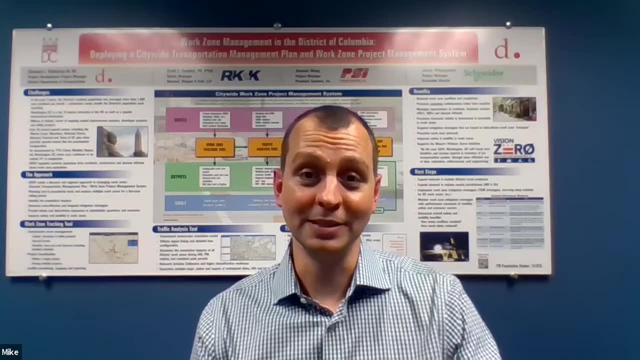 that I would qualify as being the most proud to be involved in. which kind of? I was involved in the roadway design portion of the work. Okay, So one of those was the work development here in DC, which was just a very massive project. I actually 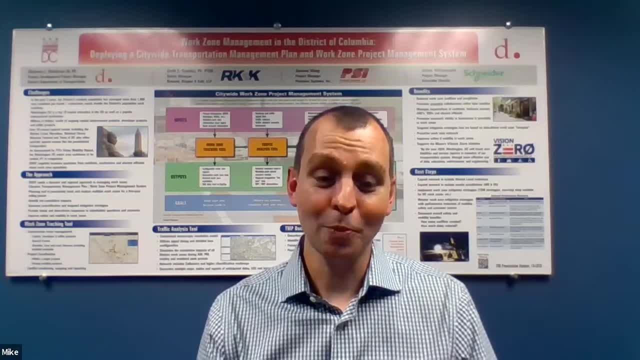 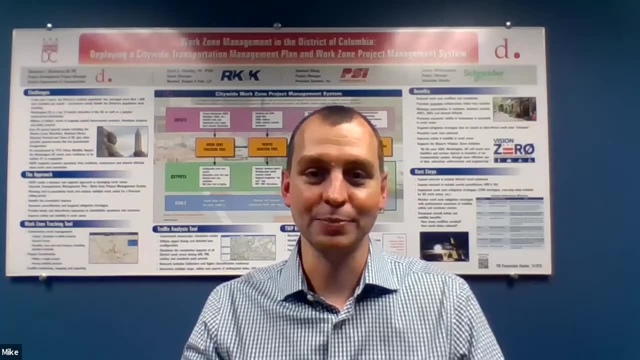 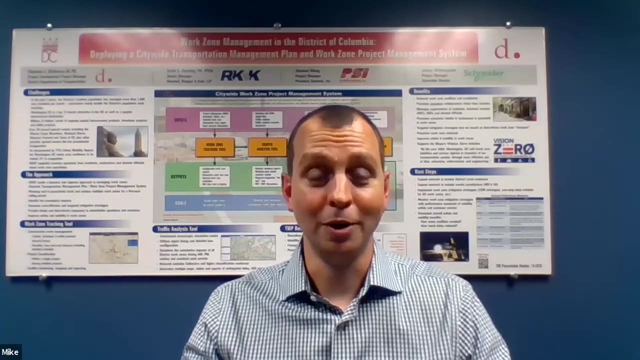 forget how much it was at this point, But one of those where I got to do the road, the redesign of the roadway right in front of that, In every aspect, from looking at some of the drainage to designing all the traffic signals, to doing all the curb placement throughout the whole corridor, So that was one that. 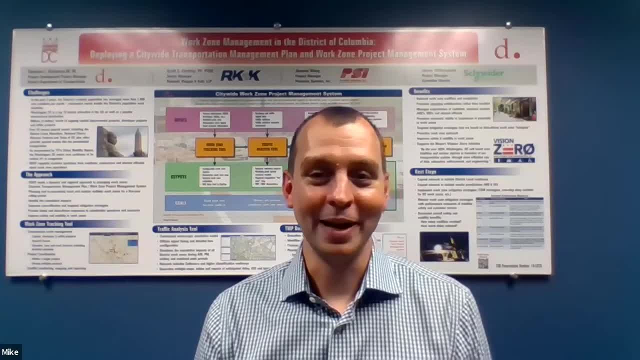 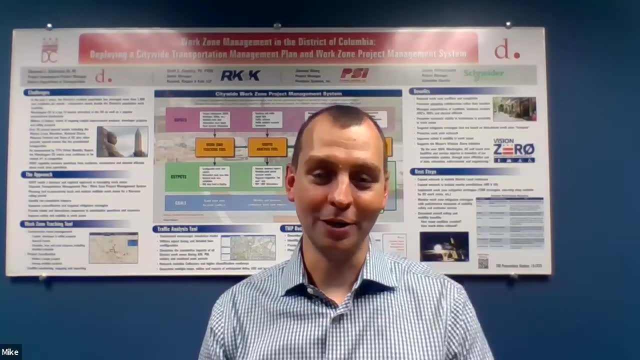 comes to mind, But really kind of right now I'm I'm almost always excited for what my current and next project are going to be. So, as I mentioned, right now I'm working on the Connecticut Avenue project, which, to me 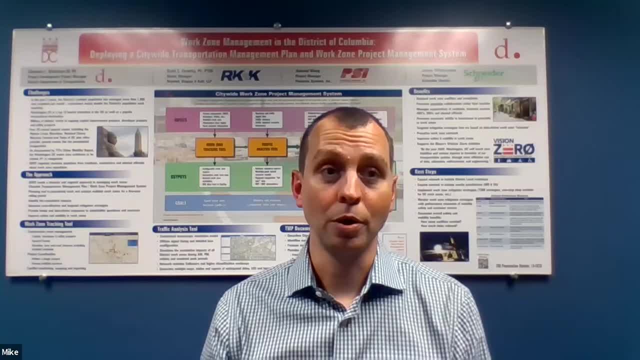 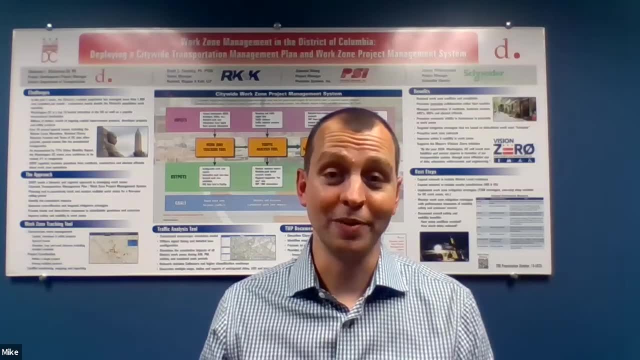 is the one of the most exciting that I've worked on, just because we are looking at changing kind of the nature of a major arterial through DC And then we're also looking at providing a new structure to serve as a plaza, a pedestrian area. 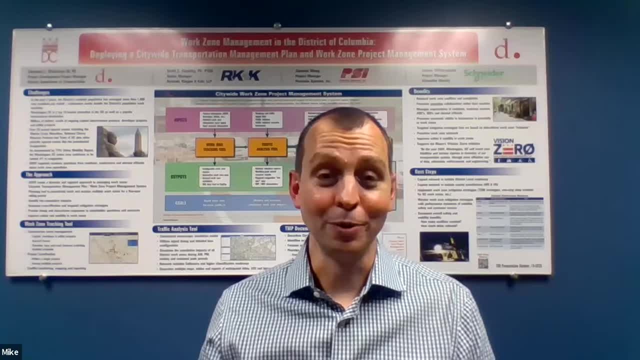 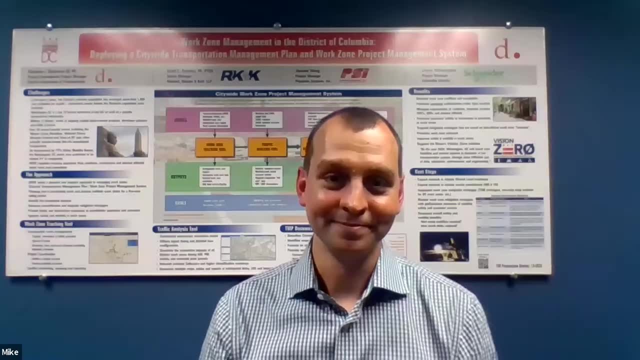 So we're looking at a new pedestrian plaza for for people right by DuPont Circle, So one of the very heavily most heavy pedestrian areas in DC. That's really interesting. I didn't know you worked on the Wharf project- I mean, that's a great project- like you, 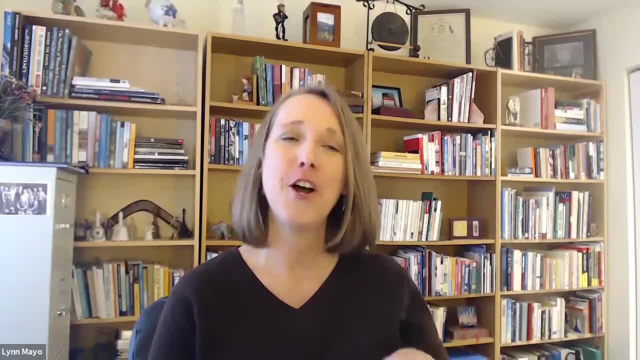 said. Actually, I encourage people to go to repicturecom, Google the Wharf and we actually have a number of project write ups about it. We don't think on transportation yet, So maybe we can get you on that, But that is, that is. 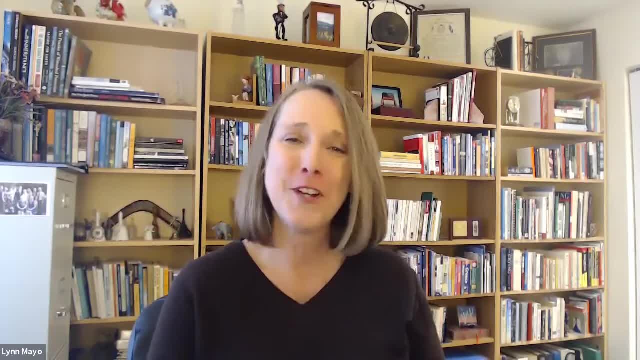 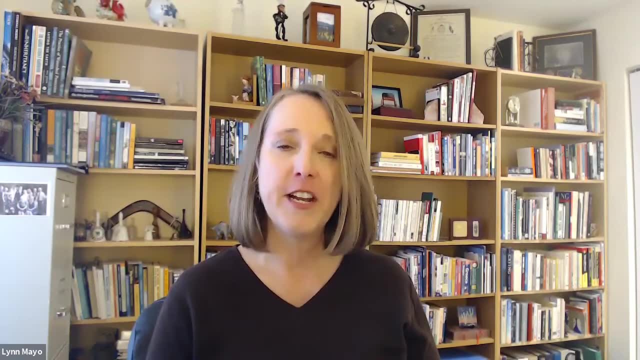 just one, probably one, one sort of light bulb, What's in a lifetime or what's in a career type type project. So that's great, you worked on it. So if students were interested in getting into transportation engineer, you know, I assume, like you, they should be a. 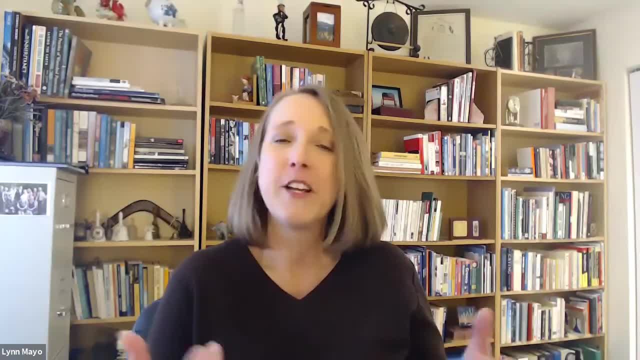 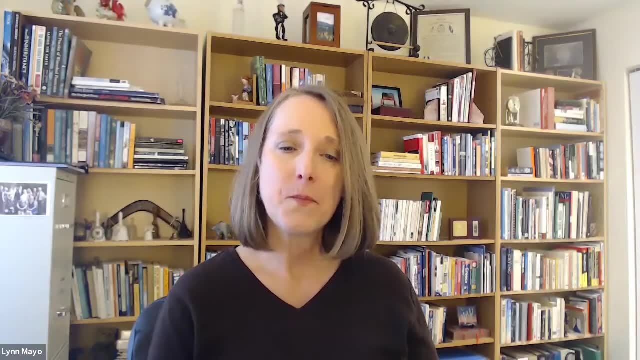 civil engineer. But what? what courses in addition to, like, a transportation engineering course, what courses you think would be helpful for them to take? Yeah, so, as you mentioned, the transportation engineering courses would be at the top of the list any of the times. 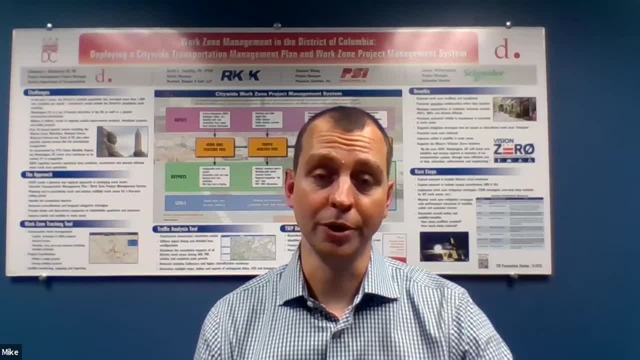 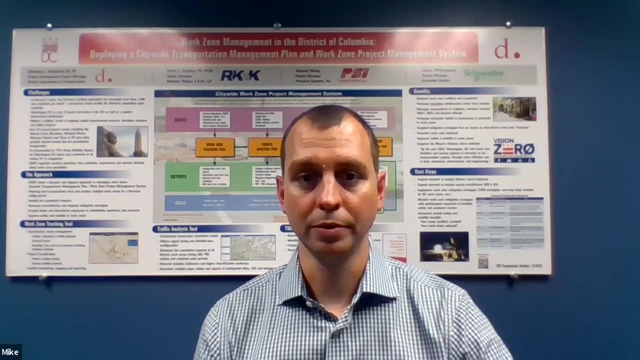 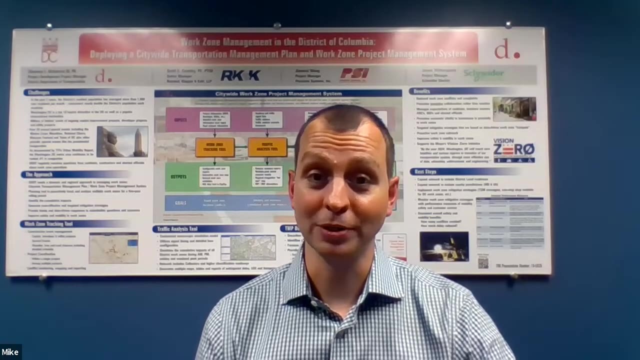 that they have any traffic engineering. It's really helpful to understand any of the traffic modeling and kind of the decision making that goes into modeling and planning and those aspects of it. Public policy courses, if there's any related to transportation also, oddly enough- or I guess not oddly enough, but it's one of those that 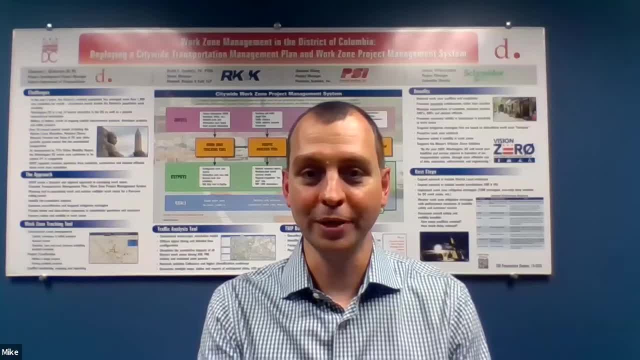 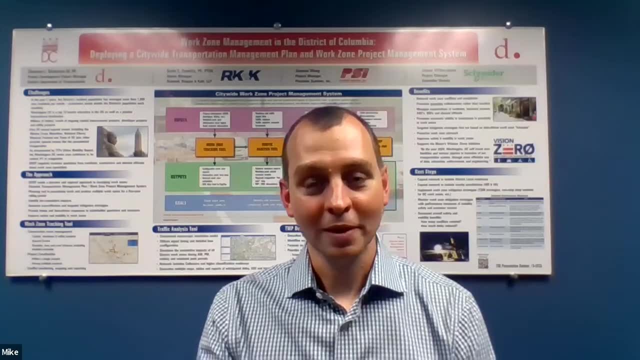 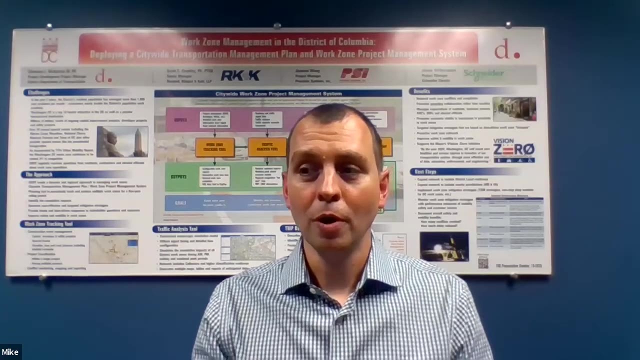 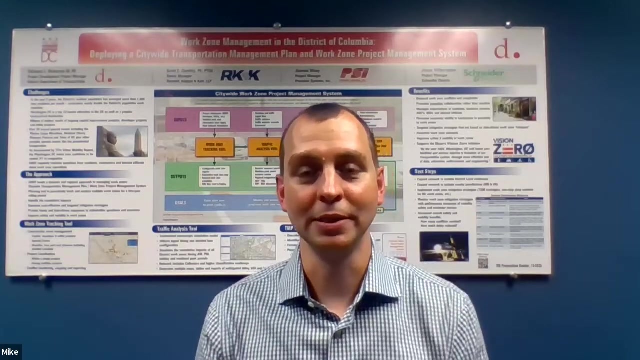 I hadn't realized early on how much zoning actually in property uses goes into the transportation design for public facilities, So kind of. some of those public policy aspects actually are really helpful for figuring out kind of the future of roadways, where things are going to go and what the future priorities of different land uses are. So that would be another. 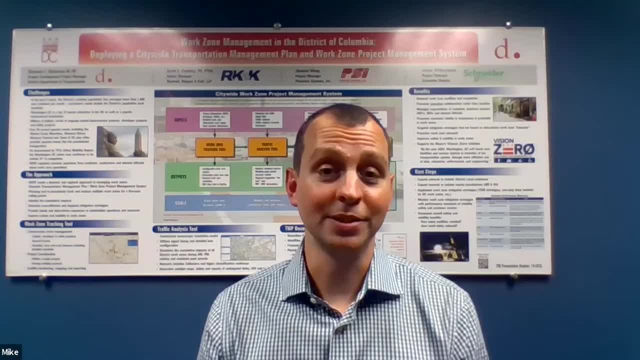 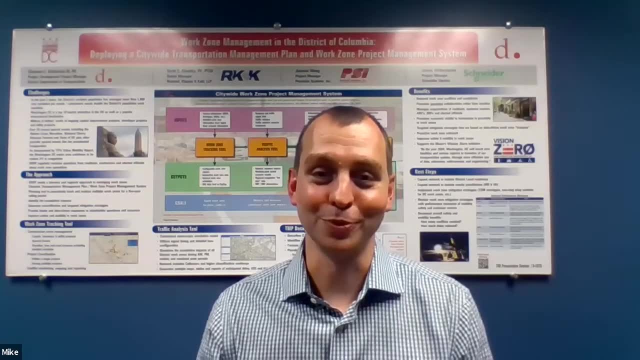 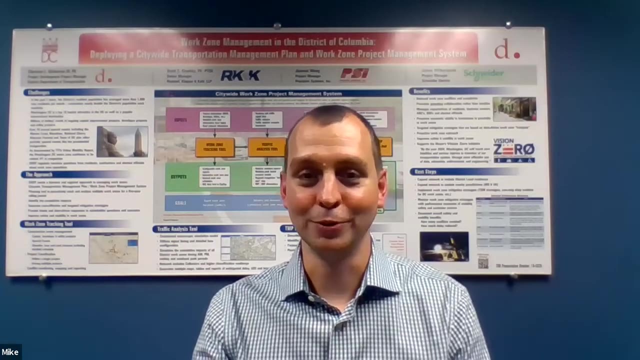 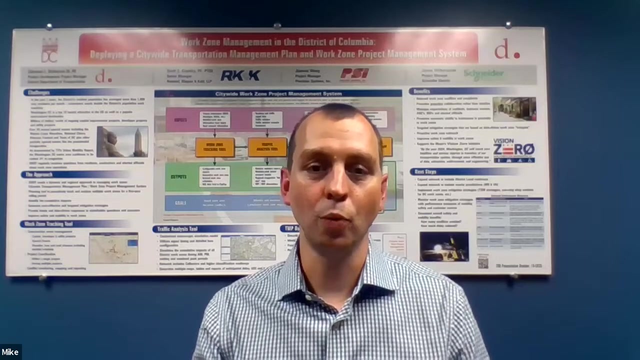 suggestion And then really almost any civil engineering course out there is going to be helpful in some way. as it's come up a couple times, Our projects really just touch on everything. So having a base understanding of the water resources, design structures, design any of those, it really just helps to understand what the other 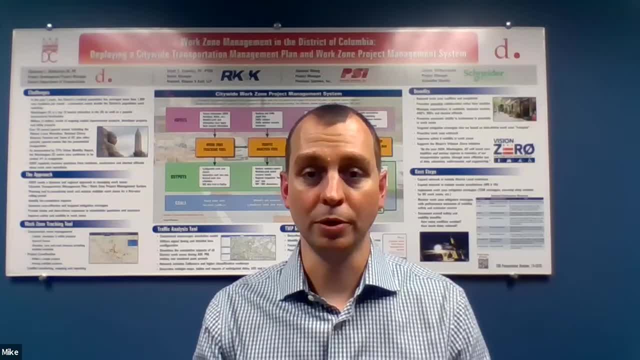 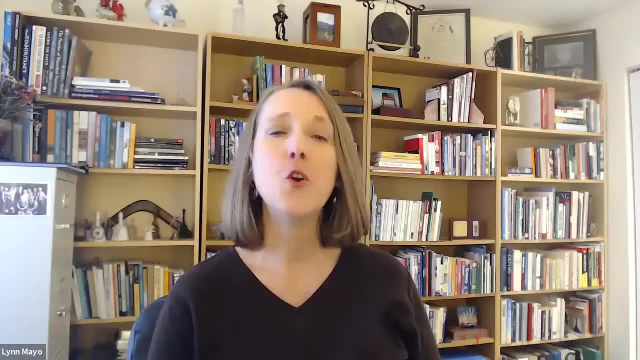 disciplines are looking at And so you can relate to them and also make sure that you're providing them with what they need and that you're getting back really what you need. That's interesting. So even if you don't directly use, say, a structures class, it's still it's useful to have a structures. 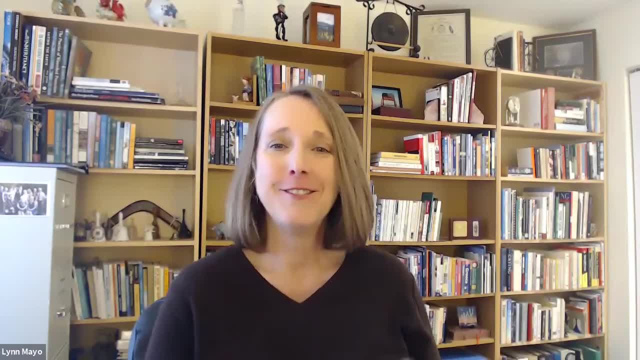 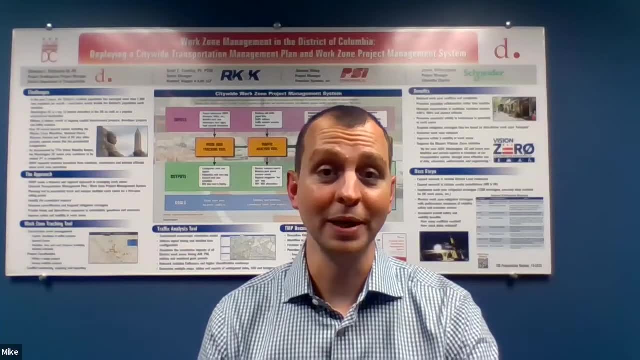 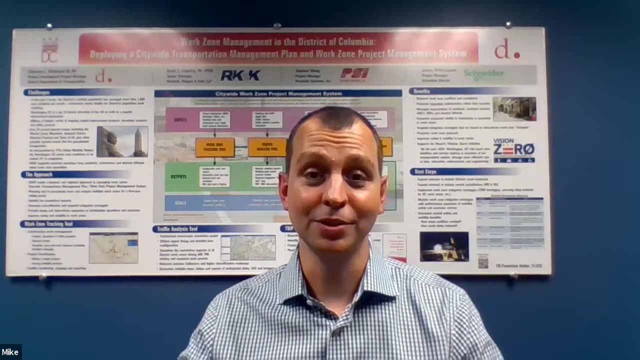 background. So when you talk to those people, you can Absolutely. I actually was working a few months ago on a project that was structures-based, So the main design was for this very large bridge. I was in charge of the roadway design on each. 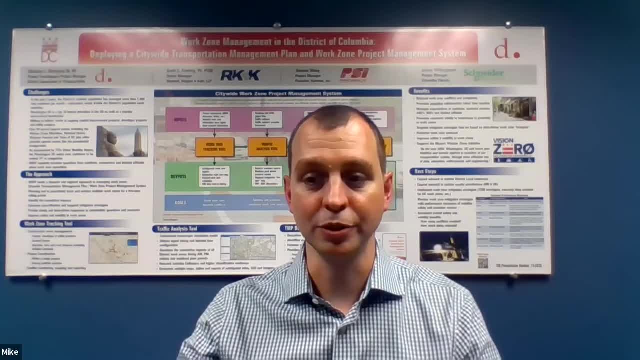 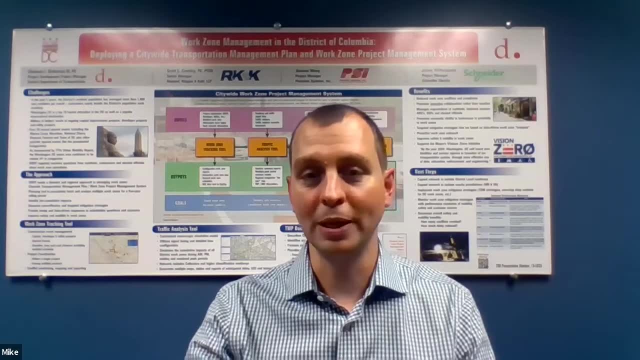 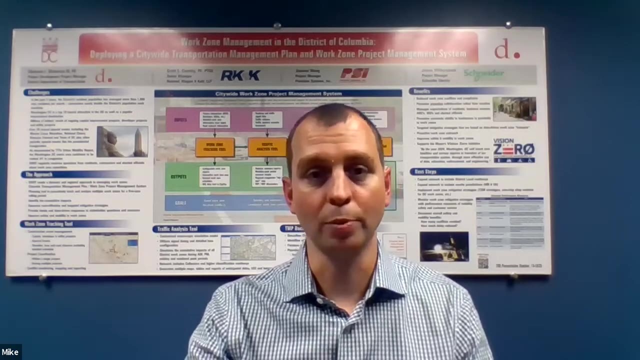 of the approaches and kind of the connections into the existing streets. But being in those meetings and really understanding the knowledge that I knew about structural engineering really helped me a lot, Really allowed me to talk to the bridge engineers and make sure that with the alignments that we 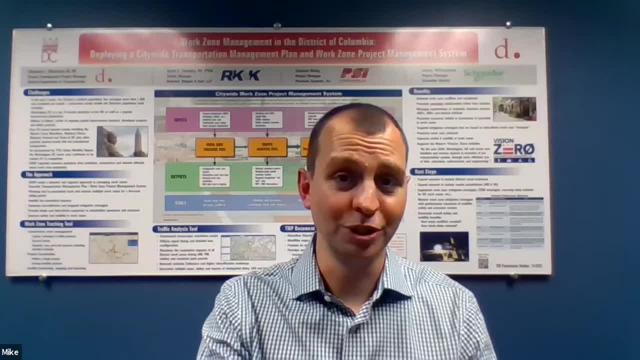 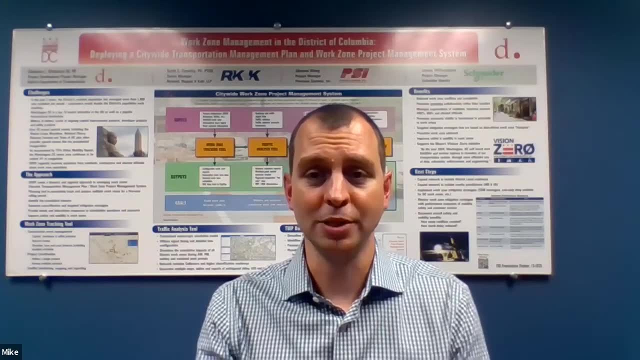 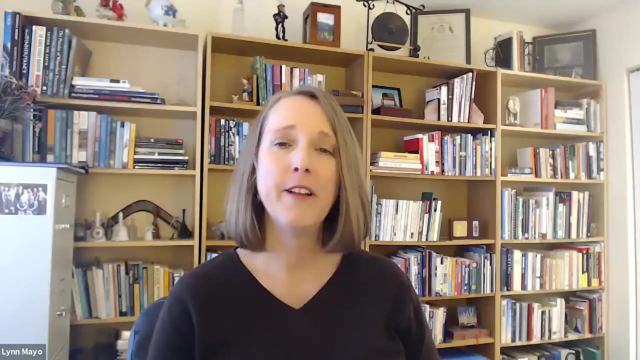 were providing them with all the information that they needed from the geotech engineers, kind of that. there was a good exchange of information just based off of us having some of the common knowledge of what each of the other disciplines was looking at. Yeah, that's a great point And that's really interesting, because not only you know. 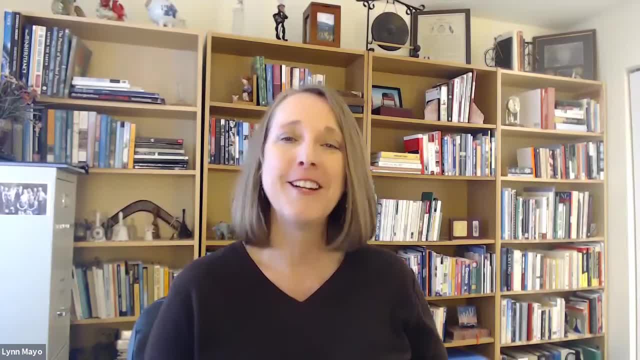 structures, water, all those things that maybe say, well, I'm not going to meet, I'm not going to get a job in that If you go into transportation engineering, you're going to need to know the water, you're going to need to know the construction management, all that. So that's a great, great point and 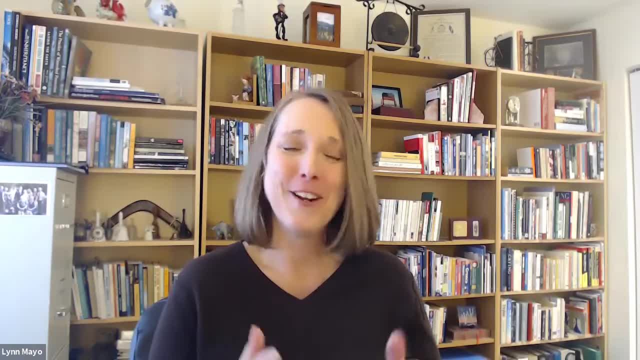 great motivation for people to pay attention to those classes, even if you're not going to be going to transportation engineering. So is there a certain software? if you want to go into transportation engineering, is there like a certain software or different softwares that you most have to use? you encourage? 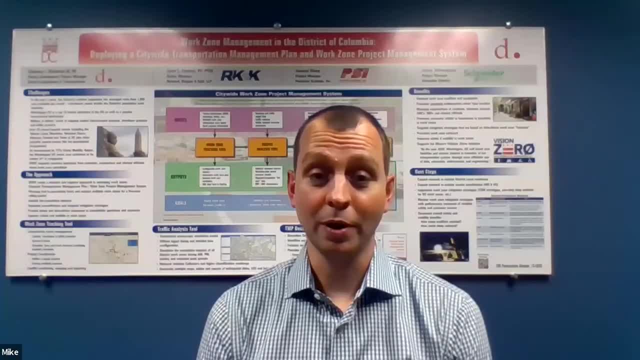 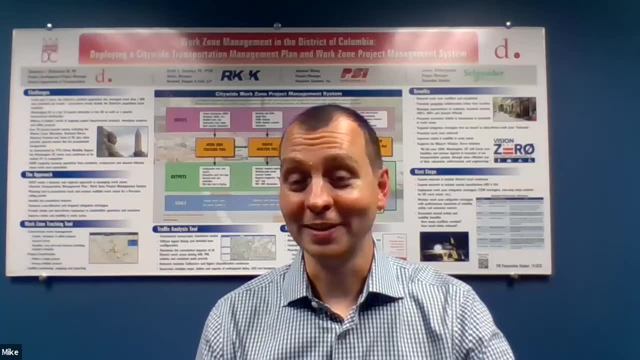 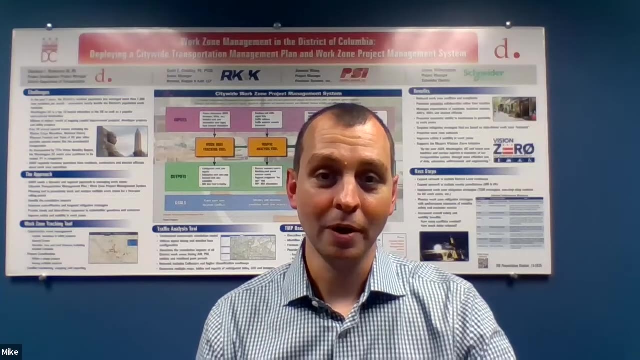 people to learn. Yes, Yes, So I know most civil engineering is done in, In AutoCAD. as far as a design software, That is not the case for transportation engineering. Most of transportation engineering ends up being done in MicroStation And then within. 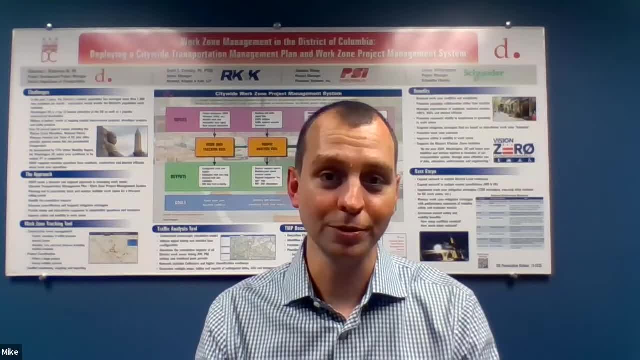 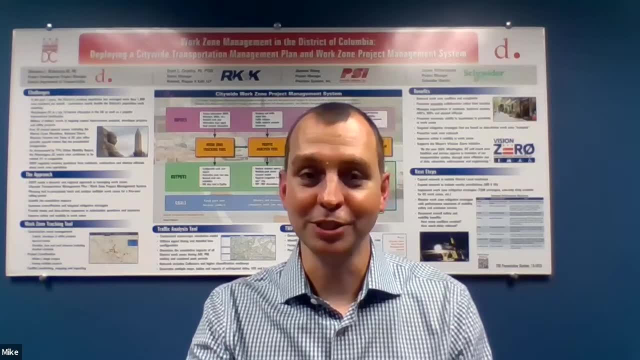 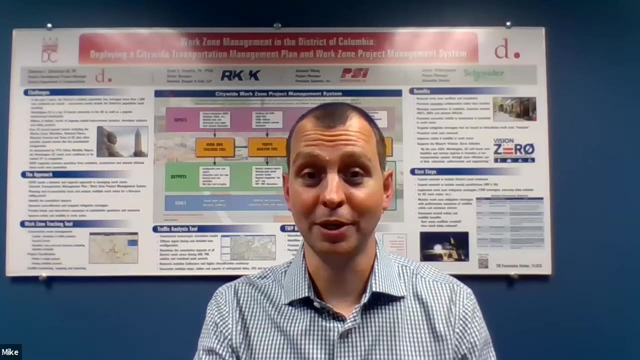 MicroStation. there's a 3D modeling platform called OpenRoads. That seems to be the new one that all the all the clients are moving towards. So those that would be my suggestion as far as roadway design software And then as far as 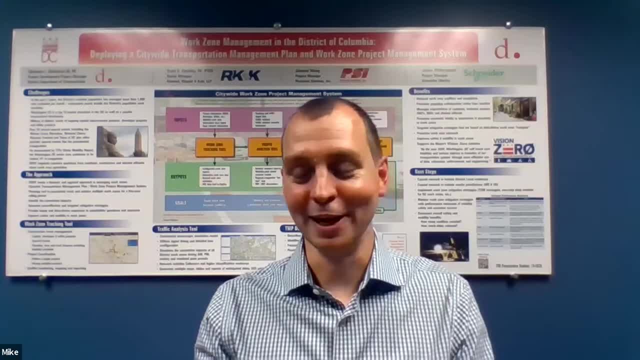 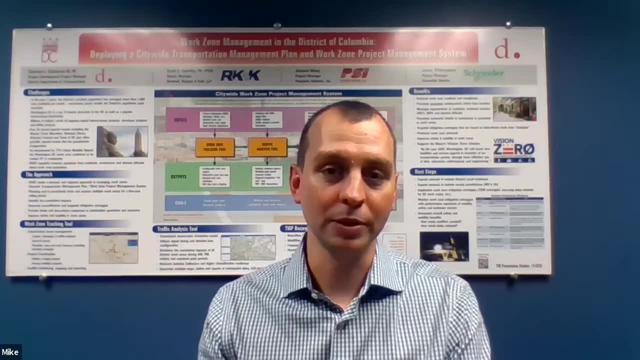 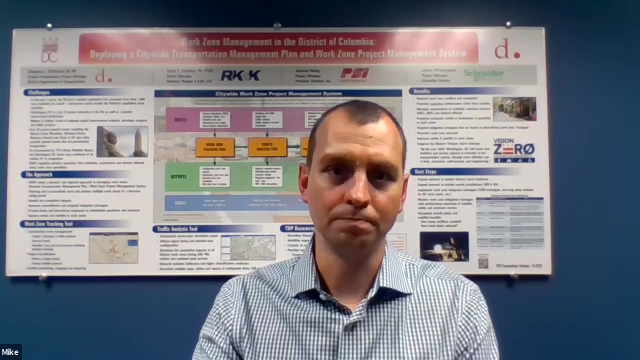 Not that I'll get too much into it, because I once again not a traffic engineer and don't want to get things wrong, but it does seem like there are. there's a number of different traffic modeling softwares, from Synchro to Vism, And so there's different models that 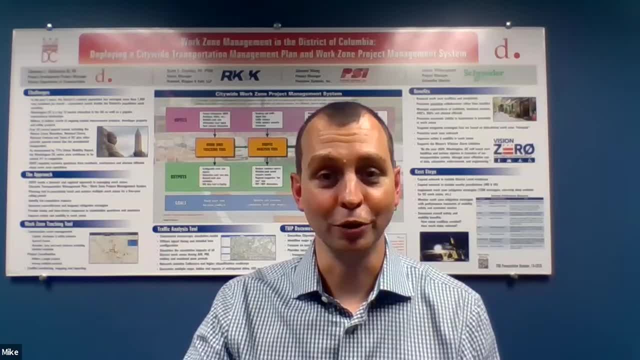 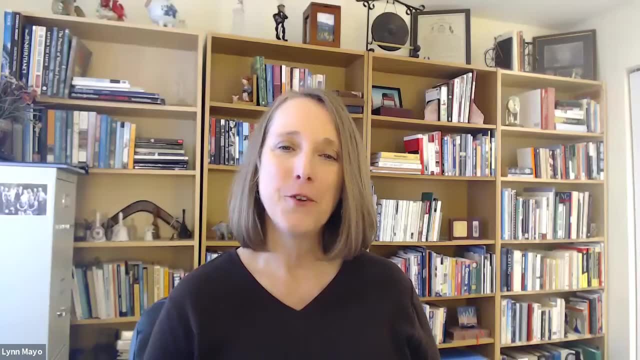 are out there that are. if you're going into traffic engineering, you'll end up needing to learn how to use those. Okay, great, And how about technical writing? Has that been a? Has that been important for your career? Technical writing, yes, has been very important. Almost any project that we do, we'll end up 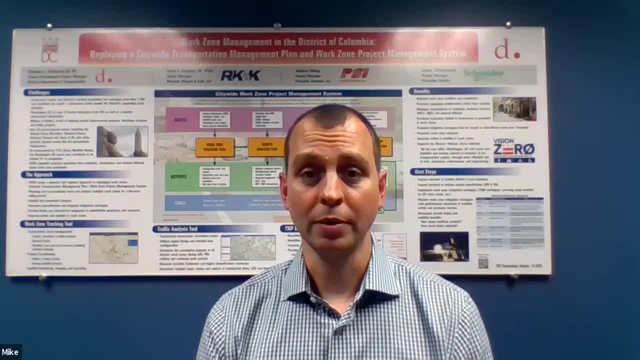 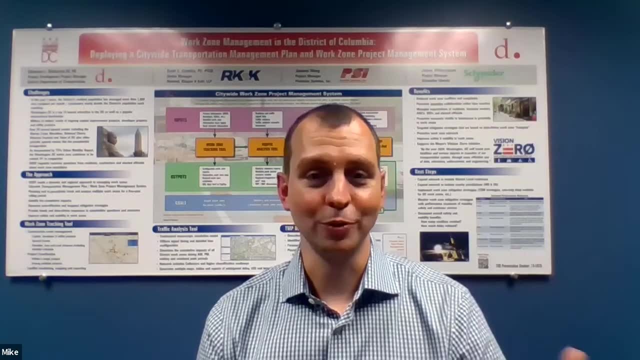 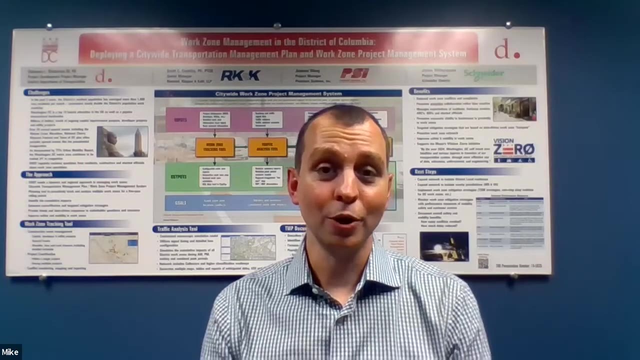 having technical memos that we'll be writing, whether it's to justify our designs, One of the projects that I'm actually working on right now. one of the things that I'm doing for it is writing design waivers and design exceptions, So it's a justification for the design that we are. 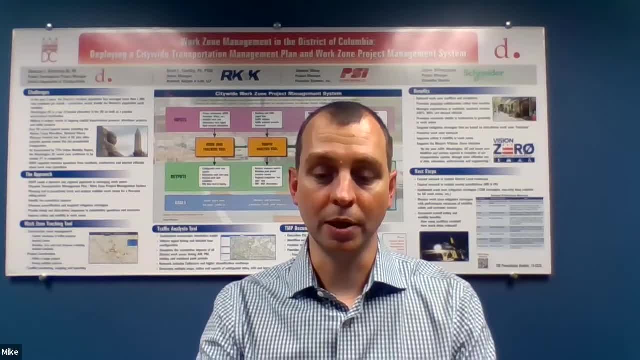 providing where we cannot meet the requirements for the design that we are providing. So it's a justification for the design that we are providing where we cannot meet the requirements for the design that we are providing where we cannot meet whatever the provided standards are. So we 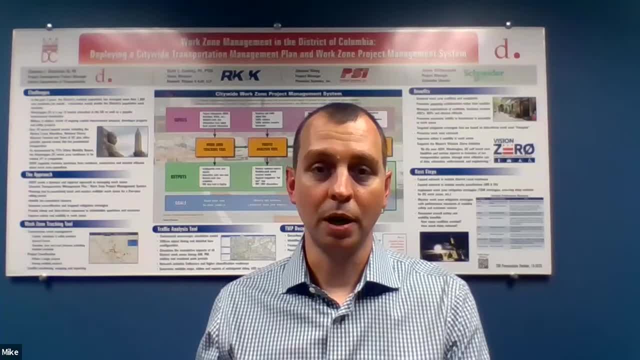 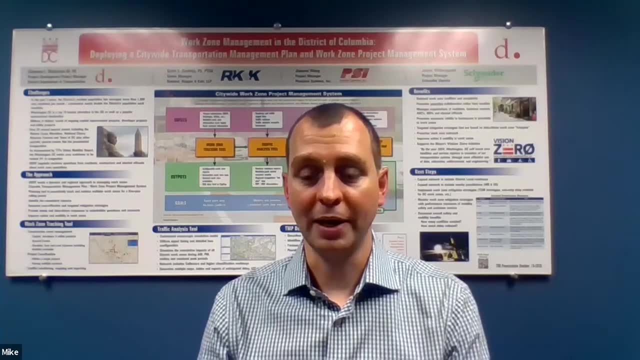 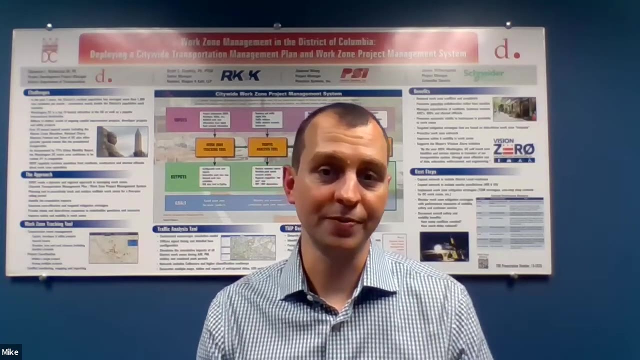 have to look at what the standard is And if we can't meet it due to some existing condition or some other requirement, we have to provide a technical memo laying out everything from how we went through the design process to the justifications for why we can't meet it to. 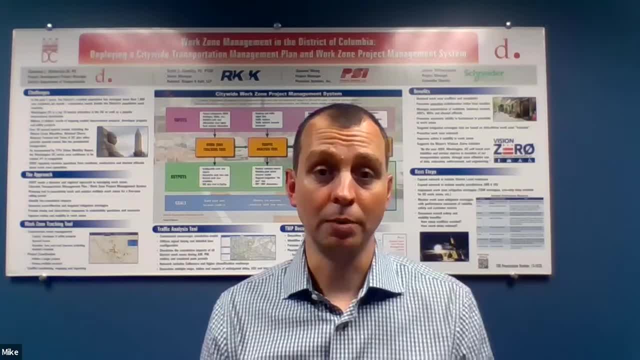 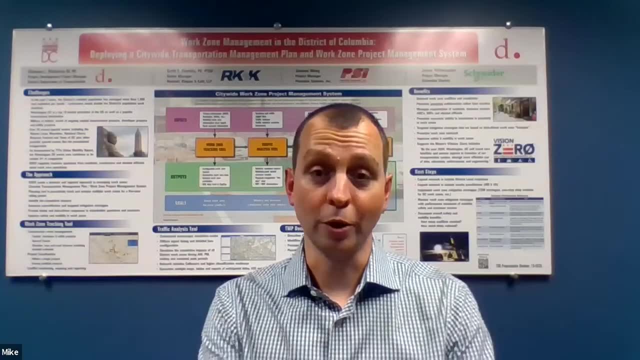 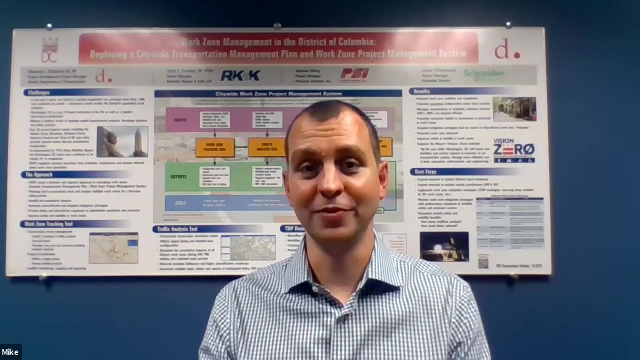 alternatives and then also how we can mitigate- mitigate any safety hazards that might be created from that. So it really is one of those where we are creating this technical memo, where our writing, our technical writing, and being persuasive through it, is very important in order to 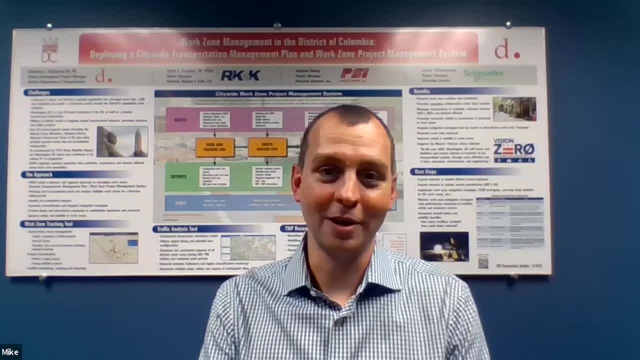 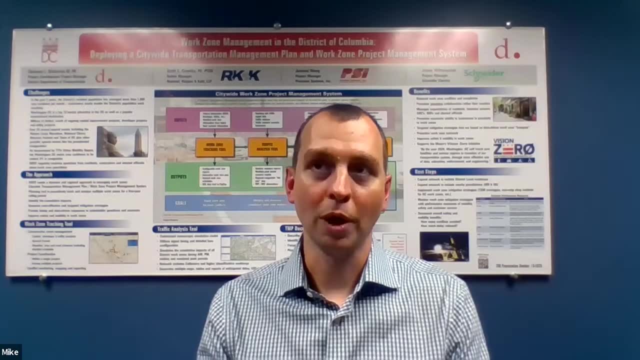 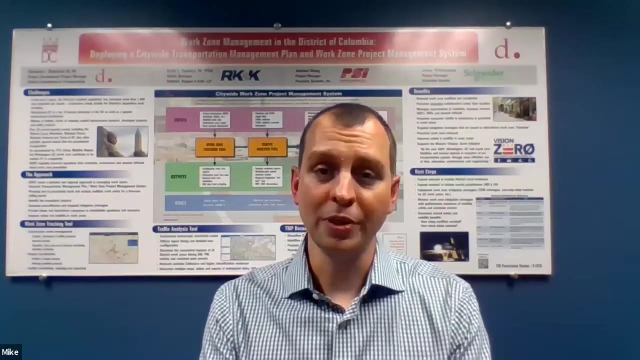 get them approved. So that's just one example A lot of our other projects. we do end up writing memos, whether it be recommendations or recommendations for things like safety improvements through a corridor or an analysis of different alternatives. So with each of those it's really important to have good writing. 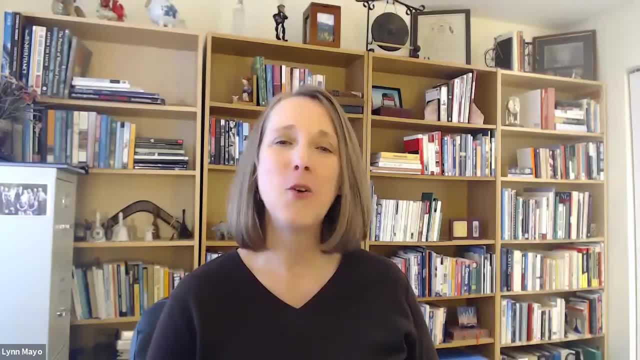 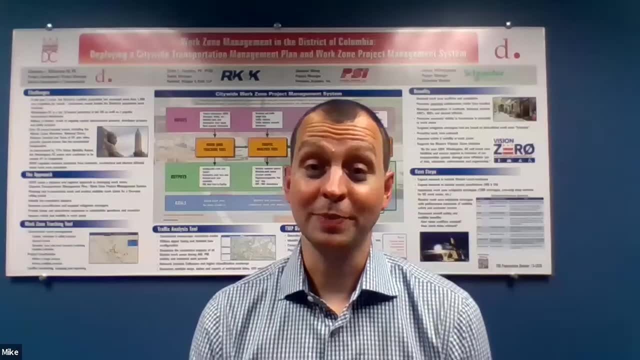 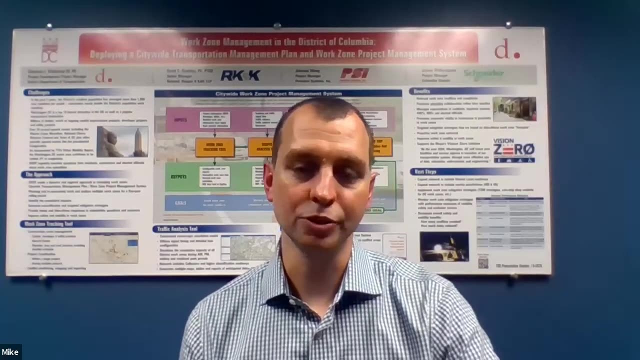 skills. So these writing skills are important. How about communication? as far as, like, public speaking, Have you had to do much of that in your career? Yes, public speaking is incredibly important, and it's one of those skills, too, that the more you advance in the industry, the more you end up using it. 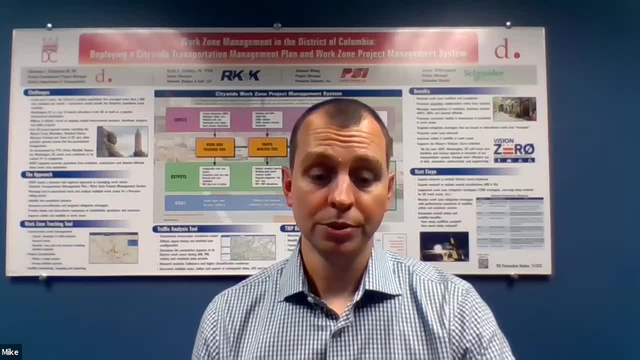 A lot of the time. it's a lot of the time. it's a lot of the time. it's a lot of a lot of the time. it's a lot of the time. it's a lot of the time. it's a lot of the work is one through quality based selection. So it's actually. we put in a 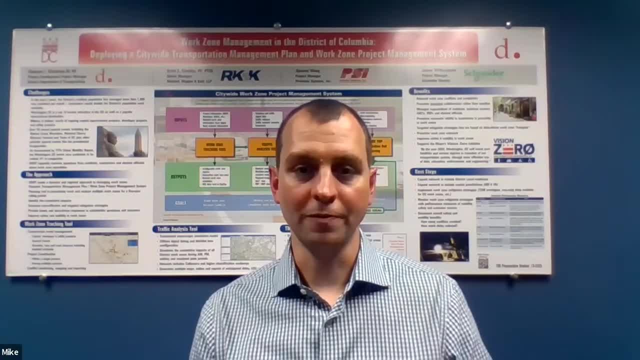 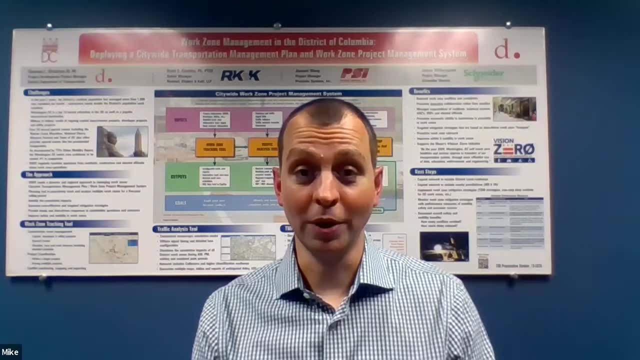 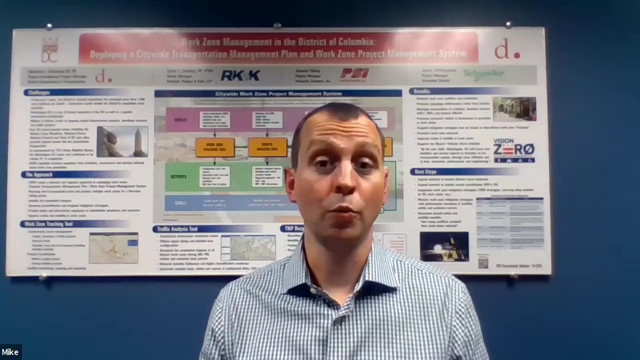 proposal that really lays out what our qualifications are. but then most clients bring us in to do an interview for that project. if we want to, if we want to win it, And so obviously we need to win it to then be able to work on that project. So with those we end up presenting in front of clients what our 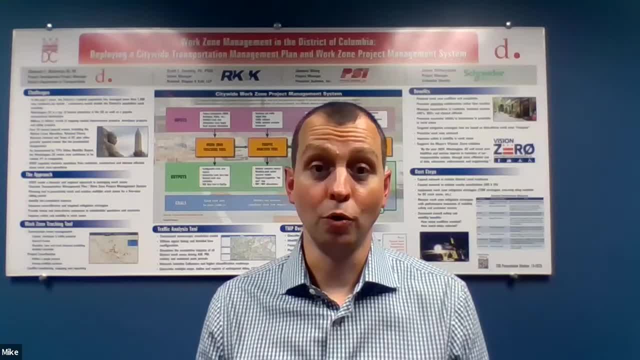 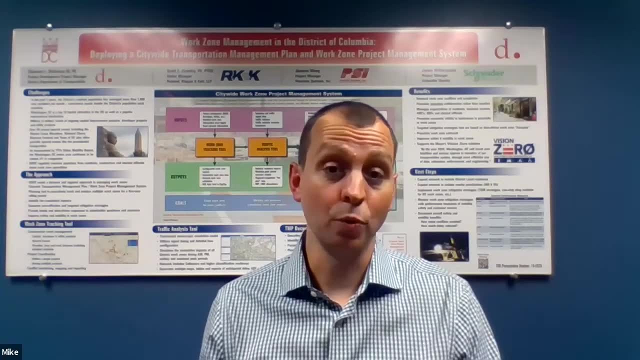 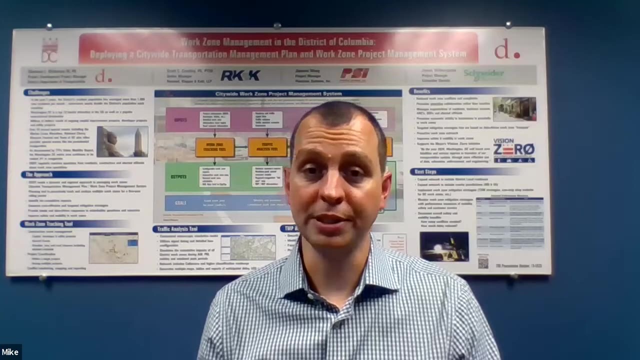 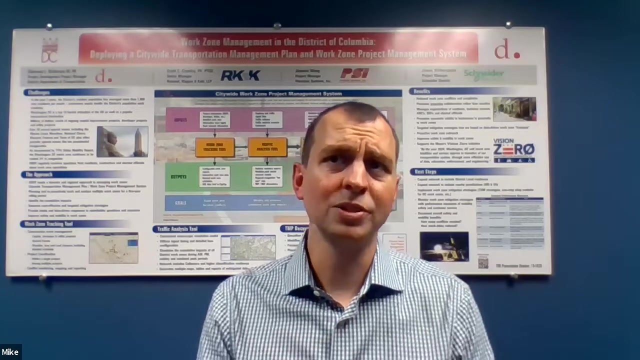 ideas are what our approach for the project is, And so public speaking, presenting to them is really important. And then also with our projects, most of them have a public outreach element to them, So we end up giving presentations to the public about the designs, about what will be happening about the designs. 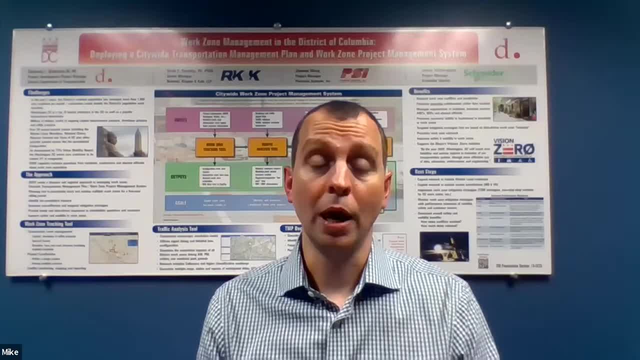 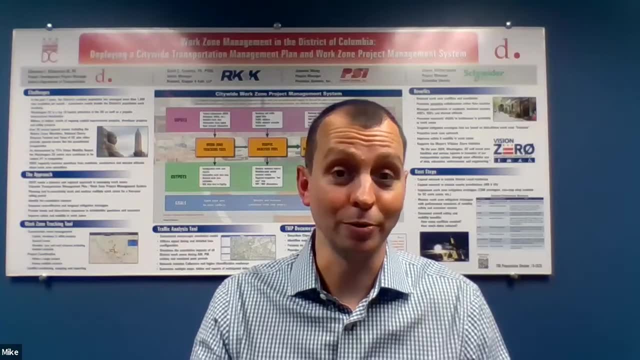 where have they being developed, what decisions we're making, how it's going to change a lot of times- the roadway that's in front of their house, or a roadway that they use right now Regularly, and then we'll have more updates again once we actually 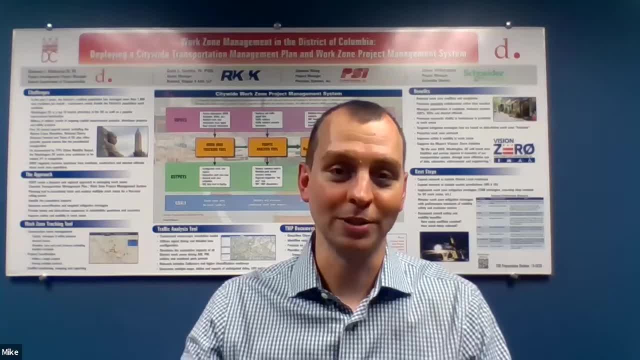 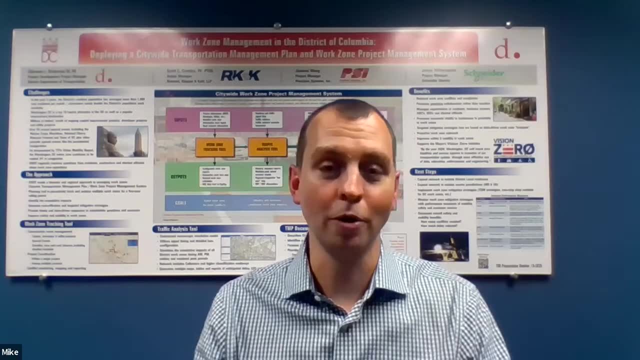 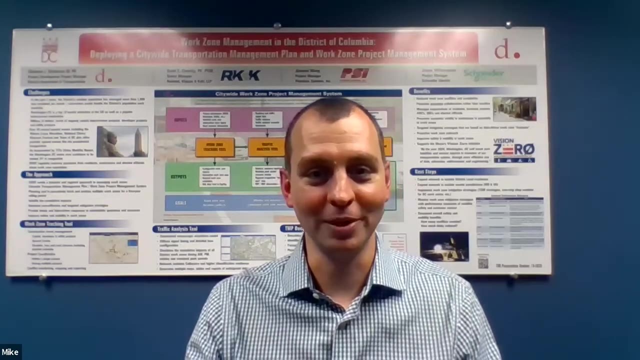 reach construction to keep the public aware of the progress of it, What to expect, especially if there's lane closures or anything like that. Just keep them aware of how things are progressing. really, just the more public outreach you do on those and the more informed the public is, the smoother your. 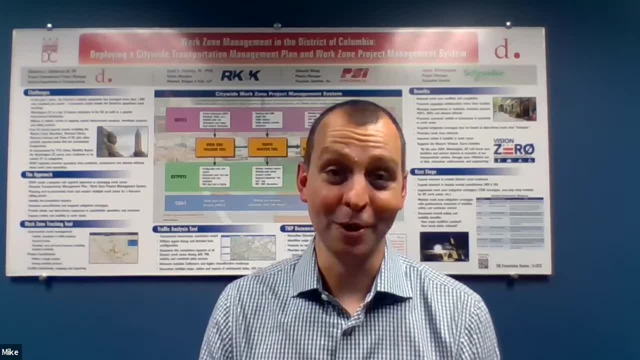 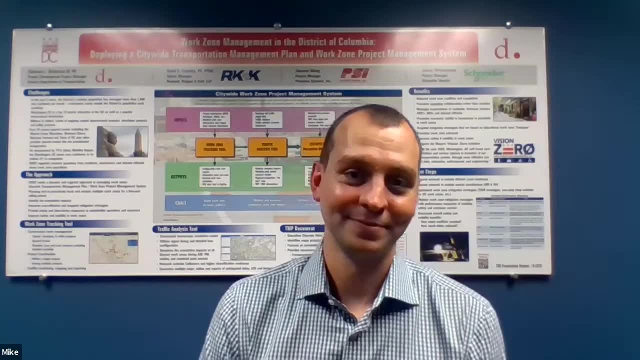 projects tend to go, So I hope you need to be able to present those to the public, to do public presenting for any of those instances. Yeah, so it sounds like. as an engineer, you need to be able to write, you need to do. 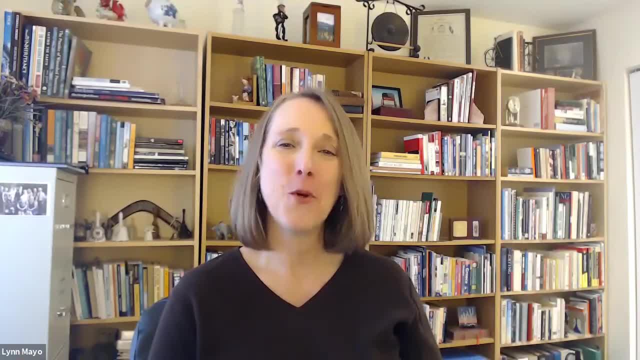 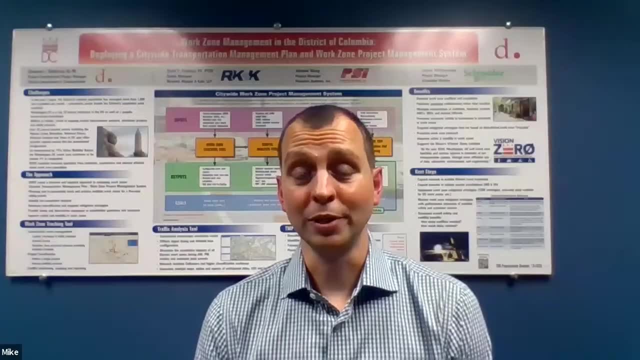 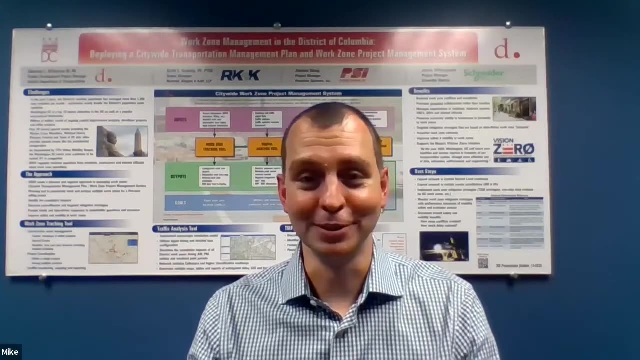 the presentation- obviously technical stuff- you have to have the software in some of the classes. Are there any other skills you think are important for a transportation engineer? I think the biggest one really is just problem solving With any of your projects and I know I've noticed this through. 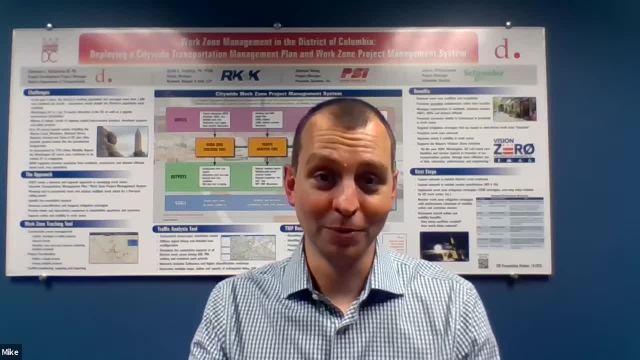 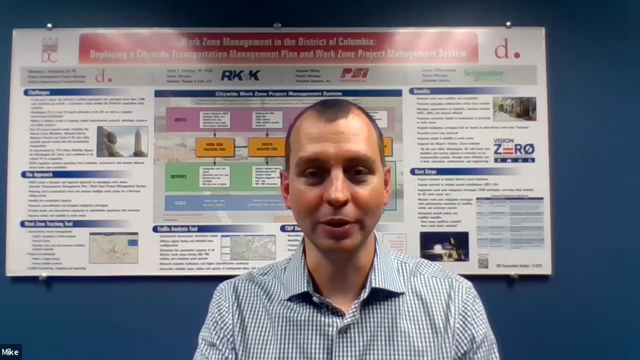 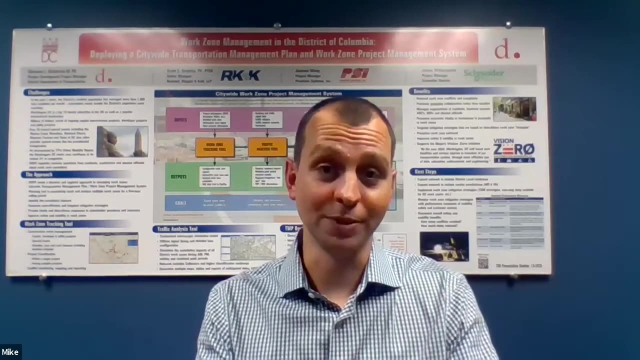 throughout my work history. you never know what's going to come up, So it's going to be something different on every project. that creates a new situation that you have to look at and really figure out how to best approach it and then come up with a solution or a number of solutions. 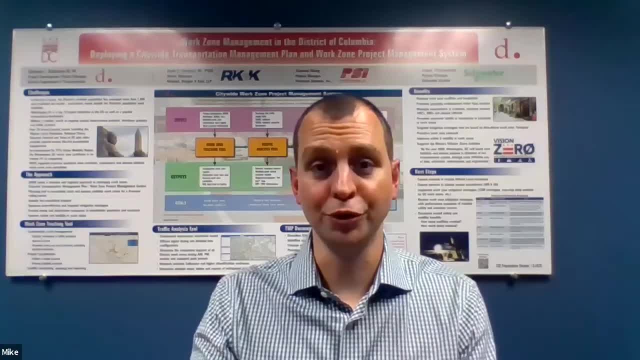 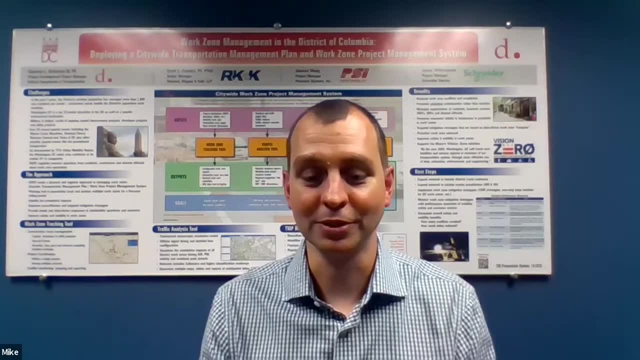 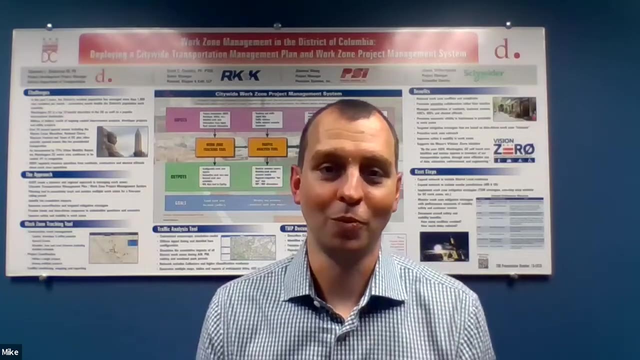 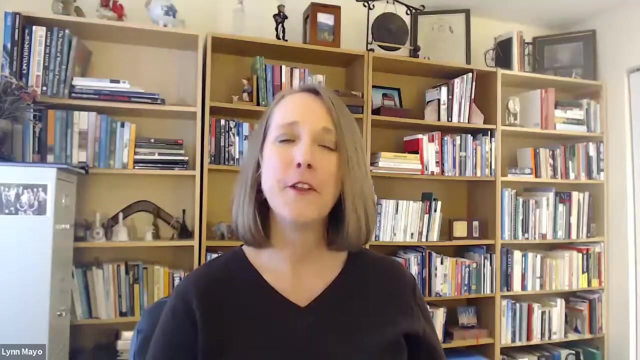 and then turn around and then communicate those to whoever the decision-making people are, to make sure that you get buy-in on whatever the best solution is. So it's kind of both problem solving and then commuting, communicating what the solutions are and what the trade-offs of each of them is. That's great and that's hopefully the 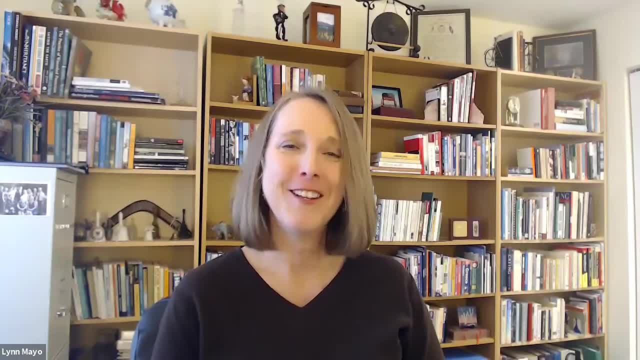 engineering education is helping them with those problem solving. We may not realize it, but getting those skills down. So if someone wanted to go into transportation engineering- and I know everyone's experiences are going to be different and every job will be different, but how important do you think it is? 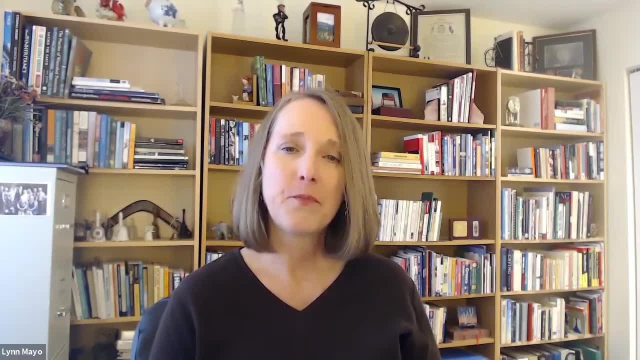 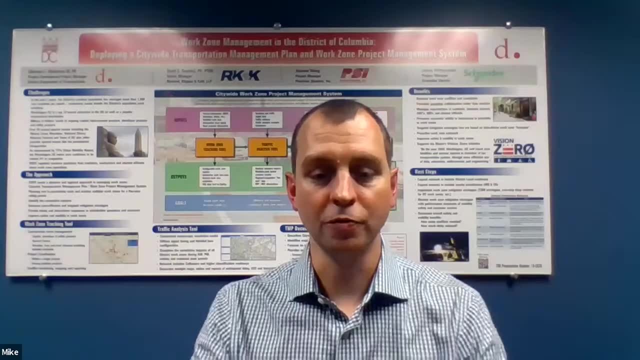 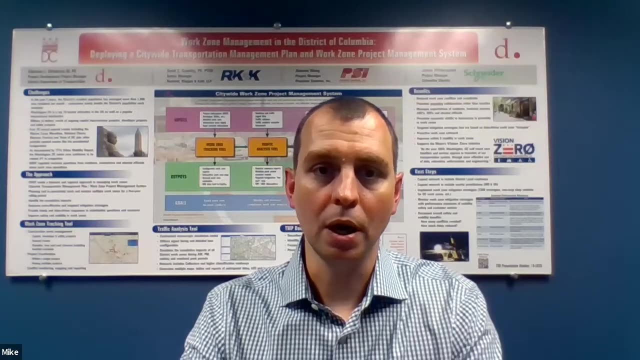 to have a master's in transportation engineering. It's a good question. So I think it really depends on the person and kind of what they're looking at. A lot of what I do from day to day is really applying what I learned in college. It's 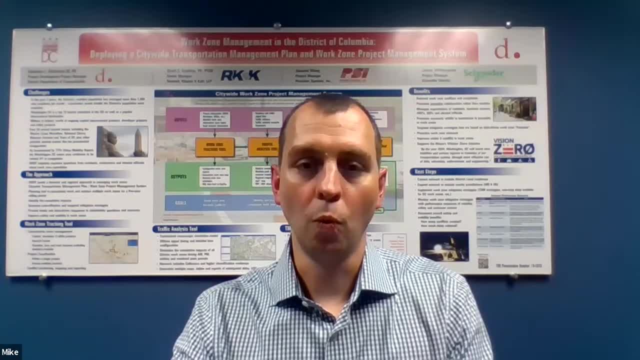 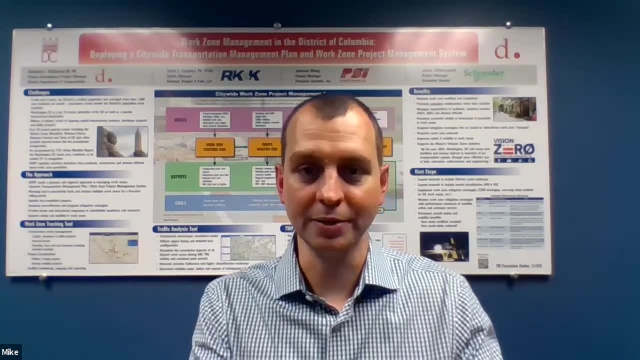 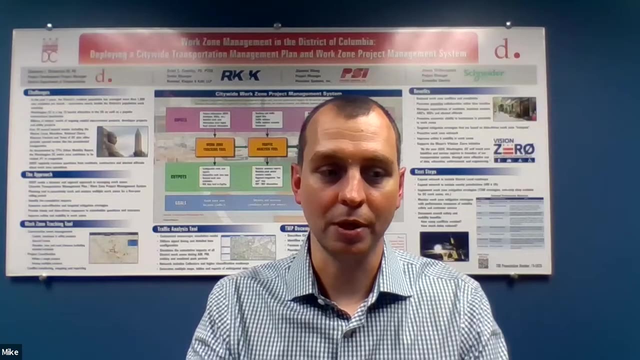 not necessarily looking at what the equations are or recalculating ways to do it. It's really just taking that equation and you apply it. But when I took my professional engineering exam, I noticed that a lot of the things that I did as far as 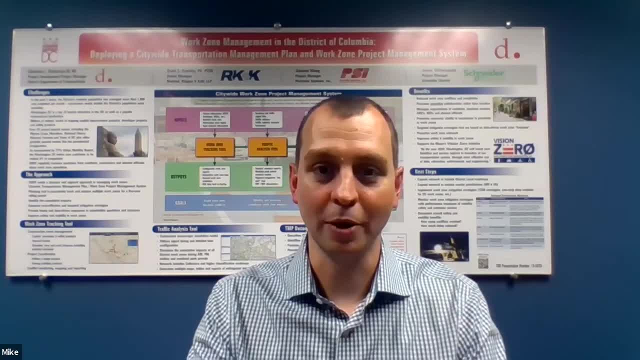 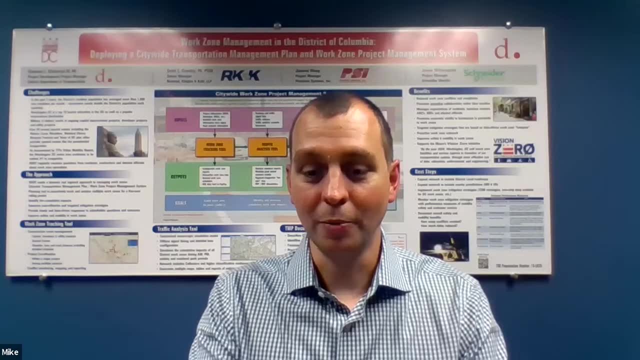 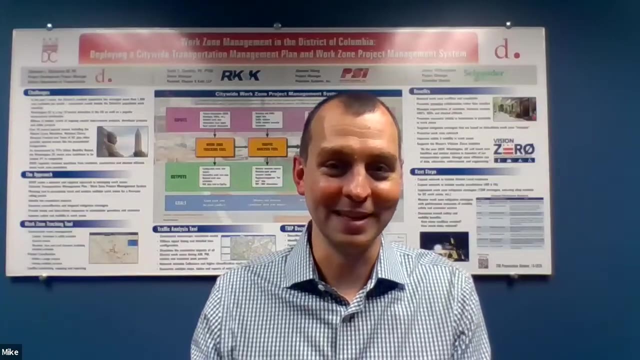 roadway design, where I was relying on our design software to just calculate things for me. I knew less of how it was actually calculated until I went to take that exam and was starting to study for it. So I actually learned a bunch from studying for that exam of about the theoretical behind what I 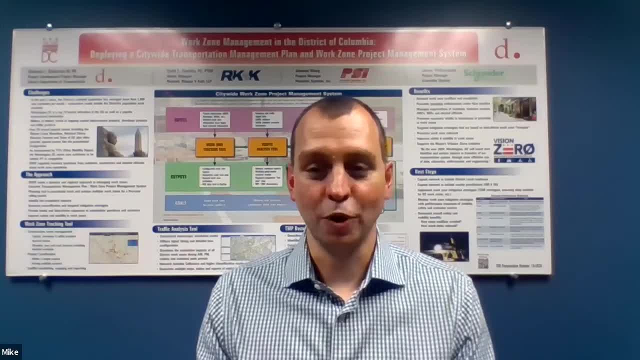 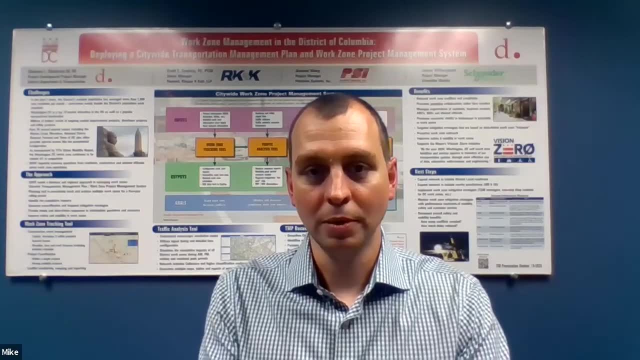 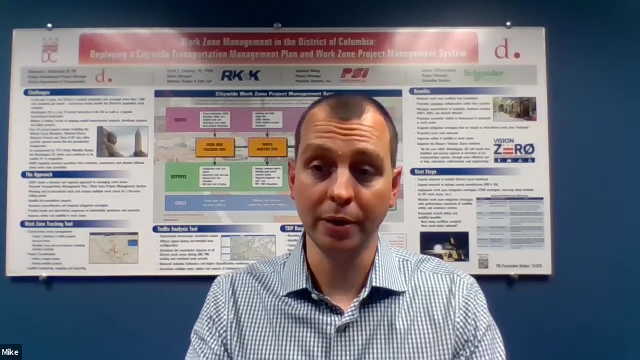 apply every day. So I think, as far as a master's and a master's, there is some of that where you will end up getting a little more into the theoretical and less into the way that it's applied, which can be very, very useful, And it definitely is showing. 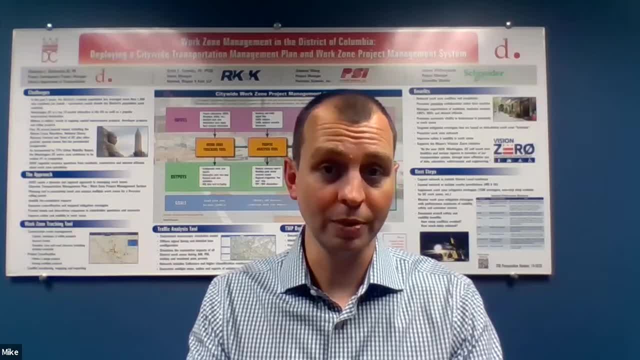 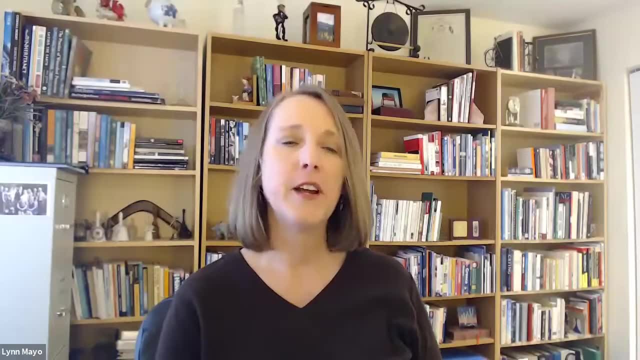 an interest in that area and you can become much more of an expert in that area. But I would also say that it's not necessarily needed. Yeah, that's a really interesting idea because I know what I've kind of seen as computers come more and more, you know. 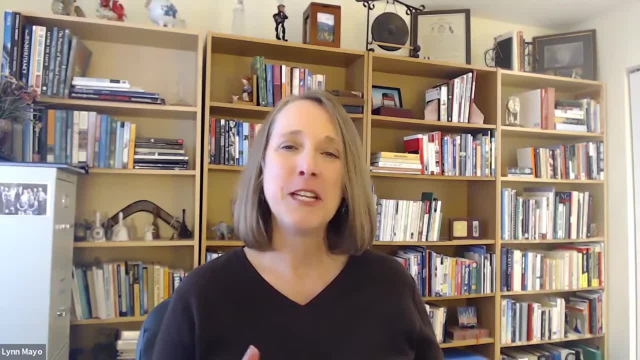 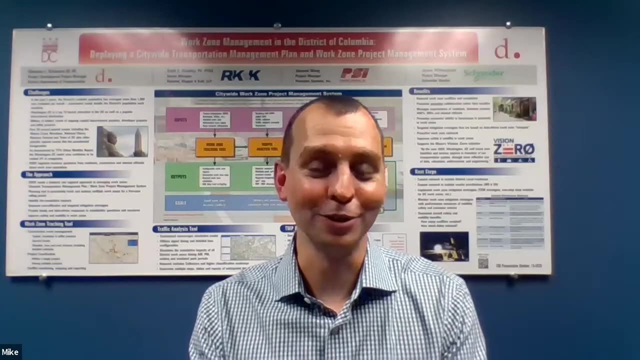 standardized and more elaborate when they can do. Sometimes it seems like less important to understand that theory until something goes wrong or there's some problem, and then to really understand that theory is really important. Yeah, I agree with that a lot. Most of the time, like I said, we're just applying things. 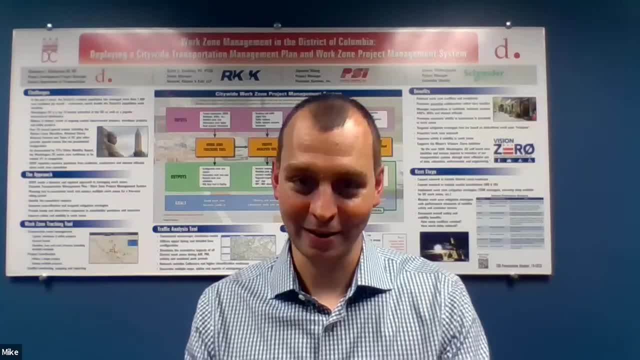 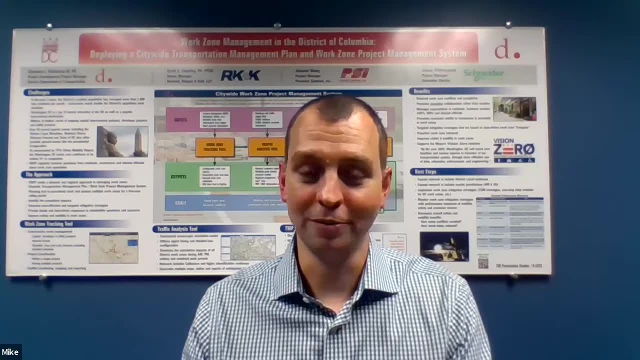 However, you also need the theory to be able to go back if something goes wrong, or even to just back check things to make sure that it is being applied correctly. I know a lot of people who are going through this number of times. I've gone through 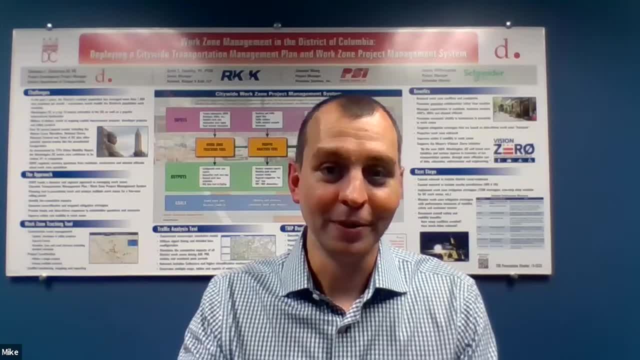 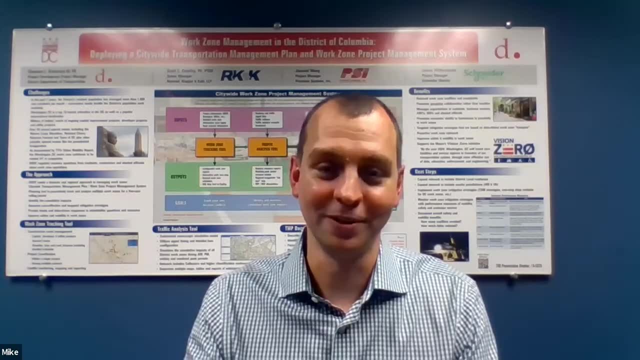 and we'll do a design and something just doesn't look right about it And, as a result, we'll go back through and do all the calculations by hand for that area just to confirm it, And oftentimes we find how something was being applied not quite correctly. 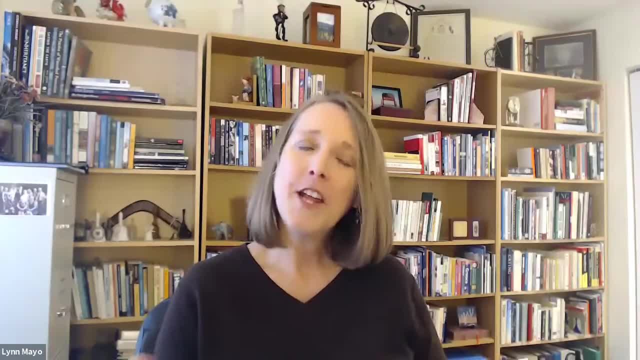 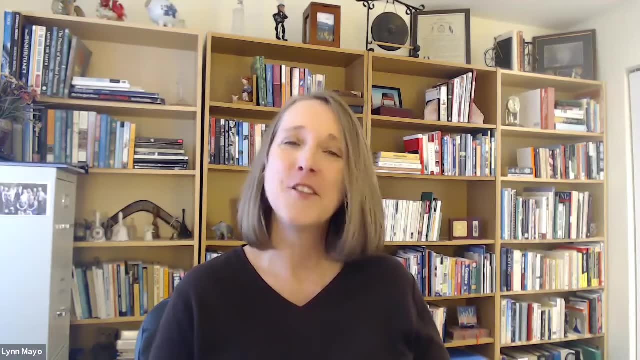 Yeah, interesting, That's really interesting. Now, you actually worked for about 10 years as a transportation engineer and then decided to get your MBA. So just curious: how did you decide to get your MBA and how that's helped you? Yeah, so getting an MBA was something that I'd 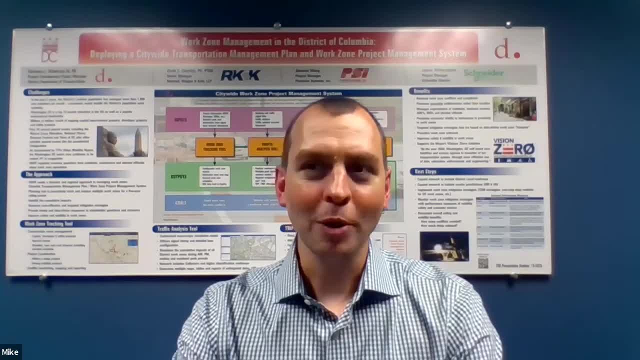 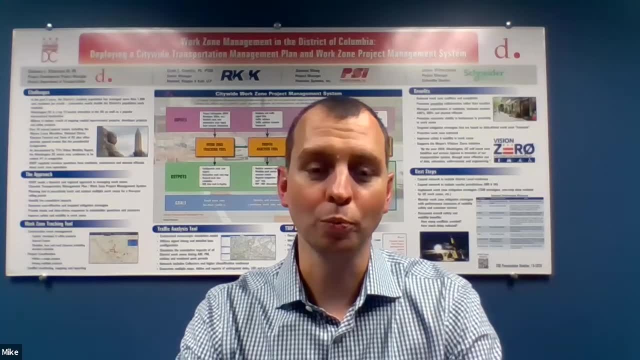 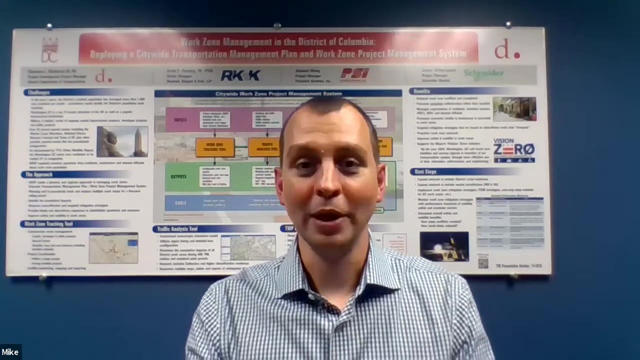 been interested in for a number of years. Actually, kind of probably coming out of college a couple years into my career, I kind of thought that it was something that I'd be interested in. I'm really interested in the business side of the industry As much as I enjoy doing the engineering and all I 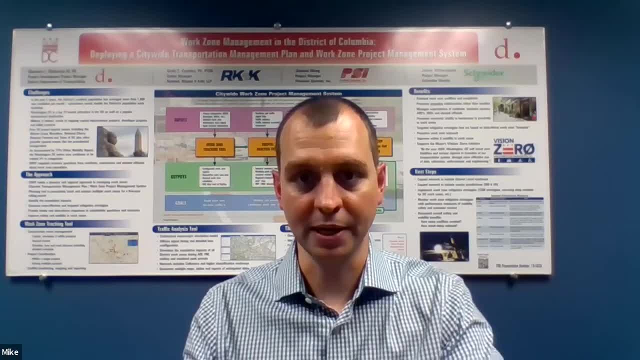 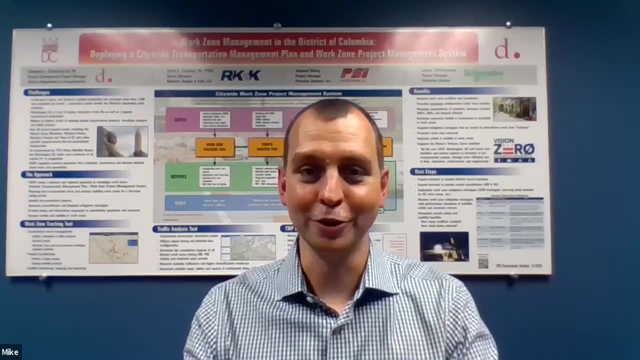 wanted to make sure that I had a really good fundamental understanding of the business side of the industry as well. So that was part of the interest for me, And then clearly I took a number of years before I really decided that that was the right move for me. 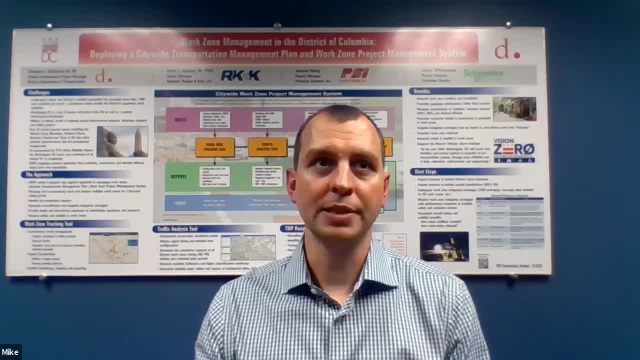 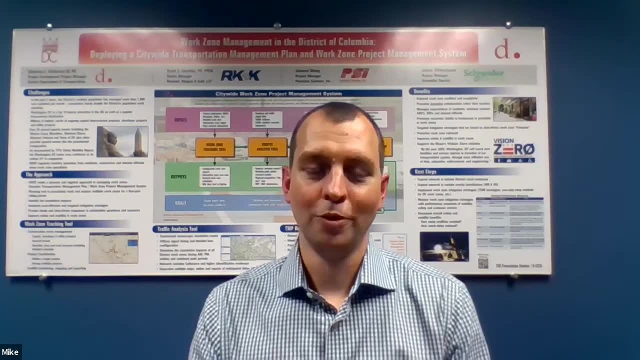 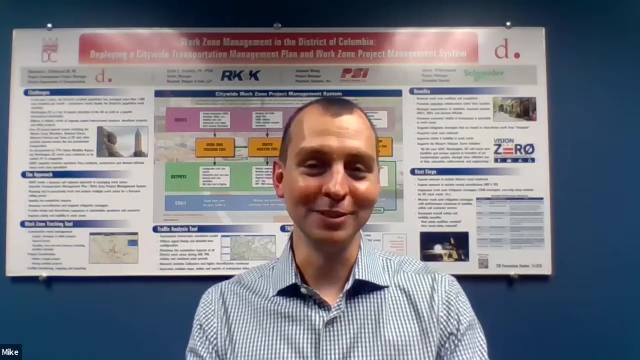 And as far as how it's been helping me, it really has given me a different viewpoint on some of the aspects of managing a project, From things like how important it is to get invoices out and kind of do some of the administrative things that are a little less. 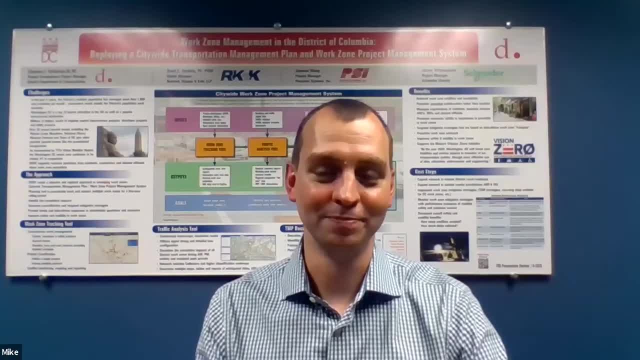 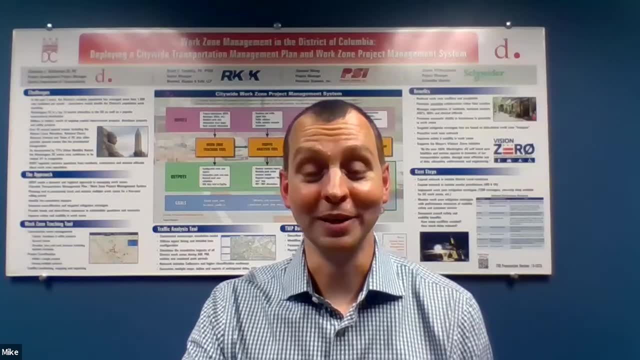 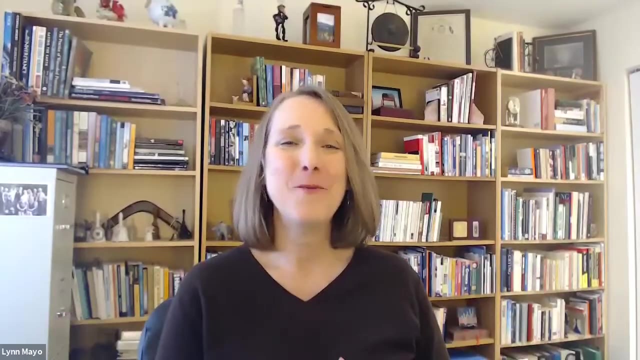 of delivering the project, but more for helping keep your company financially sound and really making sure that our company is financially sound and can be around to continue to help the clients, Which is important. right? We need to get paid for the work we're. 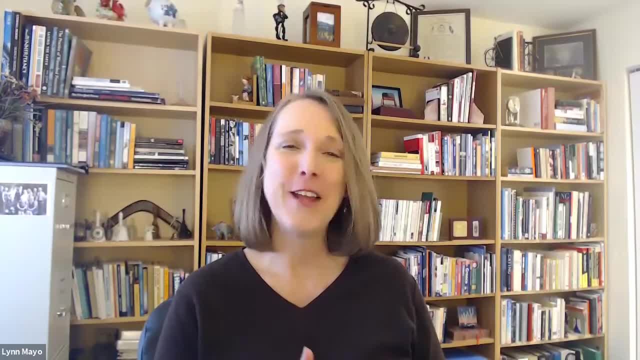 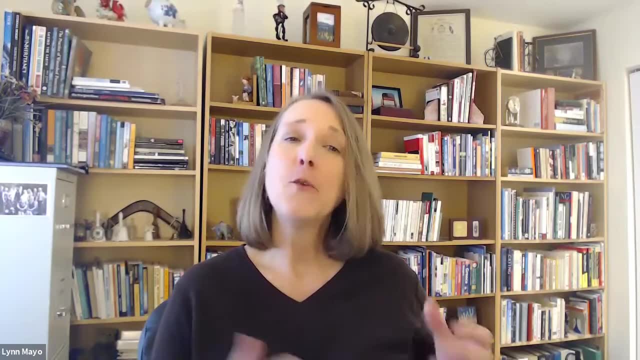 doing in order to continue. So that's great that you have really that mix of the technical as well as the business background. So someone say it was a civil engineer who's been working in a different field for a couple years and listening to you right now going that sounds really interesting. what? 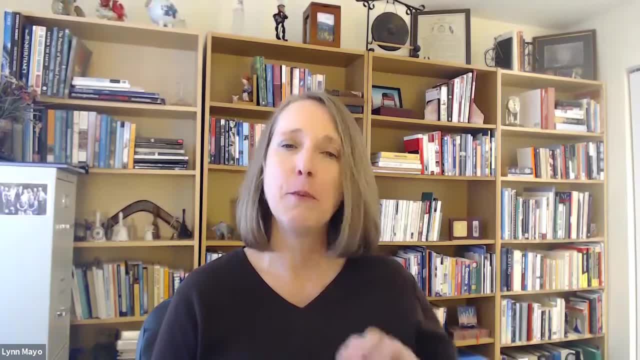 what you're doing and wanted to get into transportation engineer, but maybe they're in one of the other other fields. It would be easy to switch over and any recommendations of what they could do to maybe make that type of transition easier? So, yeah, I think it would be pretty easy to switch over. As I mentioned, most of our projects touch on almost every single one of the other aspects of civil engineering. As a result, you can I know from my past experience with our project- we pull in people from all the other disciplines at different times depending on what's happening on. 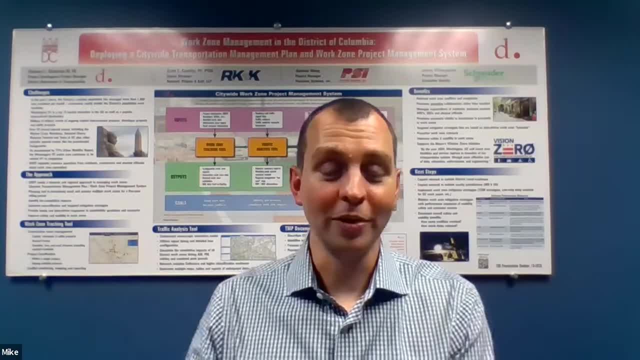 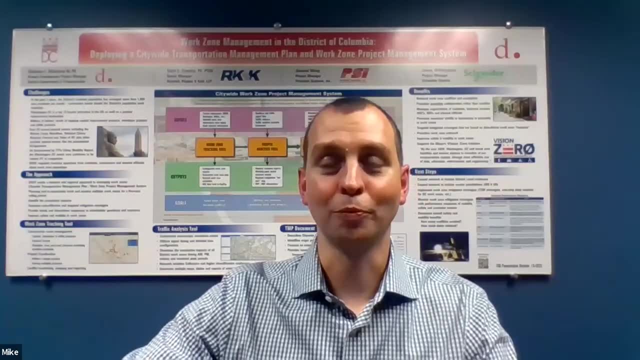 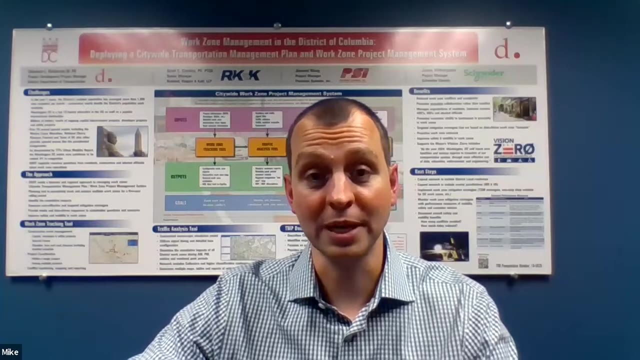 the project. So that is one way that you can start to make the transition would be if you can get involved in that as your aspect Or where your expertise is in one of the transportation projects would be an easy way to make a first step. 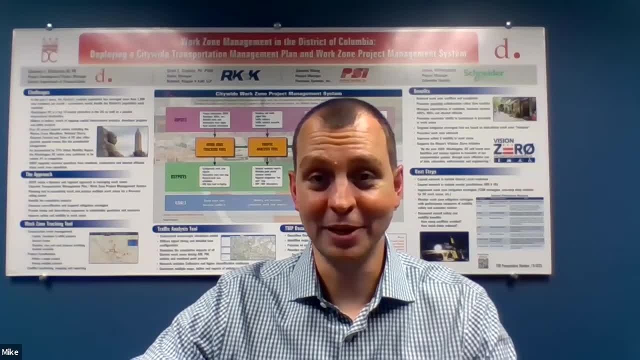 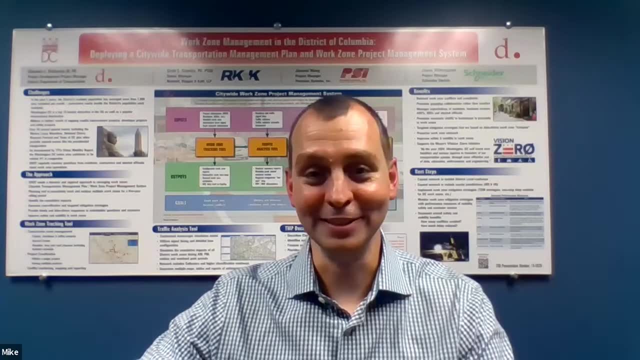 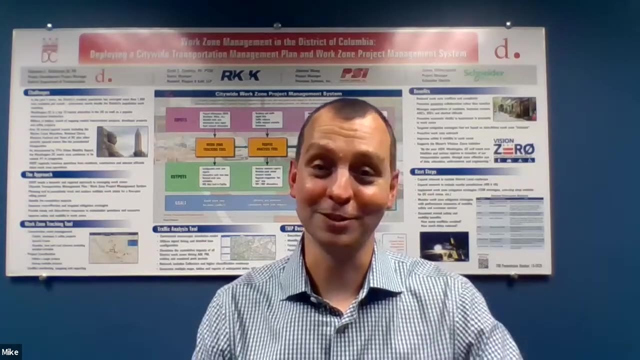 As I mentioned before, the software is a big thing, especially for roadway design. If you know MicroStation, it's very easy to teach the rest of it. So learn more or learn MicroStation. learn whatever software package is that you're seeing? 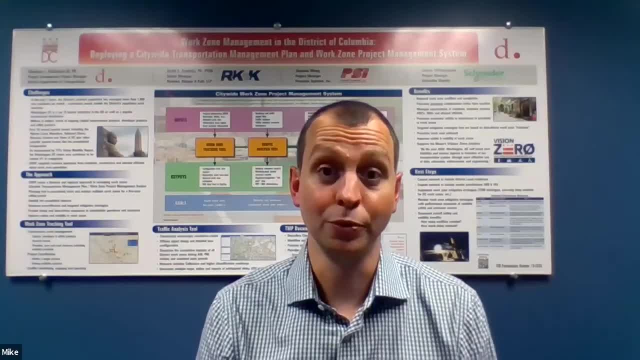 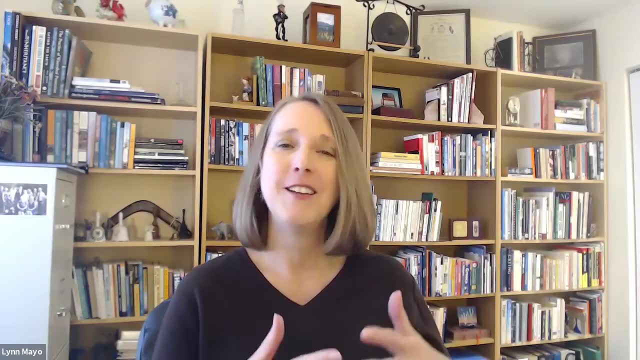 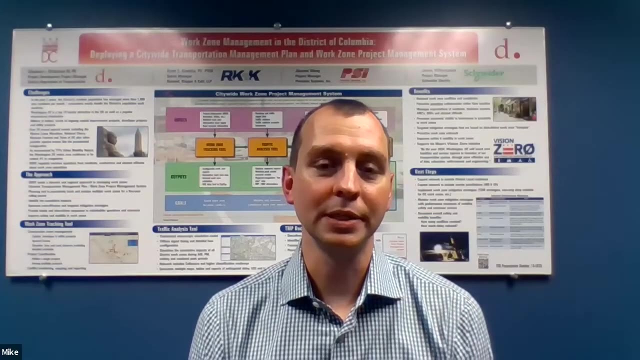 The transportation engineers in the field that you want to move into using. That's great advice. That's fantastic for people to, whether on their own or take a class, and that software it sounds like it makes it valuable for getting hired. Yeah, I think that that is one of those, that it's the 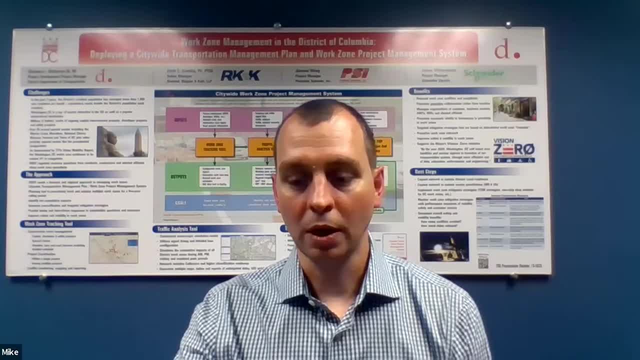 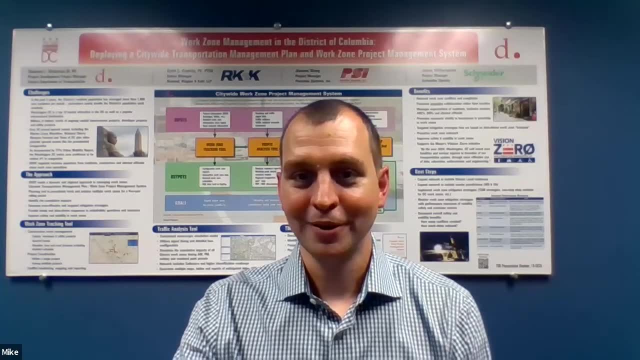 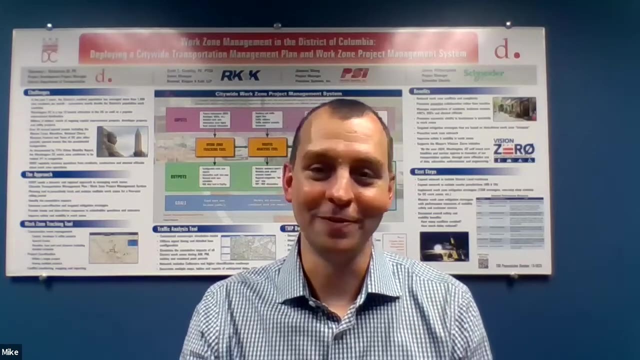 longest lead time. as far as teaching someone The technical side of things, as long as people have kind of the engineering mindset, it's pretty easy to teach those. There's manuals out there that I mean. we have our reference manuals, which are what we follow, and kind of a lot of them end up. 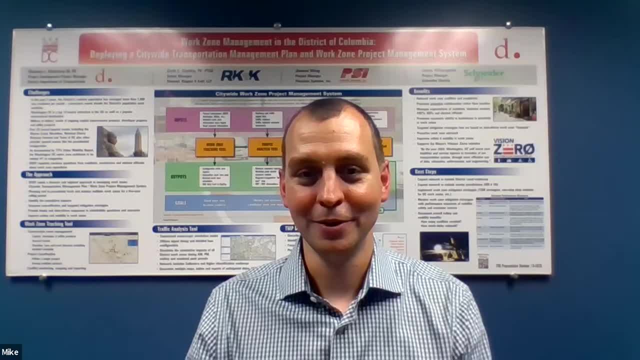 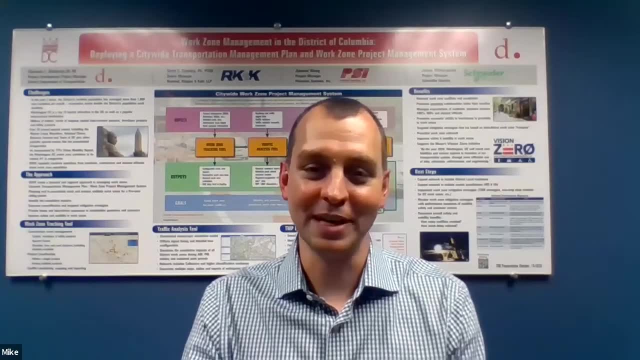 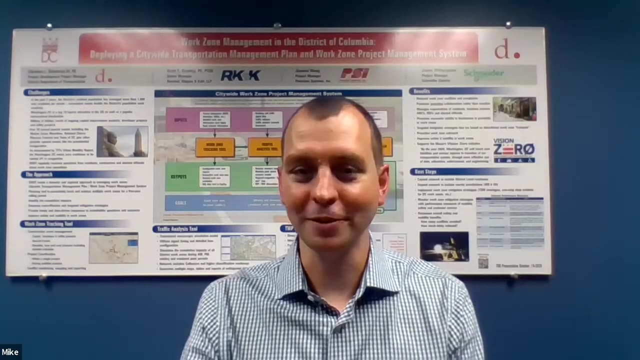 laying out kind of the steps through which we go through design. While there would be, for the software, similar manuals that lay out each of the steps and how you do them, it definitely is something that's a little harder. I feel like to learn from a book and much. 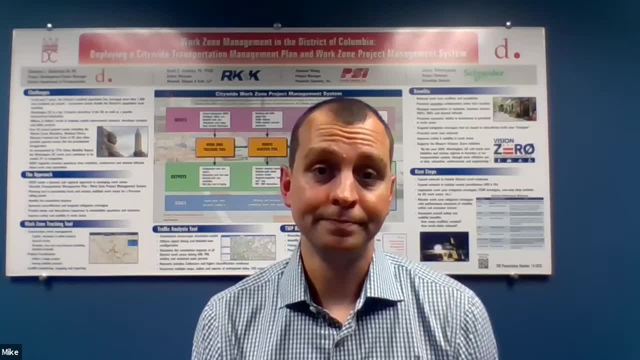 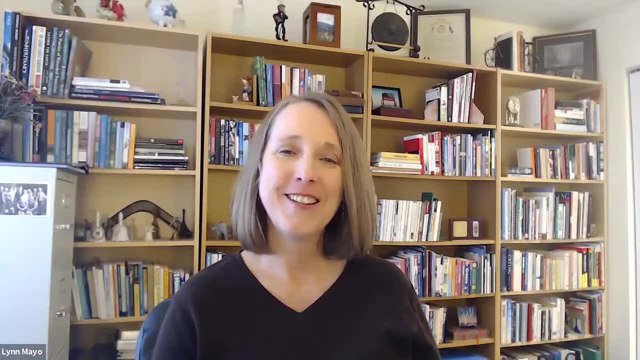 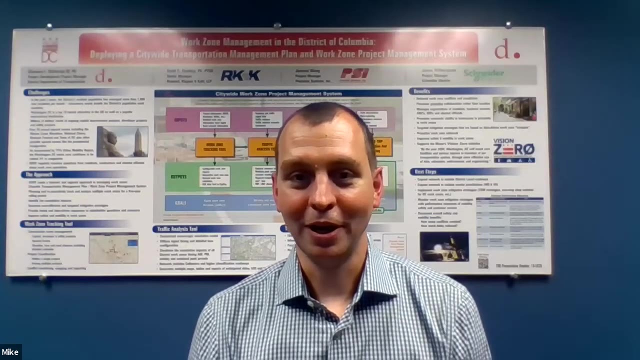 more that you learn from just doing it Interesting. That's great. So what do you think has been the best part about being a transportation engineer? So the best part that I find is really getting to see my projects built. That's kind of the most rewarding One of the things about transportation. 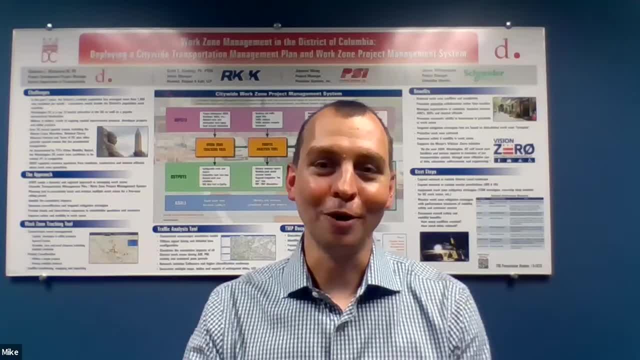 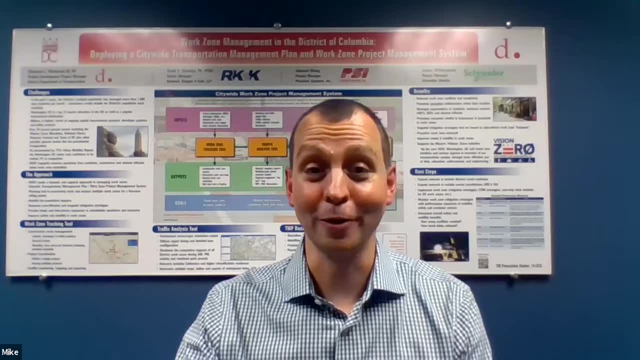 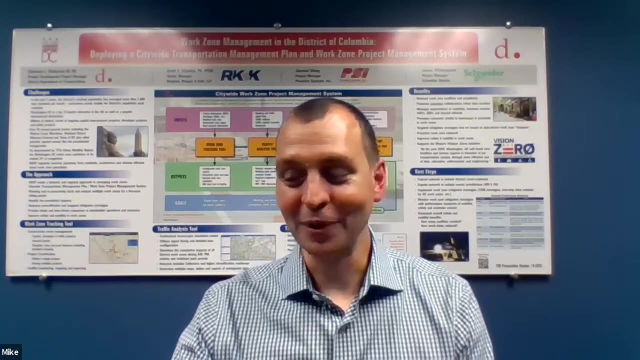 projects is a lot of them have very long, long life cycles. So I mean there's been projects- even that at the beginning of my career I worked on designing- that have still not been built, So that I mean it's been 12 years. some of them end up getting 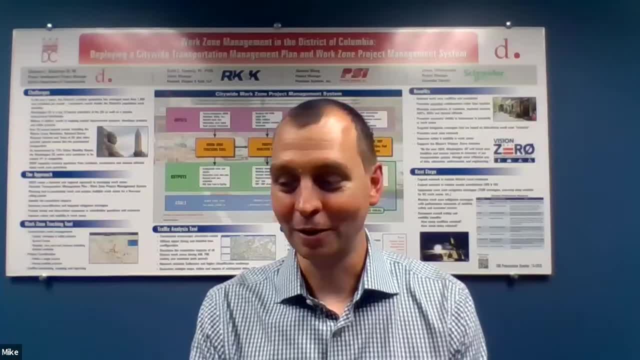 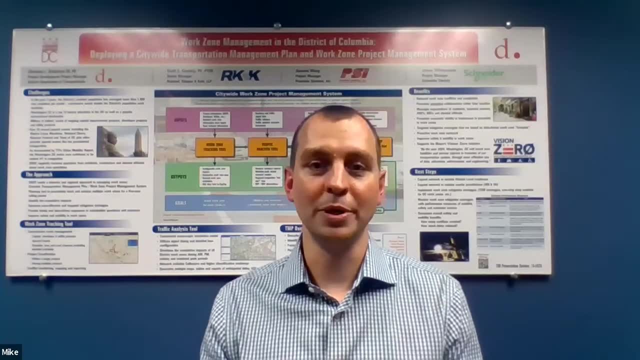 shelved or priorities change within the communities in between times, so sometimes they don't end up ever being built, But when you do have the ones that are built, it's really, really satisfying. So, as I mentioned with the wharf, 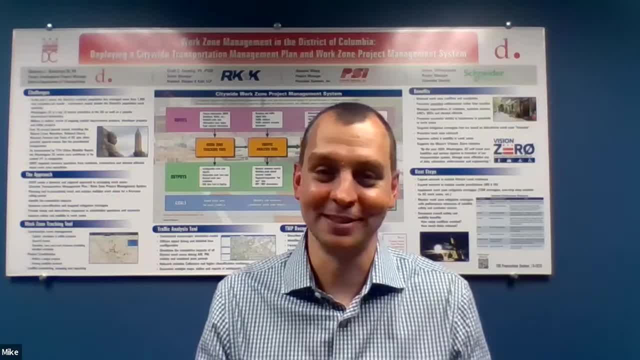 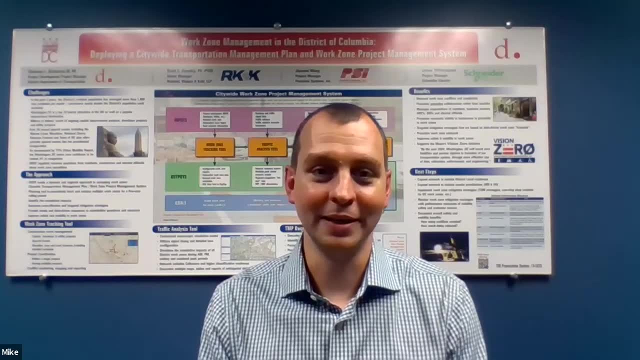 every time I drive through Main Avenue down there I just kind of feel a sense of pride. And then there's a number of other roadways around the area that I've worked on and it's always a nice reminder when I go through them of the challenges of that project. 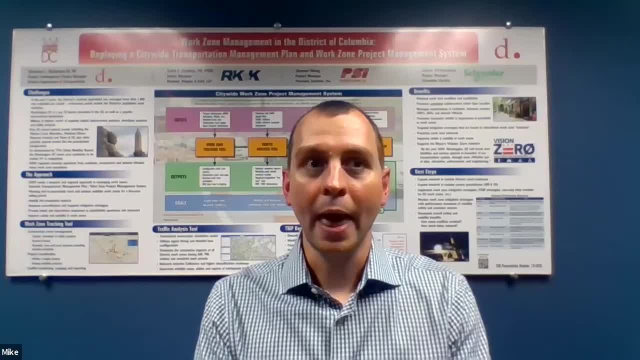 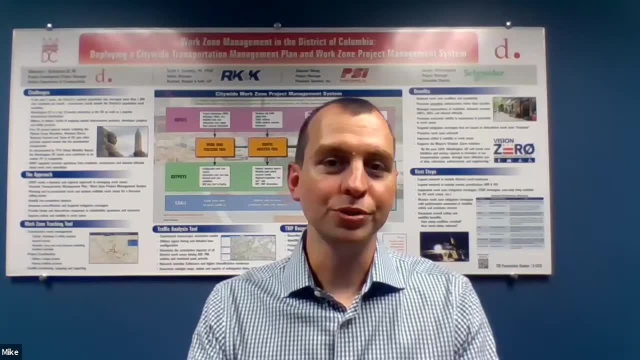 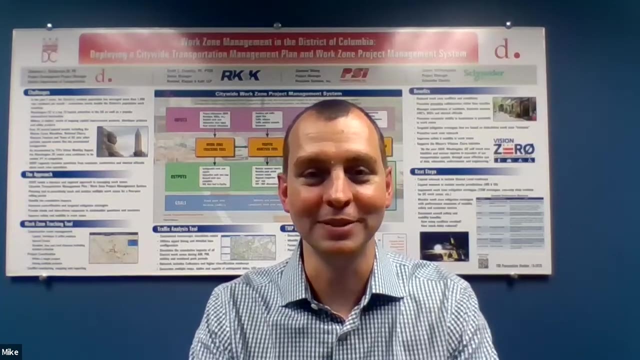 but also like the reward to really see it out there and how our projects have kind of changed what the community around them, kind of how they use the road, how they use the sidewalks, all of that, but also kind of the look and feel of the neighborhoods, how they can change. 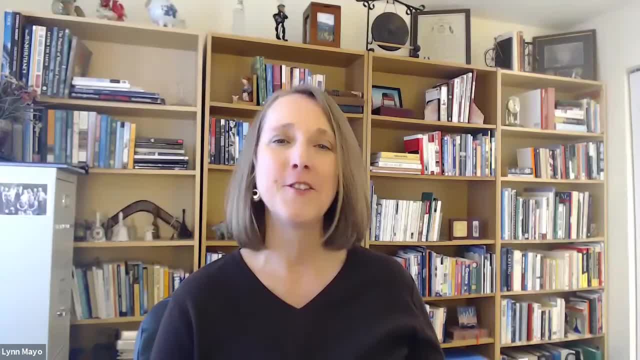 Yeah, Yeah, it must be a really good sense of fulfillment to kind of see that you're impacting, positively impacting communities and you can actually see that change. Oh yeah, absolutely. It's kind of amazing- and one of those too- that when you're looking at 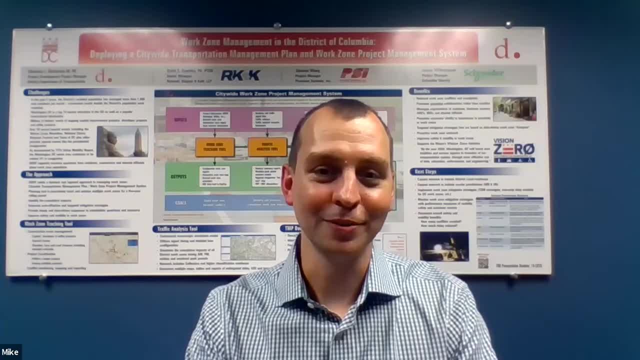 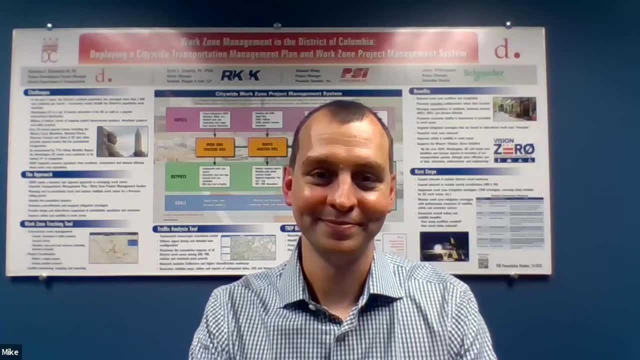 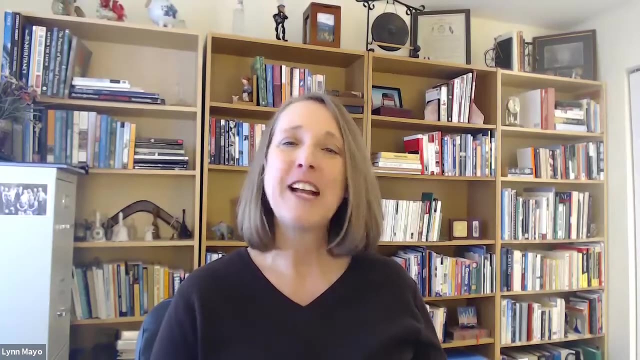 plans all day. sometimes you don't notice how much that when this is implemented, it really will change how things are out there. Yeah, So this is going to be a hard question probably to answer. but what type of person do you think would actually thrive and be happy and succeed? 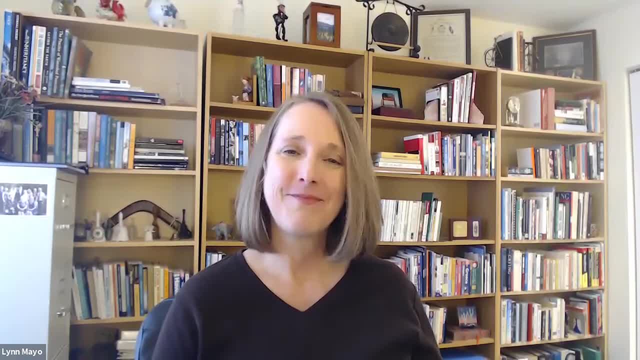 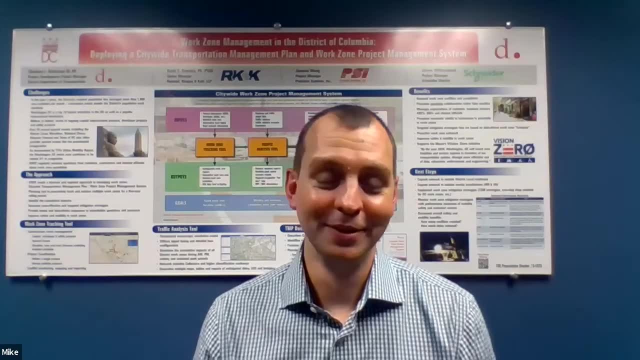 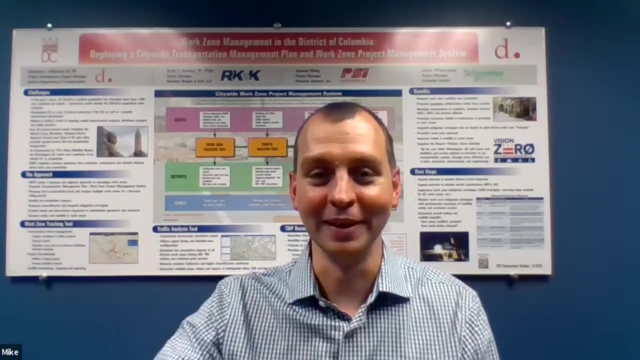 in transportation engineering. So, as I mentioned before, I think the biggest thing is having a love of problem solving. It is just thing after thing that you look at. No design is simple. Nothing is just. you can cookie cutter everything, just drop in the same design here, there and everywhere- Every. 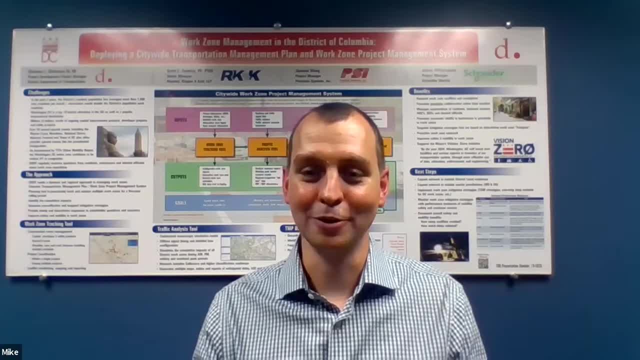 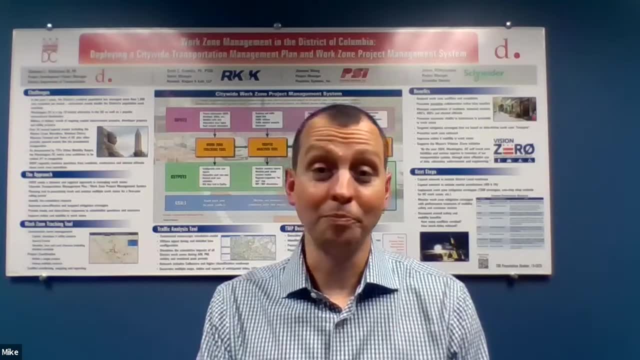 road is different. You really have to look at it and take a step back and think things through. So it's, and then, as I mentioned, solve each problem as they come up. Some of the longer lead times on projects, as I mentioned, so you have to have some patience with. 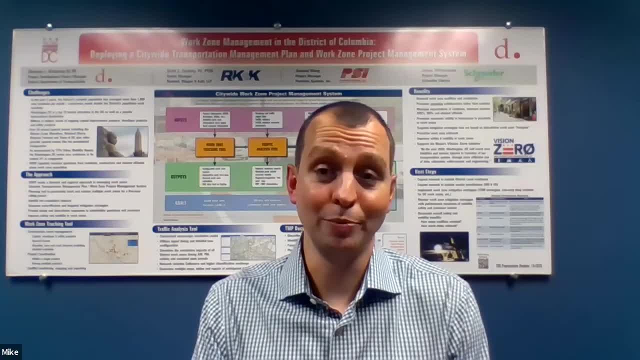 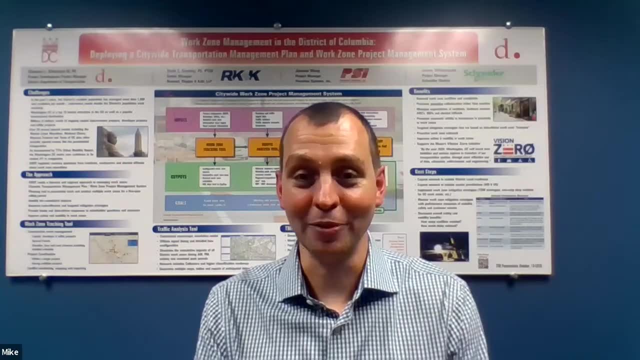 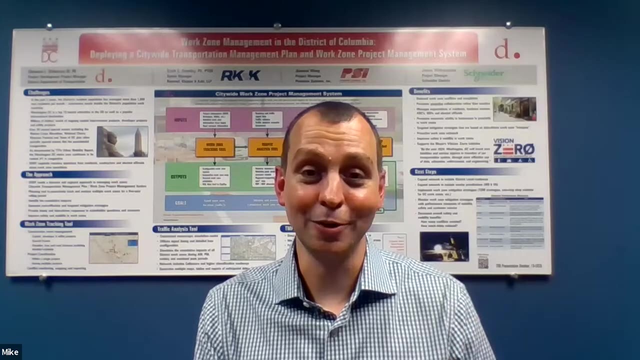 those, but then also you'll have other projects that are going to move more quickly than you can imagine. especially, there's different project delivery systems that are out there now, including design-build projects. So design-build projects are really simple projects where we team with a contractor. 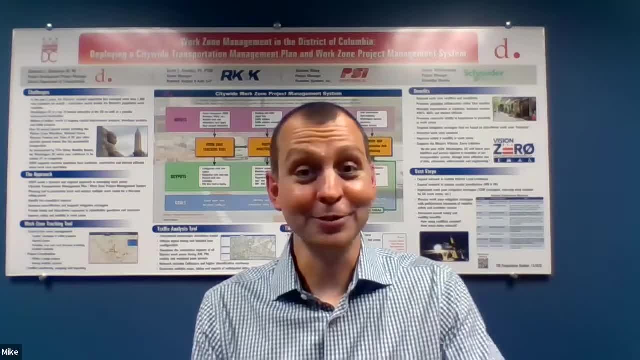 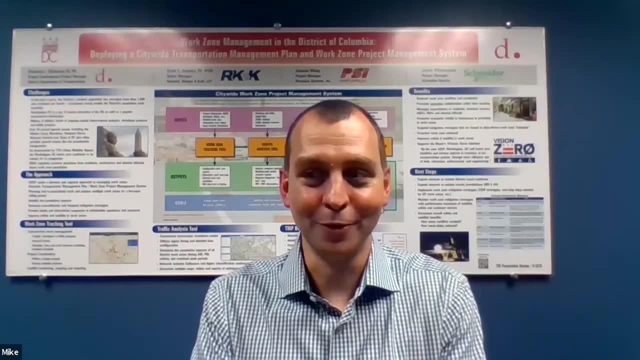 and, as a result, we are designing it and as soon as we're done with our design they're out there building it. So some of those projects really just push the timeline. It's shorter, it's high pressure, but also kind of enjoyable because you get to see the results of. 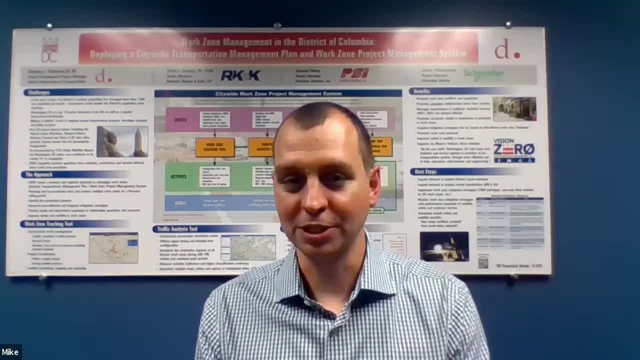 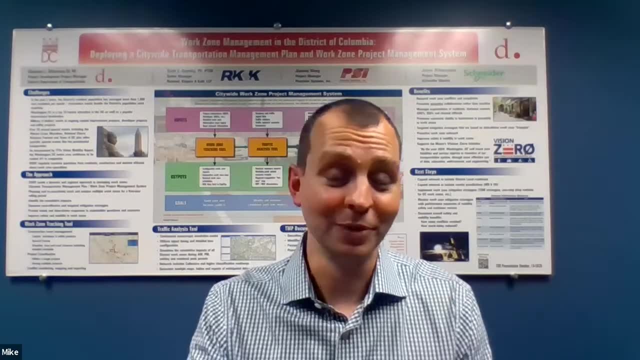 your work even faster. So I think you have to be flexible from project to project as well. but you're going to have some that we're going to move really quickly, some that'll take their time. So you just have to kind of be ready for anything. 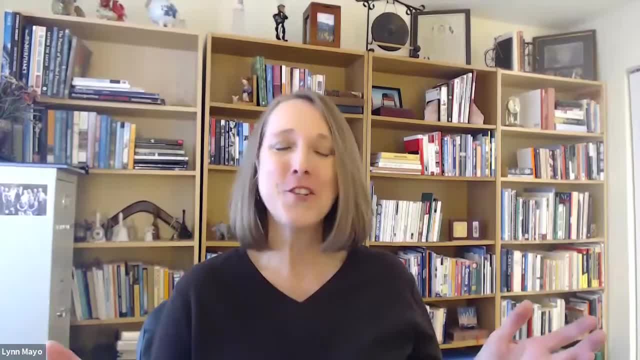 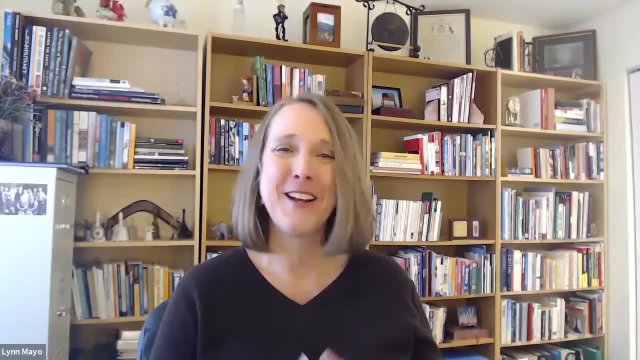 That's really interesting. So you can go from waiting 12 years to see your design to waiting days to see them starting to construct. So really there's people that kind of can go with the flow either way with those problem-solvings. Sounds like it'd be interesting for them. 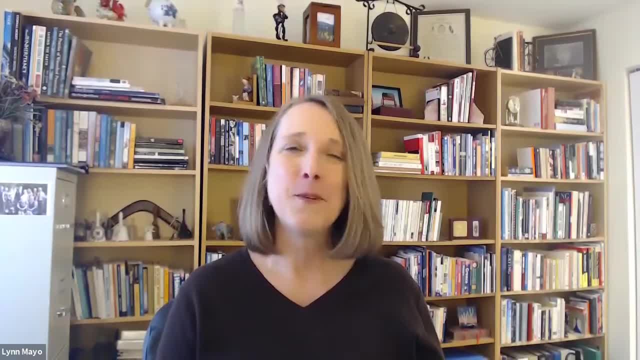 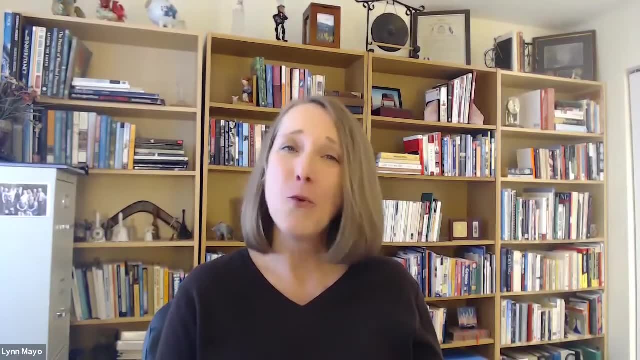 Well, thanks, Mike. That has been really interesting. I've learned a lot about transportation engineering. There's a lot of different aspects of it. It sounds like there's a lot of different things you can be doing in transportation engineering. I really appreciate your time. 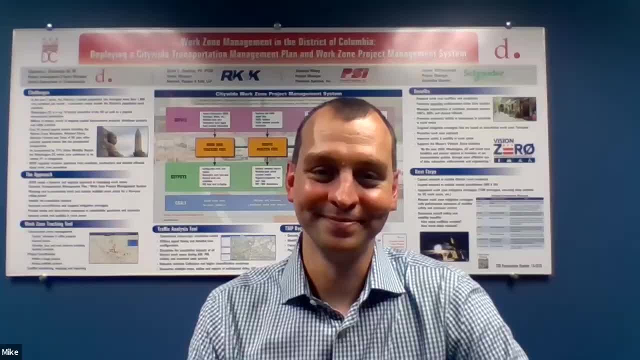 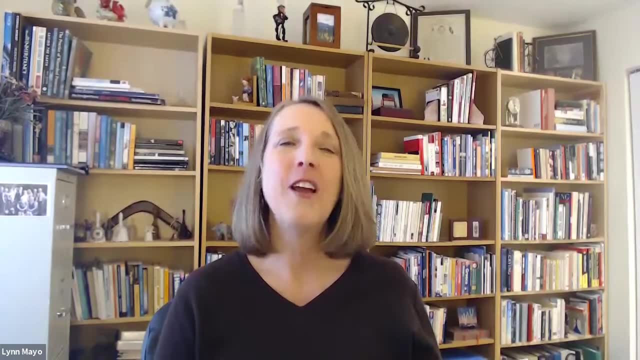 Thanks for having me, Lynn. This is really enjoyable for me too- Those people that are listening to us. if there's another engineering topic you'd like to have a webinar on, to find out more about that engineering career, just email us at info at repicturecom. Okay, thanks everyone. Thanks for having me.